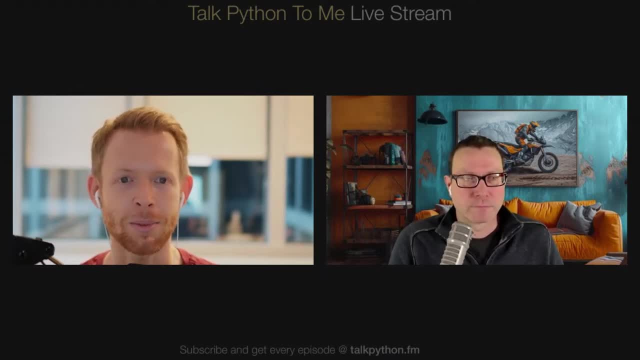 And then working with Python, And then working with the broader scientific Python, Python data science community to help enable Python to become a mainstream programming language for doing for doing data analysis and data science. And in the meantime, I've become an entrepreneur. I've I've, I've started some companies and have been working to you know, innovate and improve the computing infrastructure that powers data science tools and libraries like like pandas. 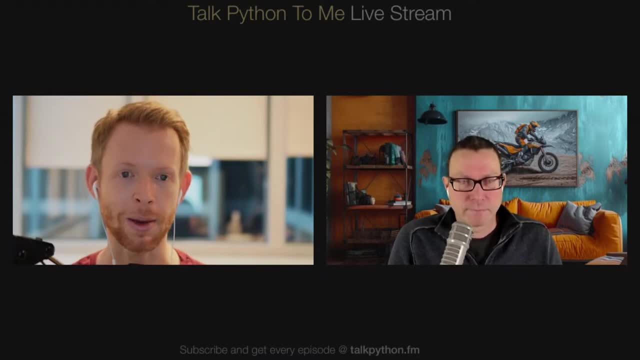 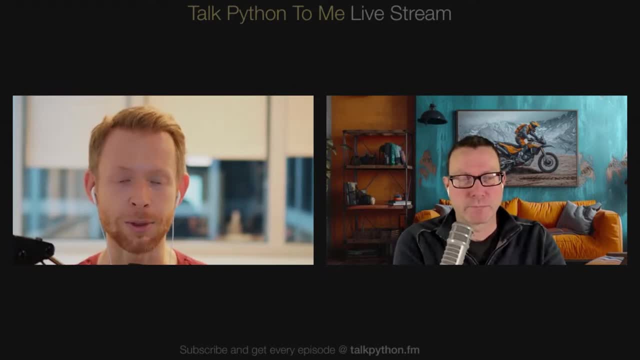 for doing Arrow development from 2018 to 2020.. They helped me incubate the startup that became Voltron Data, And so I've gone back to work full-time there as a software architect to help them with their Python strategy to make sort of their data science platform a delight to use. 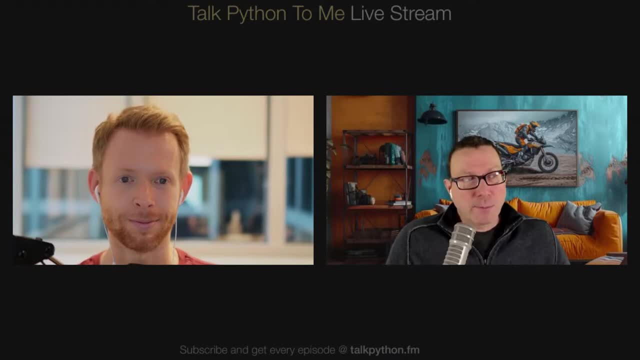 for the Python user base. I'm pretty impressed with what they're doing. I didn't realize the connection between Voltron and Posit, but I have had Joe Chung on the show before to talk about Shiny for Python And I've seen him demo a few really interesting things. 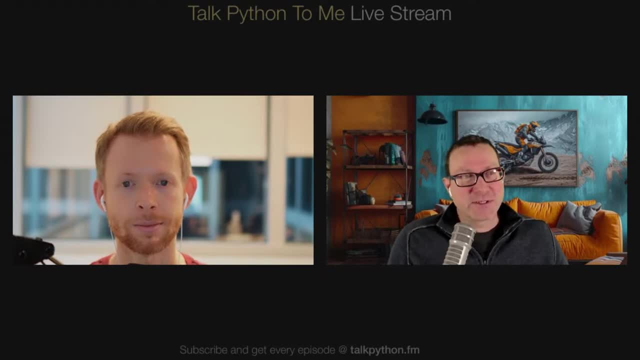 how it integrates into Notebooks these days. some of the stuff that y'all are doing, And yeah, it's just, it's fascinating. Maybe give people a quick elevator pitch on that. while we're on that subject, On Shiny or on Posit in general, 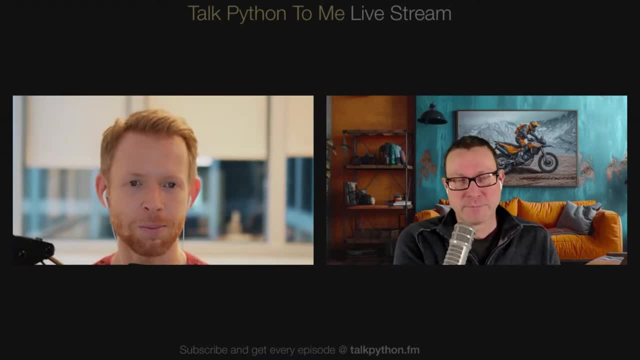 Yeah, whichever we feel like Yeah. so Posit started out 2009 as RStudio, And so it didn't start out intending to be a company. JJ Lair and Joe Chang built a new IDE: integrated development environment for R. 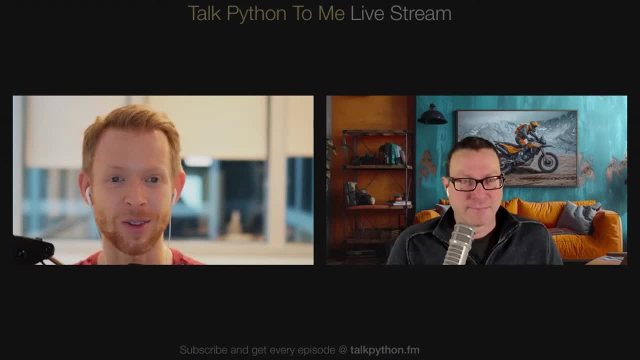 because what was available at the time wasn't great, And so they made that into, I think, probably one of the best data science IDEs that's ever been built. It's really an amazing piece of tech. So that started becoming a company with customers and revenue. 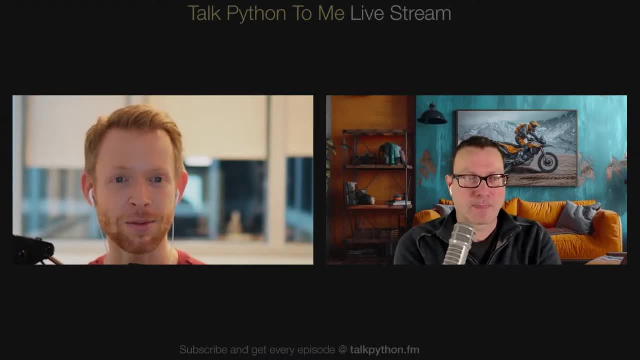 in the 2013 timeframe And they've built a whole suite of tools to support enterprise data science teams to make open source data science work in the real world. But the company itself- it's a certified B corporation- has no plans to go public or IPO. 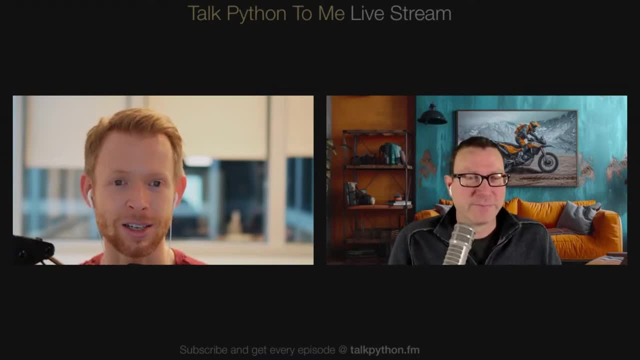 It is dedicated to the mission of open source software for data science and technical communication And basically building itself to be a hundred year company that has a revenue generating enterprise product side and an open source side, So that we, the open source, feeds the kind of enterprise. 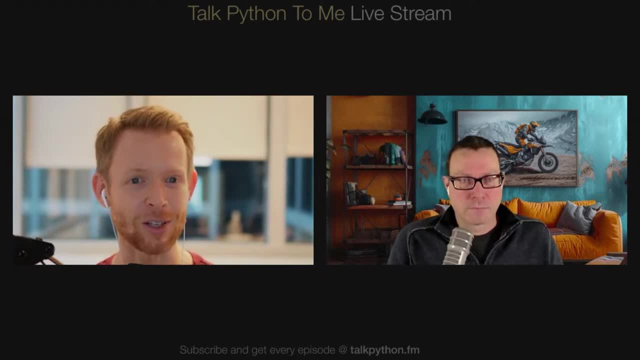 you know, enterprise part of the business. that enterprise part of the business generates revenue to support the open source development And the goal is to be able to sustainably- do sustainably support the mission of open source data science. you know, for you know, hopefully, the rest of our 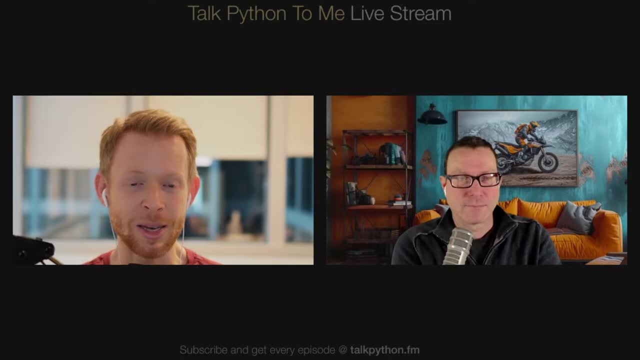 hopefully the rest of our lives, And it's an amazing company. It's been one of the most successful companies that dedicates a large fraction of its time to data science. It's been one of the most successful companies that dedicates a large fraction of its engineering time. 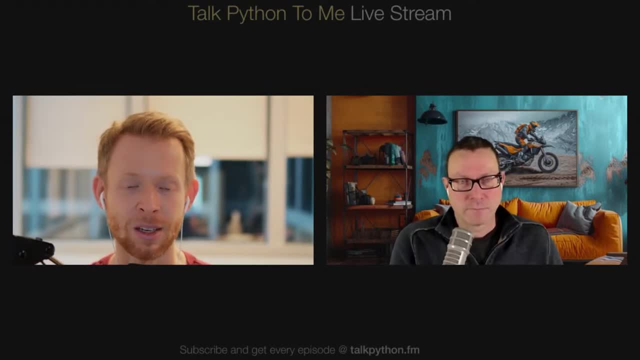 to open source software development. So it's- yeah, it's been in, yeah, very impressed with the company and you know JJ Allaire, its founder, And so you know I'm excited to be, you know. 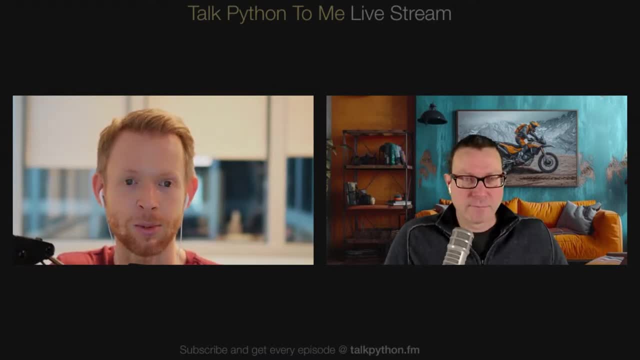 helping it, helping it grow and and become a sustainable long-term fixture in the, in the ecosystem. Yes, Yeah, It's definitely doing cool stuff, you know, as incentives are aligned well, right, It's not private equity, I think it. I think it helps. 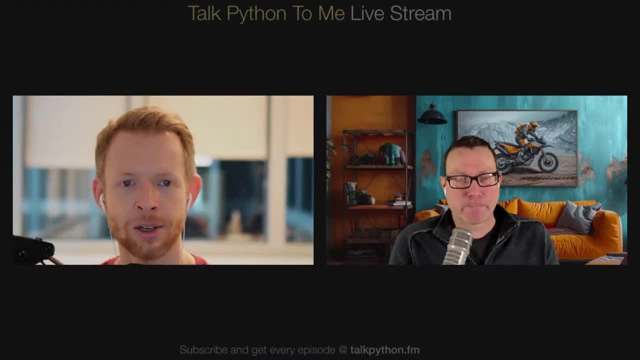 So so some people, many people know JJ Allaire created ColdFusion, which is like the original dynamic web development framework in the 1990s and that and so so he and his brother, he and his brother Jeremy. 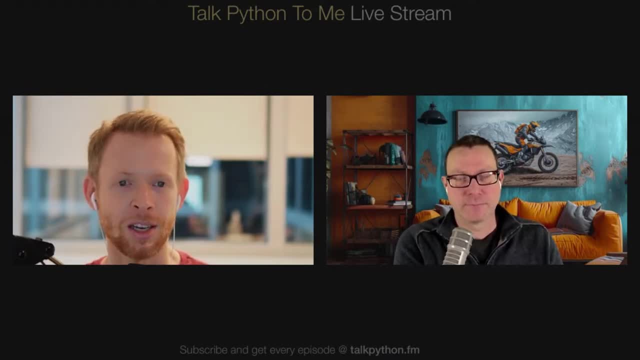 some others built Allaire Corp to commercialize ColdFusion and they built a successful software business that was acquired by Macromedia, which was eventually acquired by Adobe, but they did go public as Allaire Corp during the dot-com bubble, And JJ went on to found a couple of other successful startups. 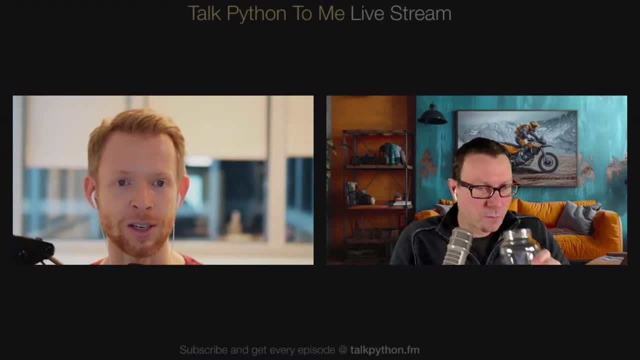 And so I think he found himself in his late thirties, in the, you know, 15 years ago or around around age 40, around the age I am now, you know, having been very successful as an entrepreneur, like no need to make, make money and looking for like a mission. 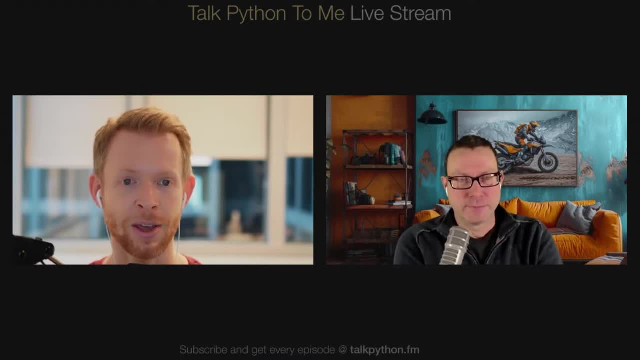 to spend the rest of his career on and that you know he just kind of, you know, have a better future. you know, identifying data science and statistical computing as, um, you know, kind of an open source, in particular, like making open source um for for data science work, um, you know, was the mission that. 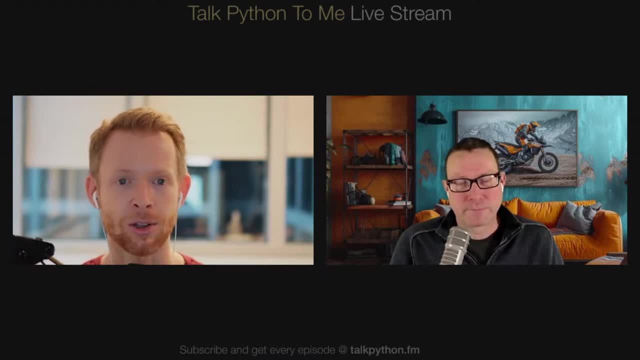 he- uh, he aligned with and something that he had he'd been interested in earlier in his career, but he had gotten busy with other things. so i think it's it's really refreshing to work with people who are really mission focused and focused on making impact in the world, creating great software. 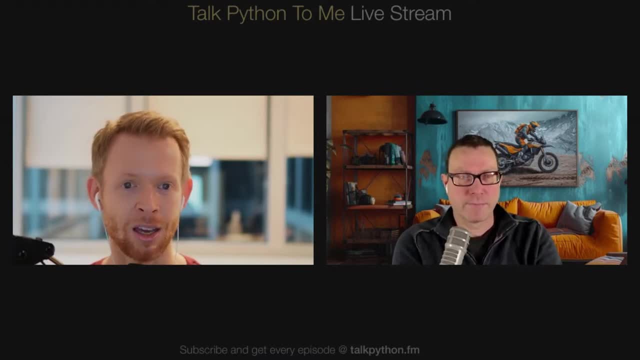 empowering people, increasing accessibility and and making you know, making most of it available for free on the internet, um, and not being so focused on, you know, empire building and um, and you know producing, you know, uh, you know great, you know great profits for you know, uh, venture. 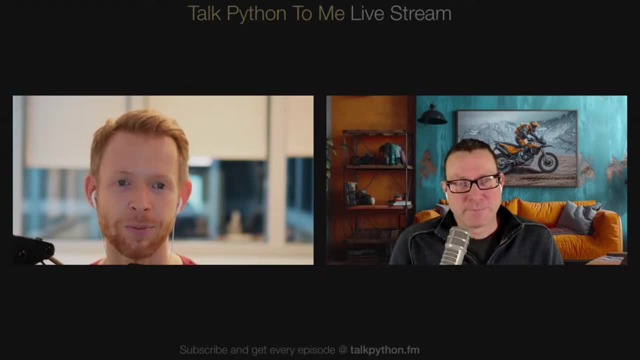 investors and things like that. so i think, um, yeah, i think the goal of the company and uh is to, you know, provide like a, um you know, an amazing home for um top tier software developers to work on this software, to, you know, spend their careers and to to build families and, uh, uh, to be a happy happy. 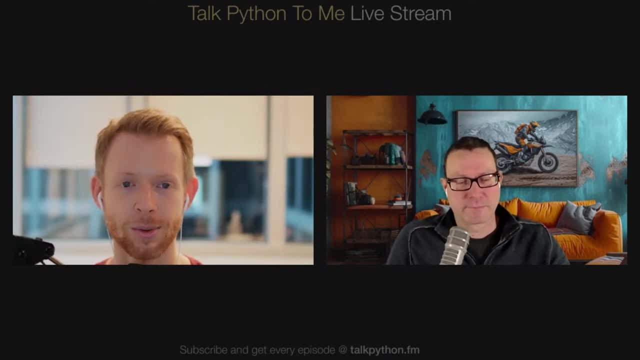 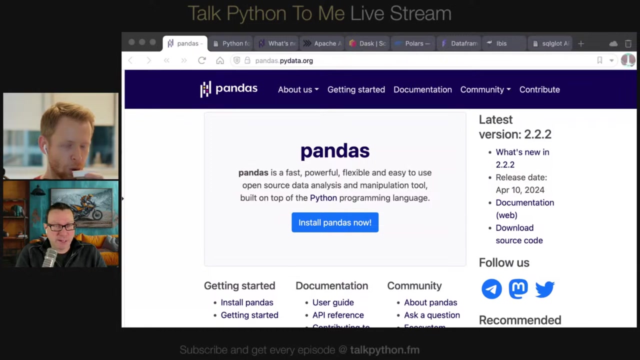 and healthy culture. uh, for for working on this type of software. that sounds excellent. wow, very cool. i didn't realize the history all the way back to cold fusion. speaking of history, let's uh jump in. there's a west. there's a possibility that people out there listening don't know what pandas. 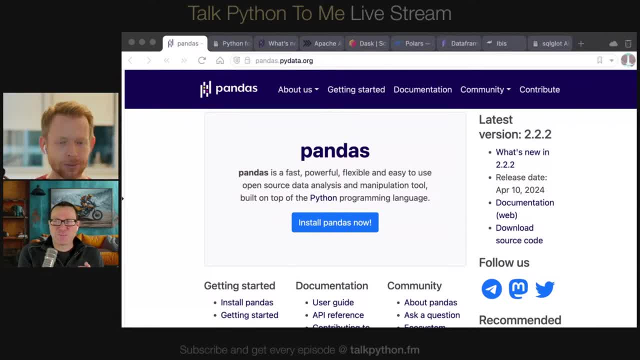 is it's? you would think it's pretty ubiquitous and i i certainly would say that it is especially in the data science space. but i've i got a bunch of listeners who listen and they say really surprising things. uh, they'll say stuff to me like michael. i've 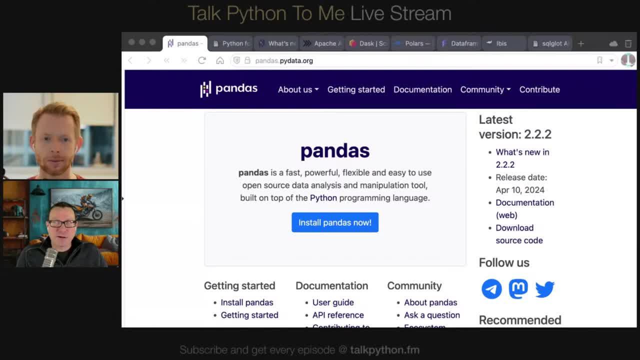 been listening for six weeks now and i'm starting to understand some of the stuff you all are talking about. like why did you list for six weeks? you didn't know what i was talking about. like that's crazy, it's, and a lot of people use it as like language immersion to get into the python. 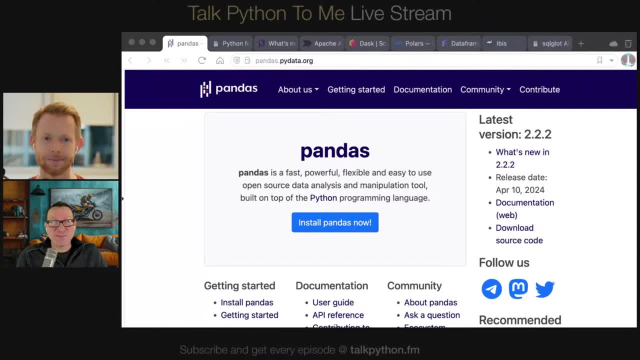 space. so i'm sure there's plenty of people out there who are, you know, immersing themselves, but are are pretty new, so i'm going to stop there. but i'm going to stop there because i think it's so. So maybe for that crew we could introduce what Pandas is then. 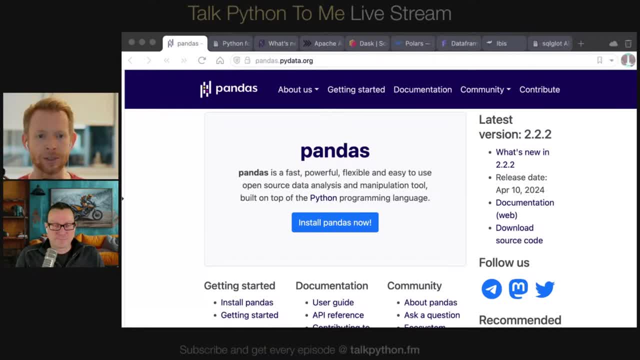 Absolutely Yeah. it's a data manipulation and analysis toolkit for Python, So it's a Python library that you install that enables you to read data files. So read many different types of data files off of disk or off of remote storage, or read data out of a database or some other remote data storage system. 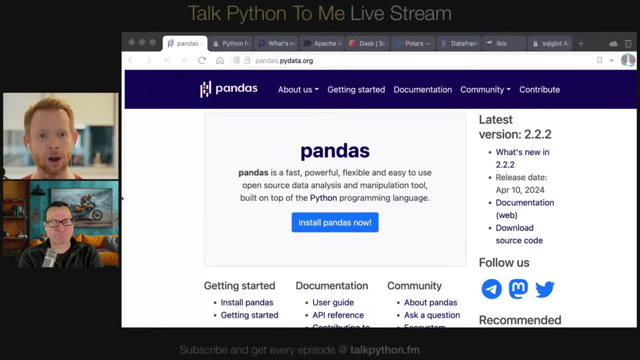 This is tabular data, So it's structured data like with columns. you can think of it like a spreadsheet or some other tabular data set And then it provides you with this data frame object, which is kind of pandasdataframe. that is the main tabular data object. 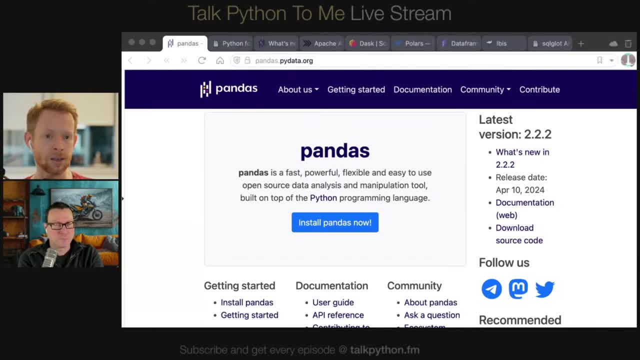 And it has a ton of methods for accessing, slicing, grabbing subsets of the data, applying functions on it that do filtering and subsetting and splicing, So you can do data selection as well as like more analytical operations, like things that you might do with a database system or SQL. 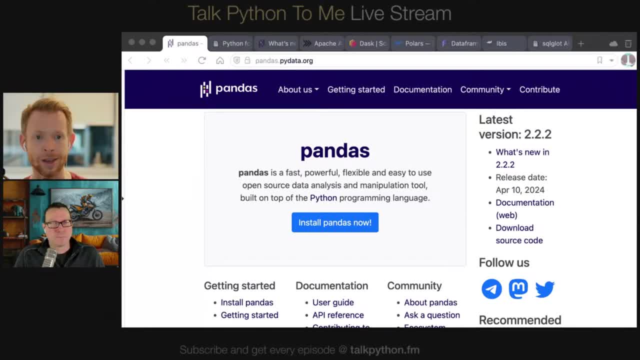 So joins and lookups, as well as analytical functions like summary statistics, grouping by some key and producing summary statistics. So it's basically a Swiss army knife for doing data manipulation, data cleaning and supporting the data analysis workflow, But it doesn't actually include very much as far as actual 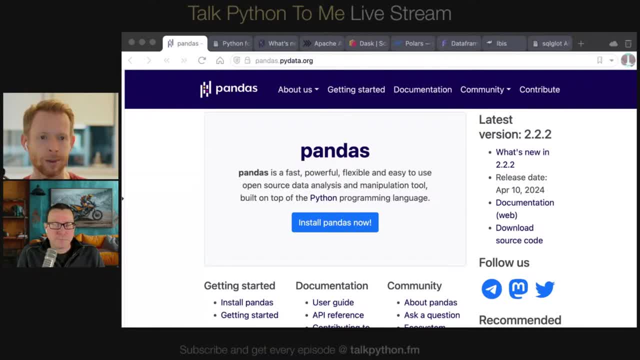 statistics or models, or you know, if you're doing, uh, something with llms or linear regression or some type of type of machine learning, you have to use another library. but pandas is the on-ramp for all of the data into um, into your environment in python. so when people are building some kind of 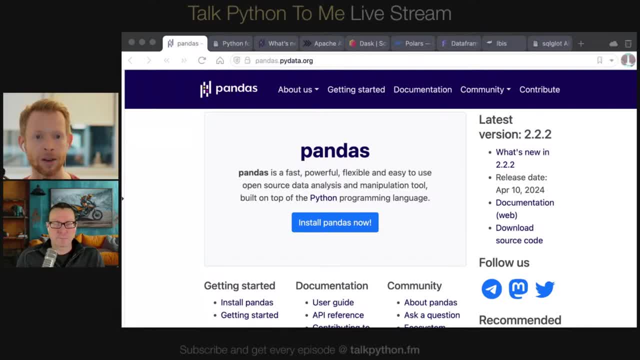 application that touches data in python pandas is often like the, the initial, like on-ramp for how data gets into python, where you clean up the data, you regularize, like regularize it, you get it ready for analysis and then you feed the clean- uh clean- data into the downstream. you know statistical 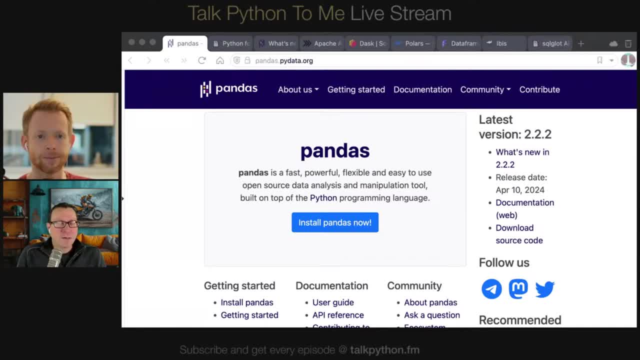 library or data analysis library, that you're using that whole data wrangling side of things, right, yeah, that's right, that's right, um, and so you know, it's some history like it. so. so python had um ray like matrices and what we call tensors, now multi-dimensional arrays. going back all the 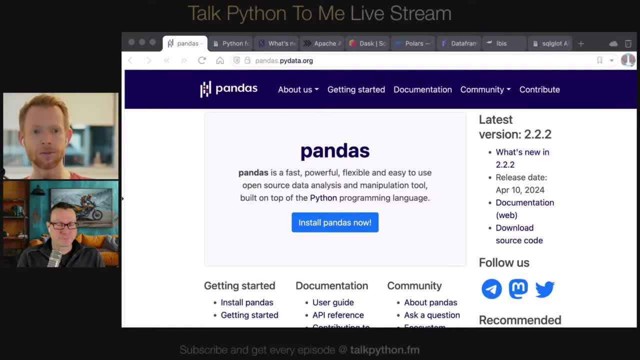 way to 1995, which is pretty, pretty early history for um, for python, like the python programming language, has only been around since like 1990 or 1991, if my memory serves. um. but the numpy- what became numpy in 2005, 2006, started out as numeric in 1995 and it provided numerical computing. 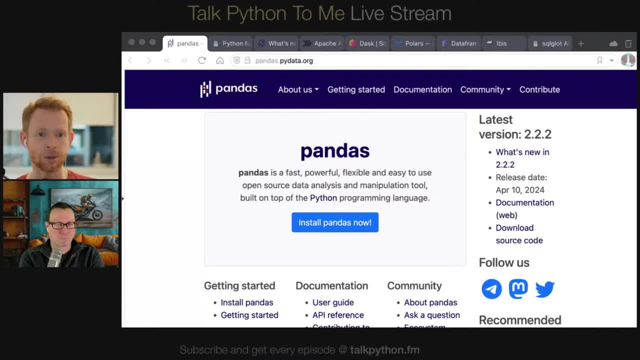 and it was mainly focused on, like multi-dimensional arrays, matrices, the kind of stuff that you might do, might do in matlab, but it was mainly focused on numerical computing and not with the type of business data sets that you find in database systems, which contain a lot of strings or 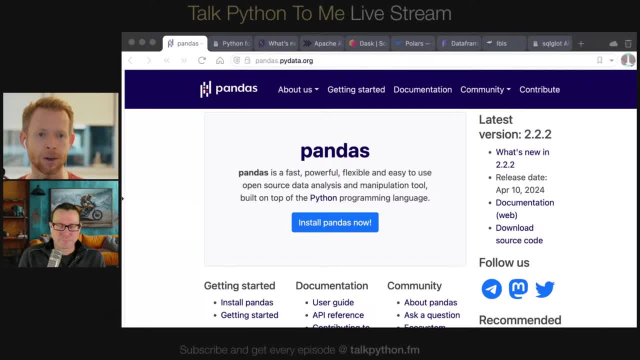 dates or non-numeric data, and so my initial interest was: i found python to be a really productive programming language. i really liked writing code in it, writing simple scripts like you know, doing random things, you know, for my, for my job, but- and you had this numerical computing library, numpy, which enabled you to work with. 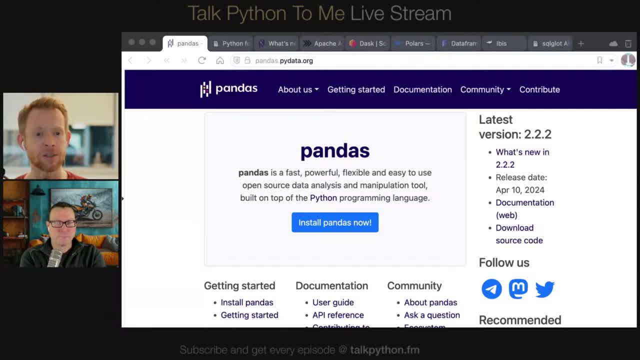 large numeric arrays and and large, you know, data sets with a single data type, um. but working with this more tabular type data, stuff that you would do in excel or stuff that you do in a database- it wasn't very easy to do that with with numpy, or it wasn't really designed for that, and so 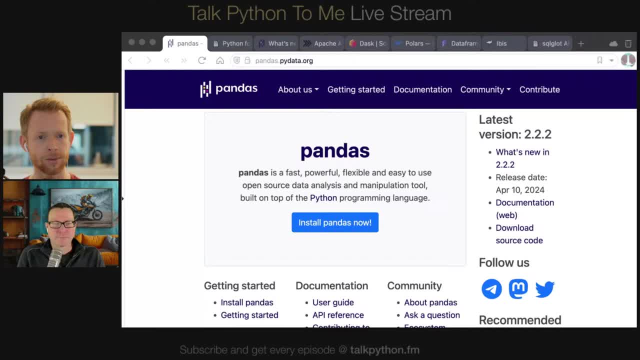 that's what led to building this like higher level library that deals with these tabular data sets, um, in the pandas library, which was originally focused on, you know, building really with a really close relationship with numpy. so pandas itself was like a thin layer on top of numpy originally. 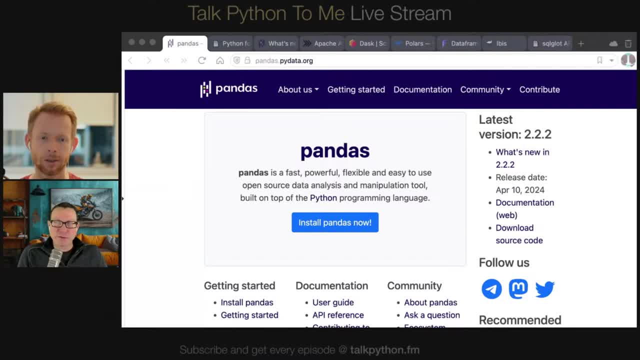 one thing i find interesting about pandas is it's almost its own programming environment these days, in the sense that you know traditional python, we do a lot of loops, we do a lot of attribute dereferencing, function calling and a lot of what happens in pandas is more more functional, it's more applied to us, it's almost like set operations right. 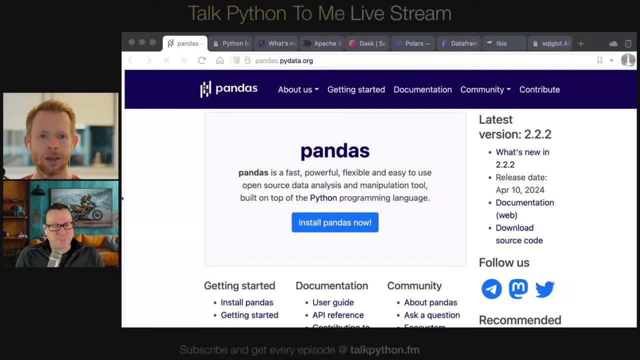 and a lot of vector operations and so on. yeah, it's so and that and that was inherited, that was behaviors inherited from, from numpy. so numpy is very array oriented, vector oriented. so you, rather than write a for loop, you would write a, an array expression which would operate on whole. 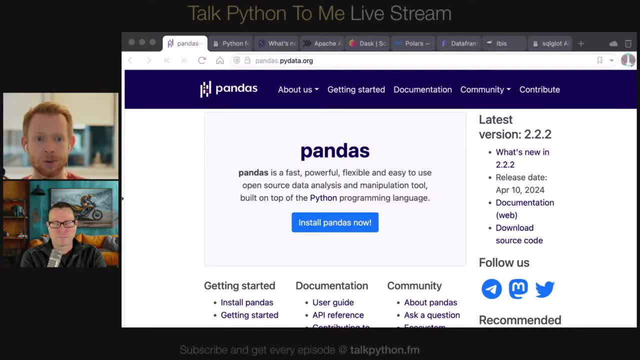 batches of data in a single function call, which is a lot faster because you can drop down into C code and get good performance that way. And so Pandas adopted the NumPy way of like the NumPy-like array expression or vector operations. 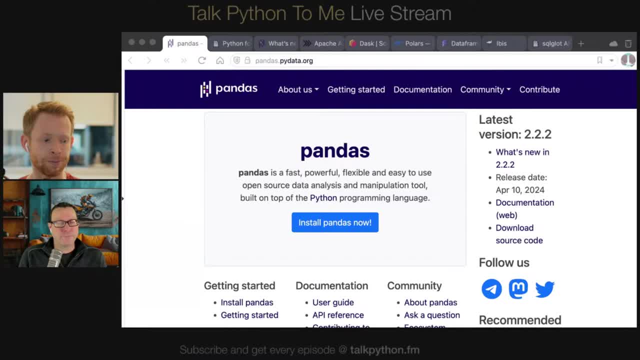 But it's true that that's extended to the types of like non-numeric data operations that you can do in Pandas, like you know, vectorized set lookups, where you can say like you would say like, oh, like this. I have this array of strings. 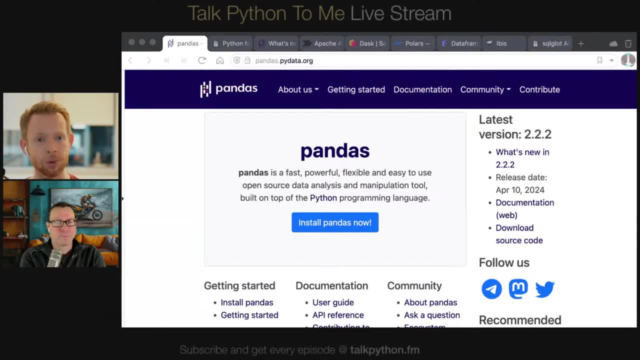 and I have this subset of strings and I want to compute a Boolean array which says whether or not each string is contained in this set of strings. And so in Pandas, that's, the is in function. So you would say, like you know, column A, 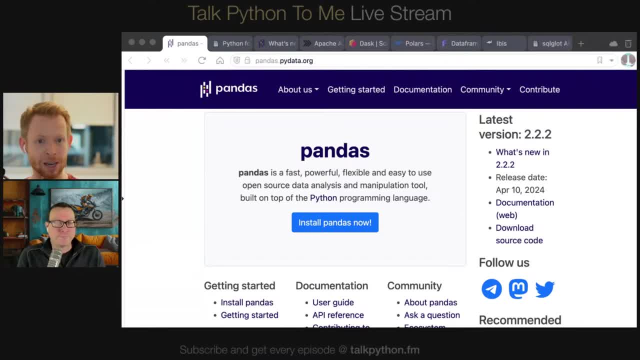 like is in some set of substrings and that produces that single function call, produces a whole Boolean array that you can use for subsetting later on. Yeah, That's kind of things that are really interesting in there, One of the challenges. maybe you could speak to this a little bit. 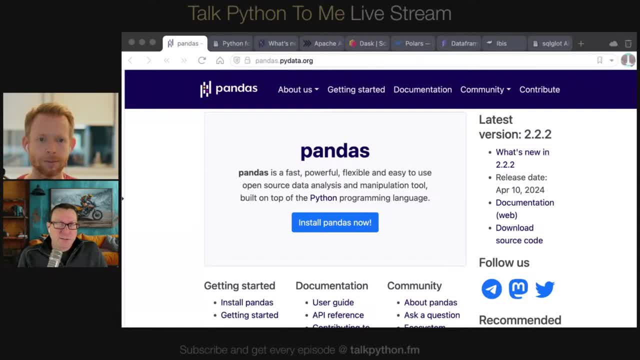 then I want to come back to your performance comment. One of the challenges, I think, is that some of it's, some of these operations, are not super obvious, that they exist or that they're discoverable right Like, instead of just indexing into, say, a column. 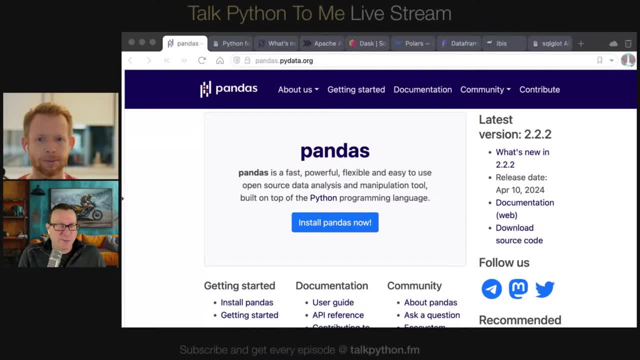 you can index on an expression that might filter out the columns or project them or things like that. How do you recommend people like kind of discover, you know? how do you recommend people like kind of discover, you know, discover a little bigger breadth of what they can do? 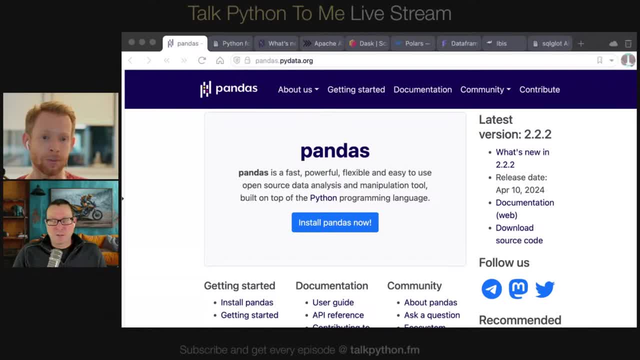 I mean there's plenty of. I mean I think there's great books written about Pandas. So there's my book Python for Data. I think Matt Harrison has written an excellent book: Effective Pandas- The Pandas documentation I think has provides really. 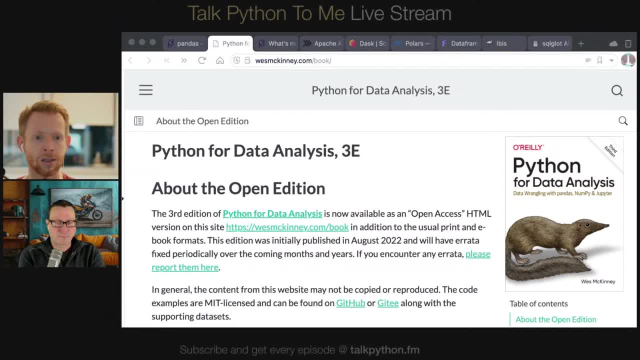 nitty gritty detail about how all the different things work. but you know when I was writing my, when I was writing. you know when I was writing my, when I was writing my book, you know, I think the most common thing was: 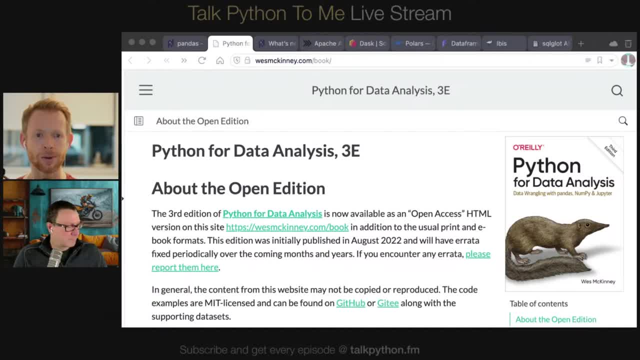 you know it was really hard to you know this, this book, python for data analysis. my goal was, to you know, provide a primer like a tutorial, and how to solve data problems with um, solve data problems with pandas, and so for that you know i. 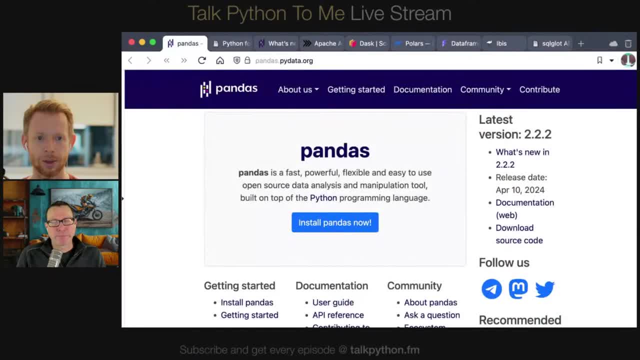 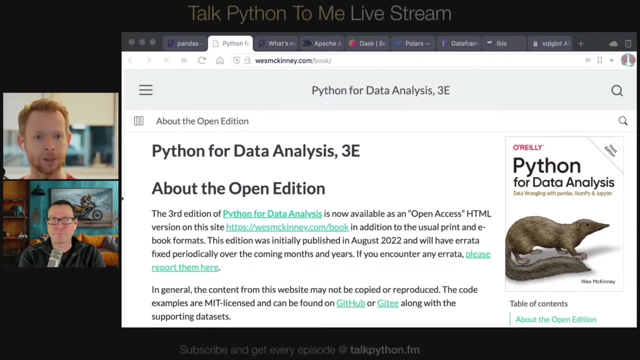 had to introduce how, some basics of how numpy works, so people array oriented computing, basics of python. so you know enough python to be able to understand, um, what things that pandas is doing. um, but the um yeah, kind of it builds incrementally and so like, as you go through the book, the 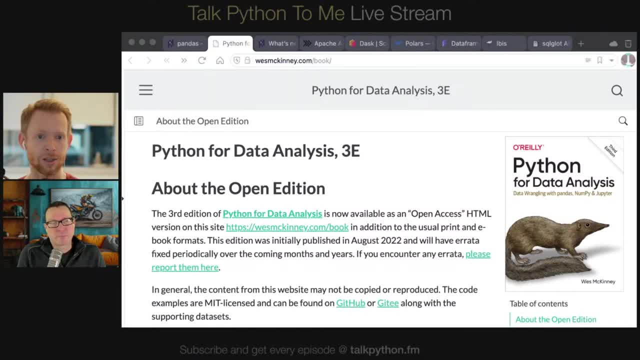 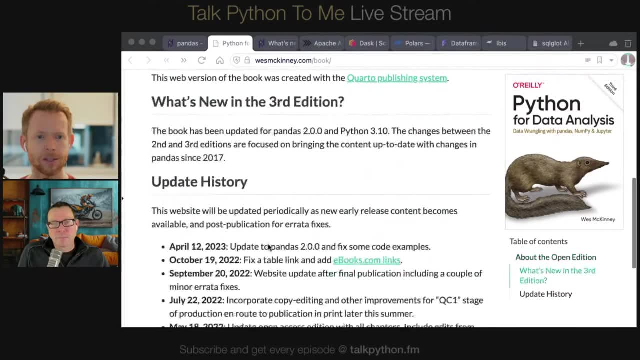 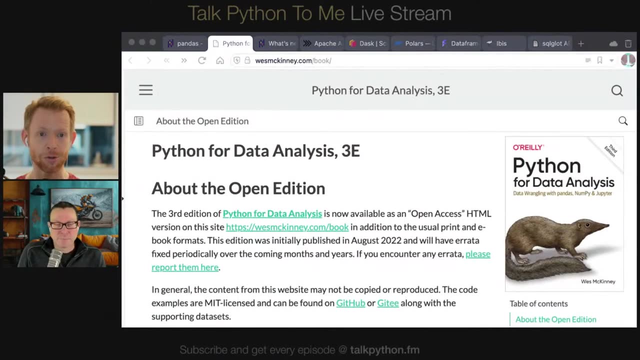 content gets um, you know, gets more and more advanced. it introduces, it built. you learn, you master initial set of techniques and then you can start learning about more advanced techniques. so it's definitely a pedagogical, you know, pedagogical resource and it is now freely as. 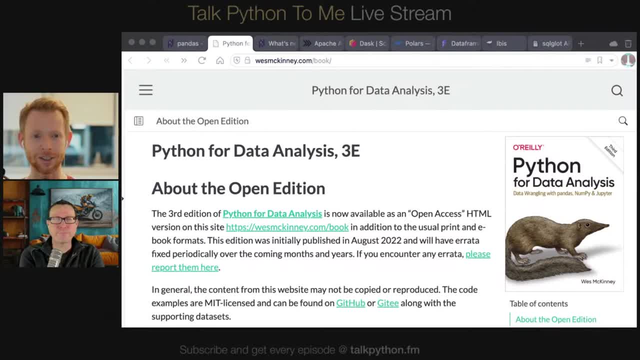 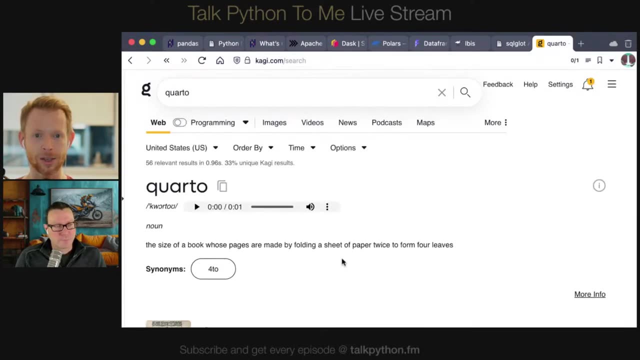 you as you're showing there on the screen. it is freely available um on the internet. so um jay helped me port the book to use quarto, which is a new um technical publishing system for writing books and blogs and and uh website. you know quartoorg um and um. there it is and uh yeah, so. 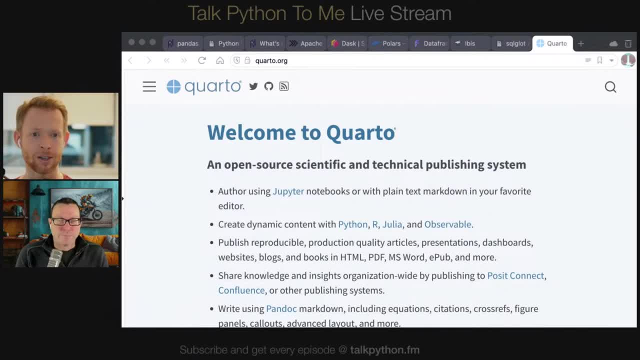 that's how i was able to publish, um my book uh on on the internet. as, uh, you know, essentially you can use quarto to write books using notebooks, which is cool. um, my, my book was written a long time ago and o'reilly is doc. xml, so not particularly fun to edit, but, um, yeah, but because, uh, quarter quarto is built on. 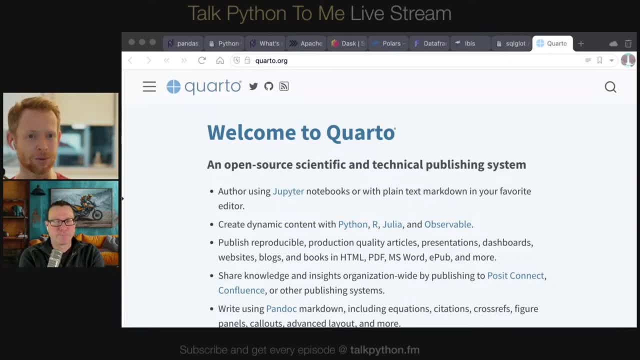 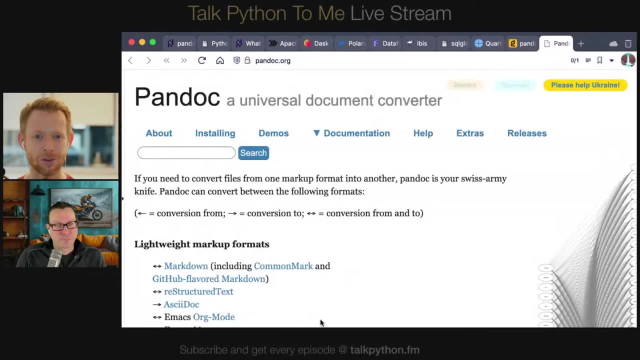 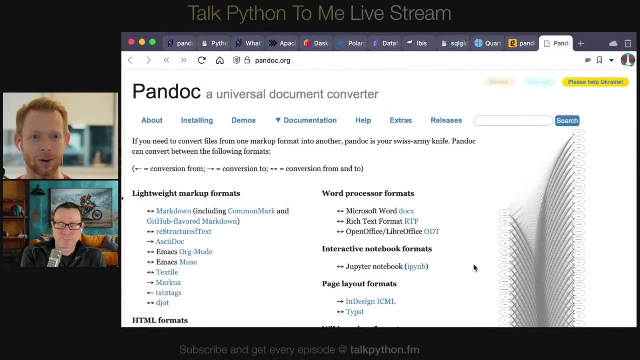 pandoc, which is a um, um sort of markup language transpilation system, so you can use pandoc to convert from one um, you know you can, to convert documents from one format to another, um, and so that's the, the for the kind of the root framework that quarto is built on, for, you know, generating 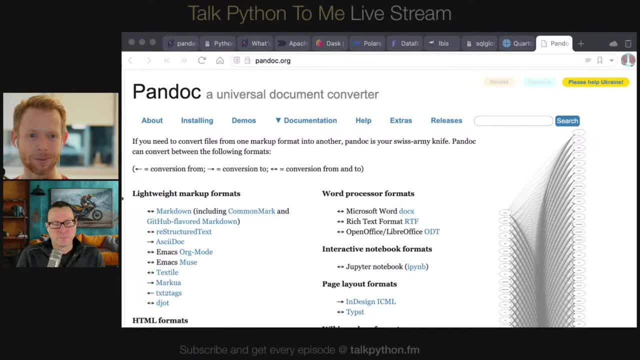 starting with one document format and generating many different types of output formats. that's cool. i didn't realize your book was available just to read on the internet. if, yeah, yeah, yeah, so in in the third edition um, i was able to to negotiate with um, with with o'reilly. 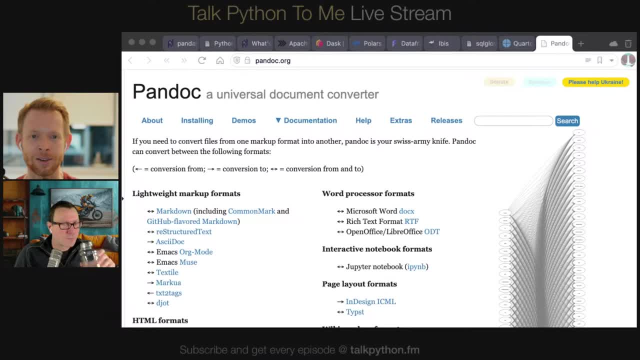 and add a. um. you know, add an, append and, uh, add a, make an amendment to my very old book contract from 2011 to let me release the release the book for free, um, on my website. so it's yeah, it's just available there at westmckinneycom and i'll see you in the next one. bye, bye. 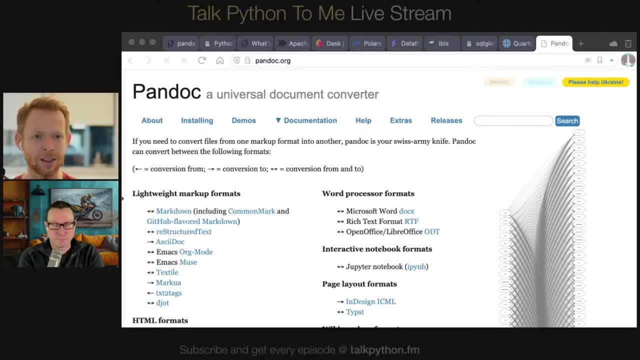 slash book. um, i find that, like a lot of people, really like the, the print book, and so, um, i think that having the online book just available, like whenever you are somewhere and you want to look something up is, is great, um, but uh, yeah, i've been hard to search. yeah, that's true, that's true, yeah. 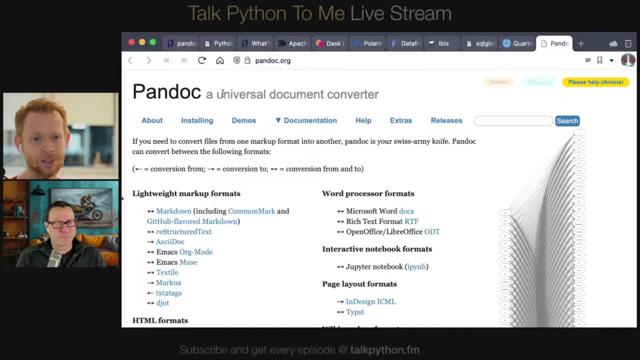 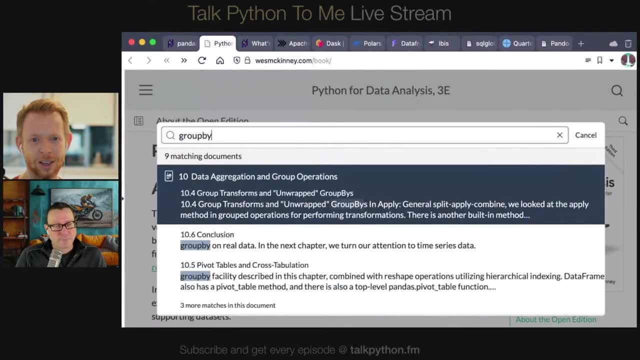 and like, if you go to the search bar and, um, if you go back to the book and just look at the search bar, um, you know, look at, just search for like group by like no, all one word, or you know, yeah, it's like it comes up really fast. you can. 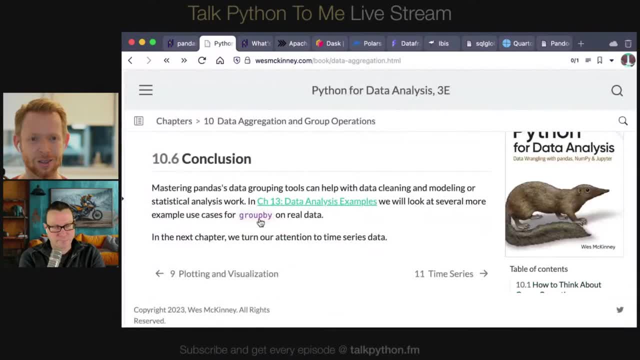 go to that section and it's- uh, it's, it's pretty cool. um, i thought that releasing the book for free online would would uh affect sales, but no people just really like having paper books, it seems. uh, even in 2024. yeah, even digital books are nice. you got them with you all the time you can, i think. 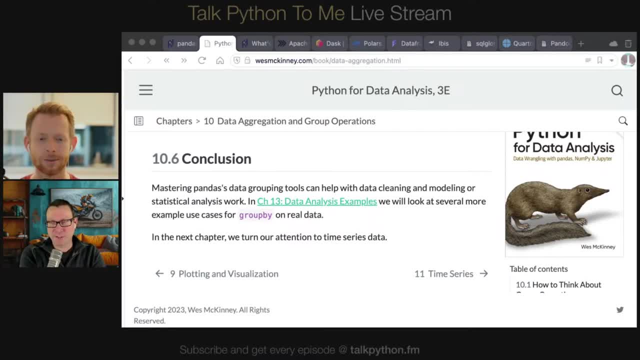 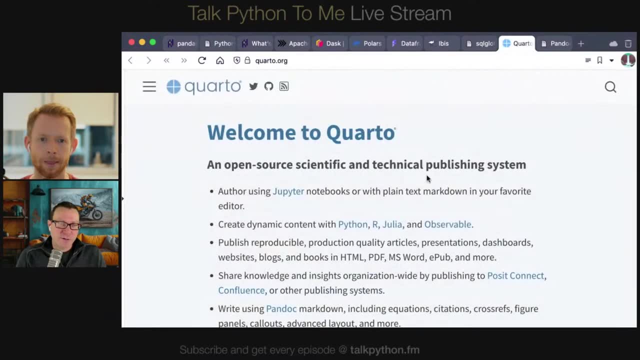 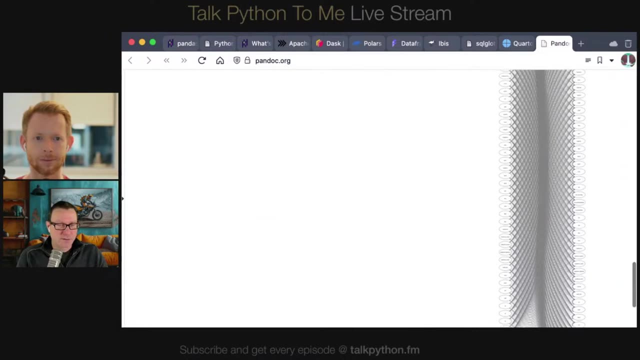 it's about taking the notes, where do i put my highlights and how do i remember it, and that's yeah, yeah, stuff like that. um, this quarter thing looks super interesting, uh, if you look at pandoc. if people haven't looked at this before, the conversion matrix. 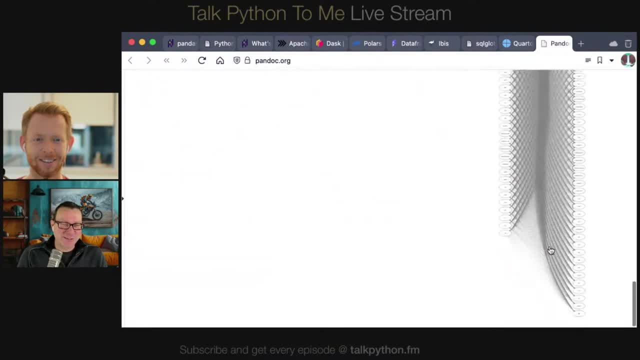 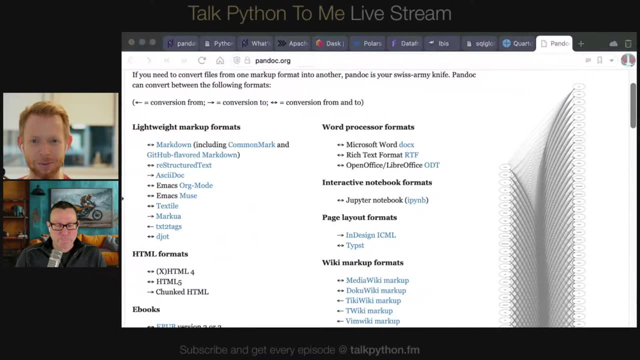 i don't know how you would. how would you describe this? wes busy and complete. what is this? this is crazy. it's very busy. yeah, it's it's. it can convert from looks like about you know 30 or 40 input formats formats to you know 50 or 60 output formats maybe, maybe more than that. it's kind of. 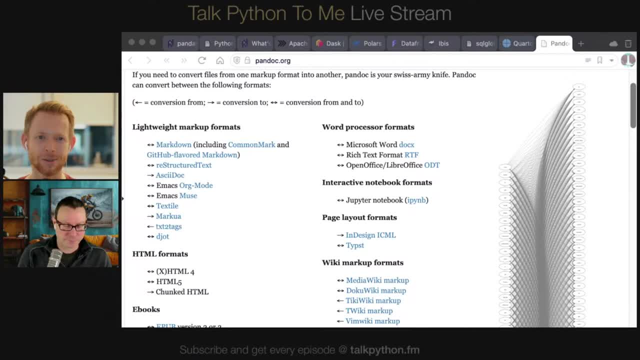 just eyeballing it. but yeah, it's like a pretty, pretty impressive. and then if you took the combinatorial of, like how many different ways could you combine the 30 to the 50? it's kind of what it looks like. it's right, it's truly amazing. so if you've got, 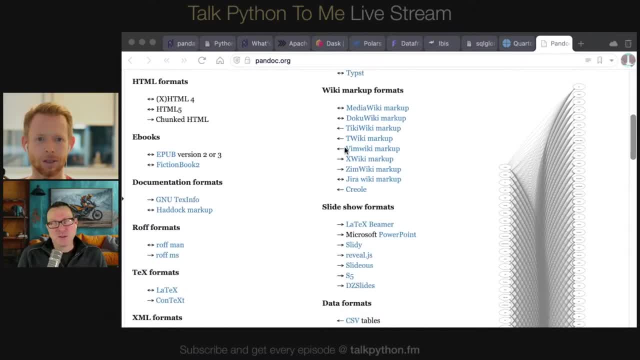 markdown, you want to turn it into a pdf, or you've got a, a doku wiki and you want to turn it into an epub or whatever right, or even like reveal js, probably to powerpoint, i would imagine, i don't know. yeah, yeah, well, as as history like backstory about, about quarto, so 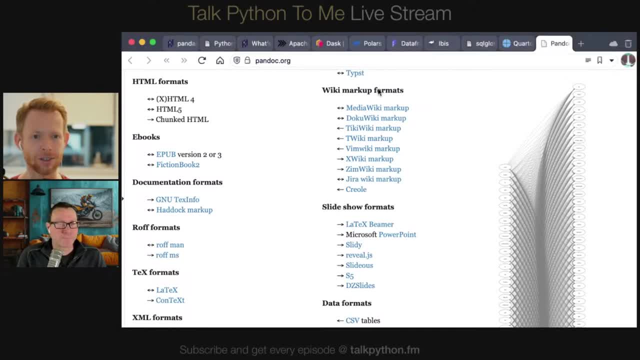 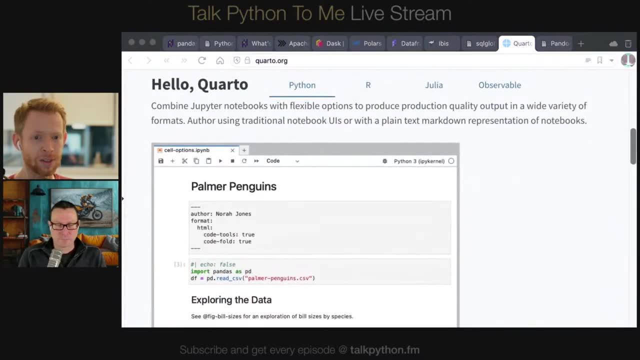 you know, it helps to keep in mind that that jj created cold fusion, which was this, uh, you know, essentially publishing system, early publishing system for um, for the internet, um similar to cgi, and and php and other dynamic, you know, web, web publishing systems, and so, at early on, at our 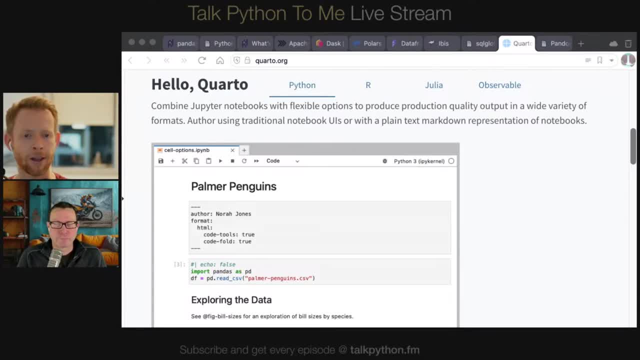 studio they created our markdown, which is a um, basically a extensions to markdown that allow you to have code cells written in in r, and then eventually they added support for some other languages where it's kind of like a jupiter notebook in the sense you could have some. 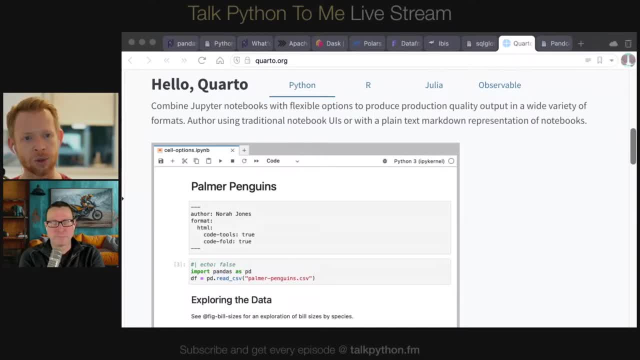 markdown and some code and some plots and output, and you would run the r markdown renderer and it would- it would, um, it would, you know, generate all the output and insert it into the, into the document, and so you could use that to write blogs and websites and everything but but our markdown. 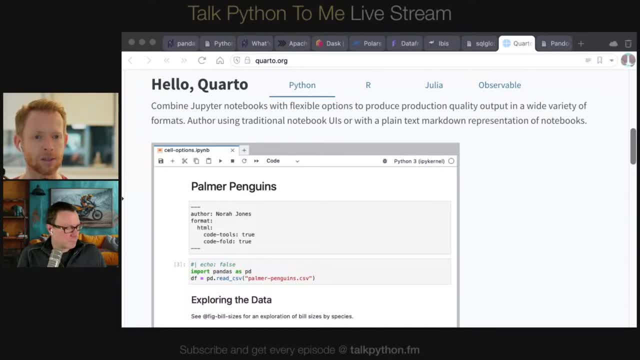 was written in r and so that that limited uh in a sense, like it made it harder to to install because it was in a way like a browser. uh, uh, you know you have to have to install r to use it. um, and also people, you know it, it in an association with r. that perhaps was like, like unmerited, and so in. 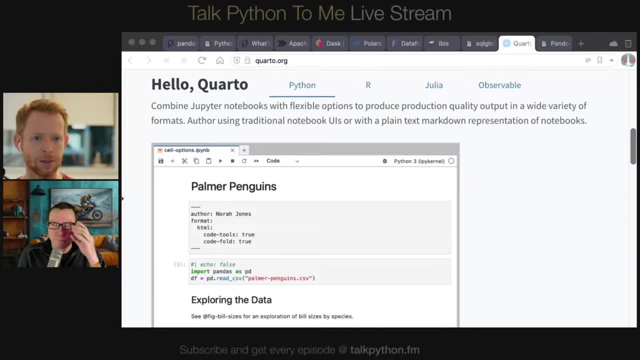 the meantime, um, you know, without everything that's happened with web technology- there's, it's- it's now very easy to put a complete uh javascript engine in a small install footprint, you know, on a machine with no dependencies, um, and to be able to run a system that is, uh, you know. 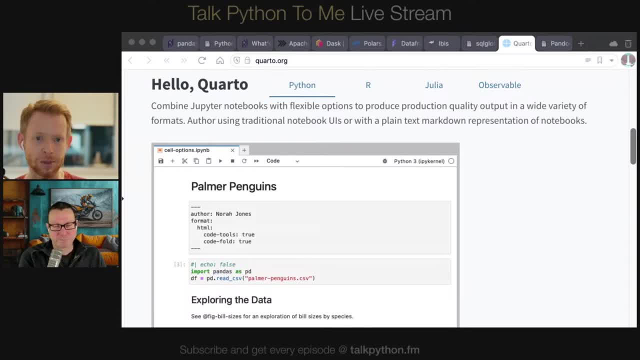 in a system that's written in JavaScript, And so Cordo is completely language agnostic. It's written in TypeScripts and it uses Pandoc as an underlying engine, and it's very easy to install, And so it addresses some of the portability. 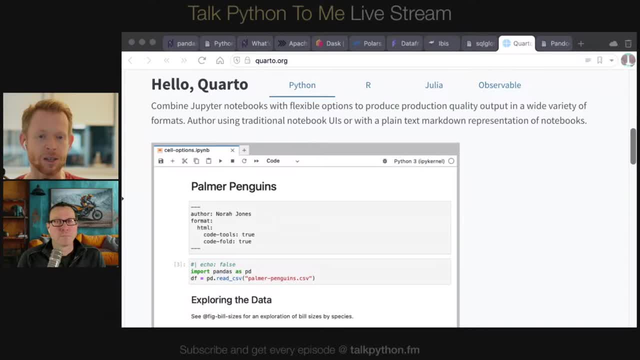 and extensive that were in R Markdown, But as a result I think the Posit team had a lot of just has more than a decade- or, if you include ColdFusion, more than 25 years of experience in building really developer-friendly. 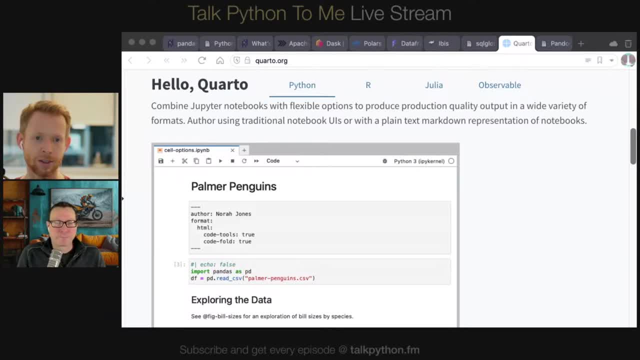 technical publishing tools, And so I think that it's not data science, but it's something that is an important part of the data science workflow, which is how do you make your analysis and your work available for consumption in different forms, And so having this system that can publish outputs. 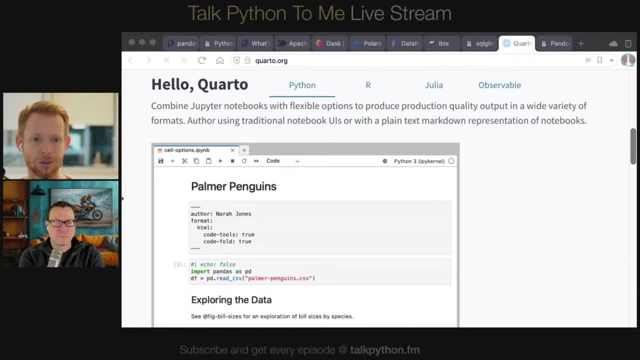 in many different places is super valuable. So a lot of people start out in Jupyter Notebooks, but there's many different possible input formats And so to be able to use the same source to publish to a website or to a Confluence page. 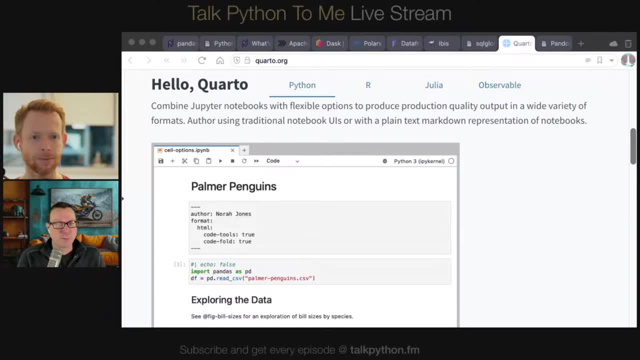 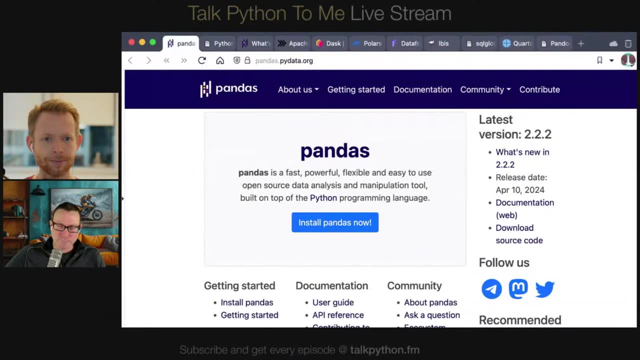 or to a PDF is like: yeah, it's super valuable, Yeah, it's super interesting. Okay, so then I got to explore some more. Let's go back to Pandas for a minute First, how about some kind words from the audience for you? 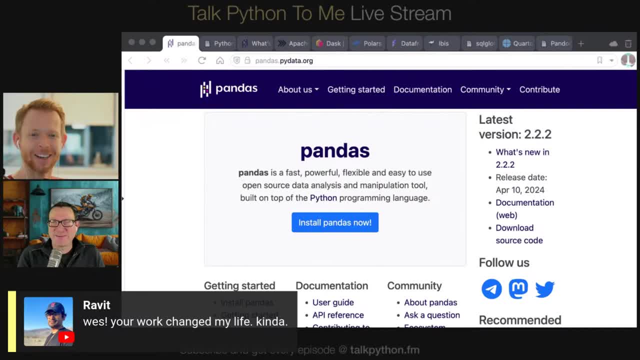 Ravit says: West, your work has changed. It's changed my life. It's very, very nice. I'm happy to hear it. But yeah, I'm more than happy to talk in depth about Pandas And I think the history of the project is interesting. 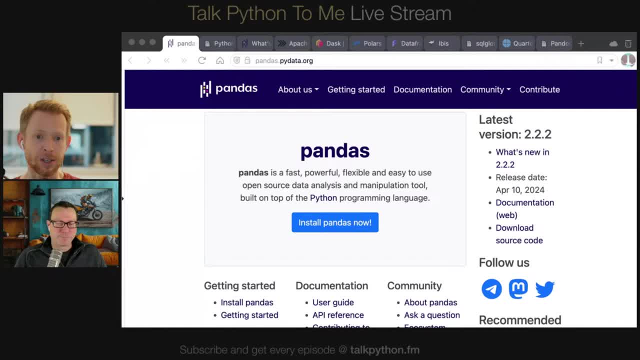 And I think also how the project has developed in the intervening 15, 16 years is pretty interesting as well. Yeah, let's talk derivatives for a minute, But I think I'm going to start with you, Ravit. I'm sure you've talked a lot about the world. 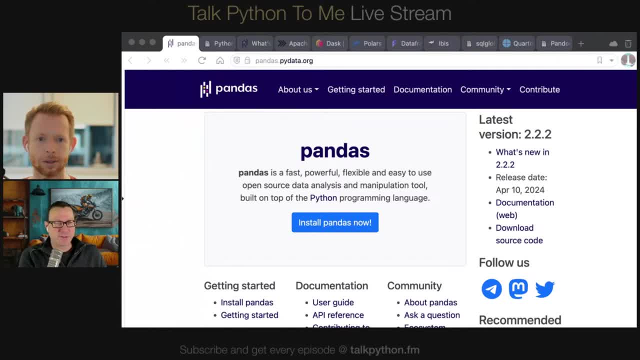 and the environmental impact on it. But what do you think of the world and the growth and speed of adoption and all those things? When you first started working on this and you first put it out, did you foresee a world where this was so popular? 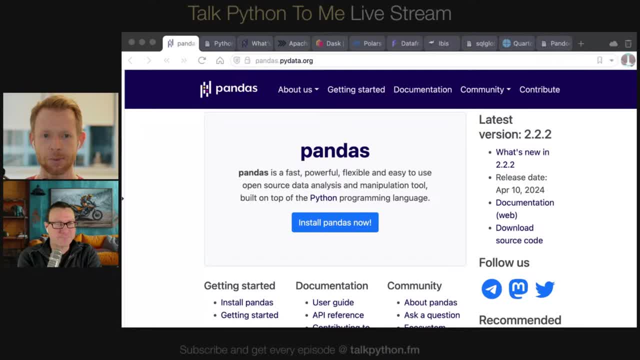 and so important. Did you think of- yeah, pretty soon- black holes. I'm pretty sure I'll be part of that somehow. Ravit Shahi, Founder & CEO Pandascom, of making um, making python, this mainstream um, mainstream language for statistical computing. 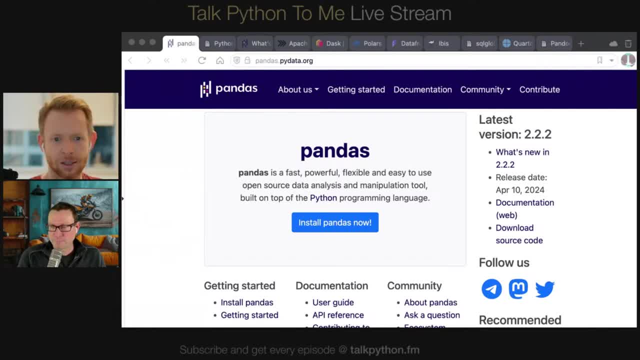 and and data analysis. like i didn't- uh, i, i, it didn't occur to me that it would become this popular, um, or that it would become like the one of the main tools that people use for working with data in a business, in a business setting like that, you know it would have been. 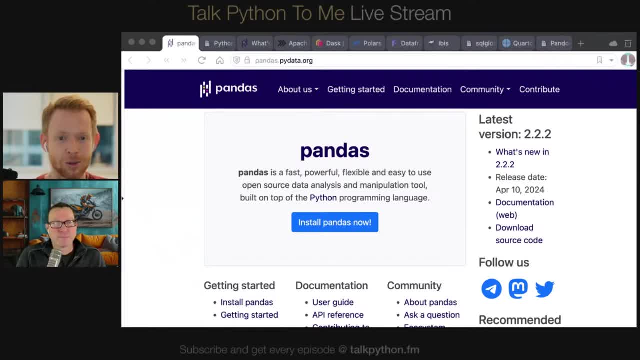 like if that was the, if that was the aspiration, or if that was you know what i needed to achieve, to be satisfied, um, that that would have been completely unreasonable. and i also don't think that that you know in, in a certain sense, like i don't- i don't know that- that it's popularity. 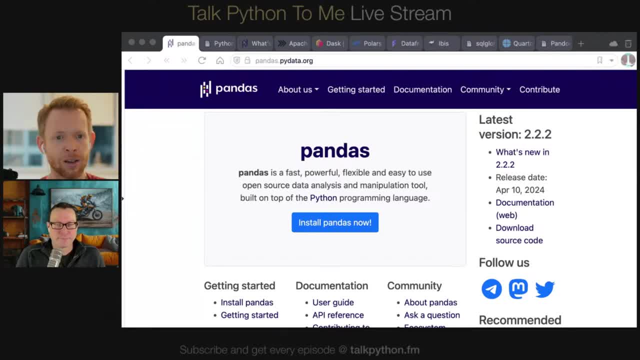 you know it, it is deserved and it's served like i. i think there's there's many other worthy efforts that have been created over the years that have been um the you know really, you know really great work that that others have have done in this, this domain. 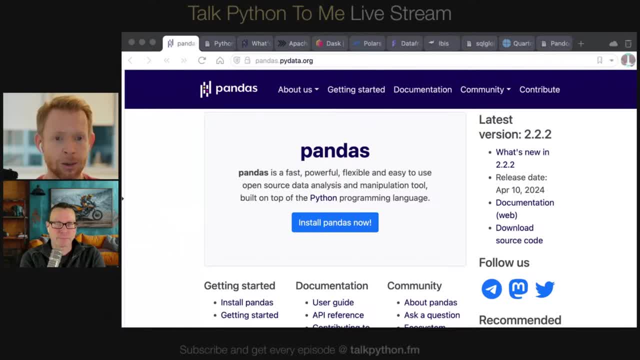 and so the fact that that pandas caught on and became as popular as it is. um, i think it's a combination of timing and, you know, there was like a developer relations aspect that there was content available and like i wrote my book and that made it easier for people to learn how to use the. 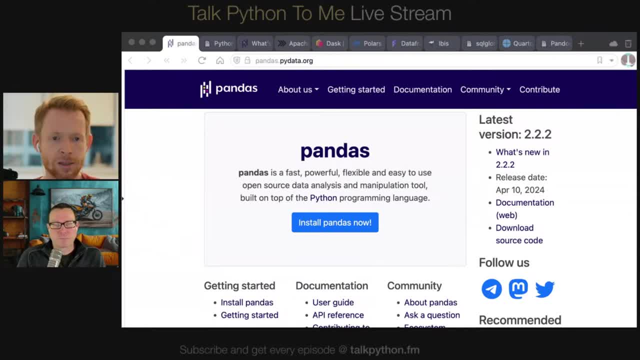 project um, but also, like we, we had a serendipitous um open source developer community that came together um that the project, to you know, grow and expand like really rapidly and the in the early 2010s and um, you know, and i, i, yeah, i definitely spent a lot of work like 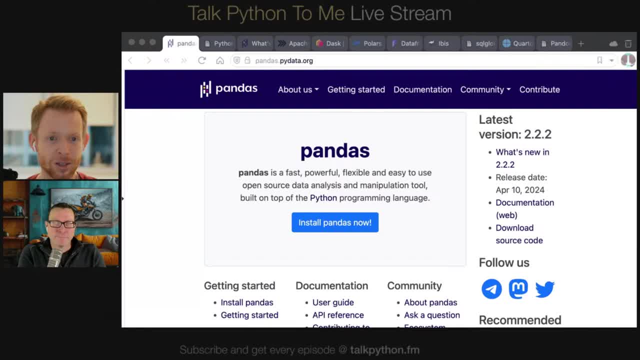 recruiting people to to work on the project and, uh, encouraging, you know, others to work on it, because sometimes people create open source projects and then it's hard, for hard for others to get involved and get a seat at the table, so to speak. um, but i was very keen to bring on others and to um give. 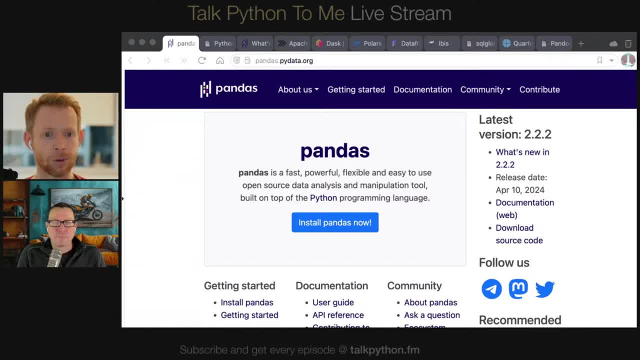 them a responsibility and you know, ultimately, you know hand over the reins to the, to the project, to. you know, uh, return the financial return to the project, um, and it was a great way to kind of spread that and and um, i've spoken a lot about that. you know over the years how important that. 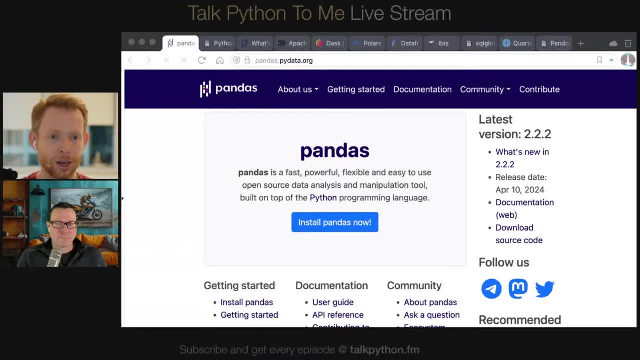 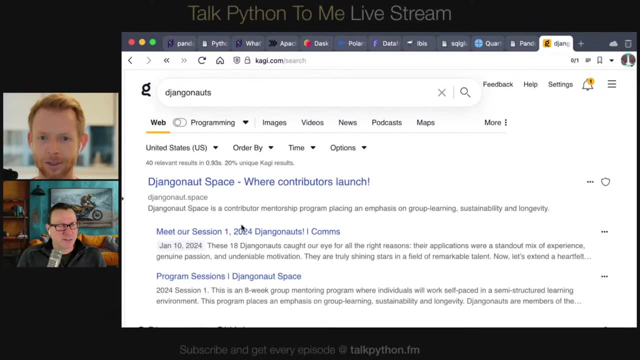 is to, you know, for open source project creators to room for others, um in um and growing the project so that they can become, you know, owner owners of it as well. it's tough to make space and tough to to bring on folks. have you heard of the jingo knots? 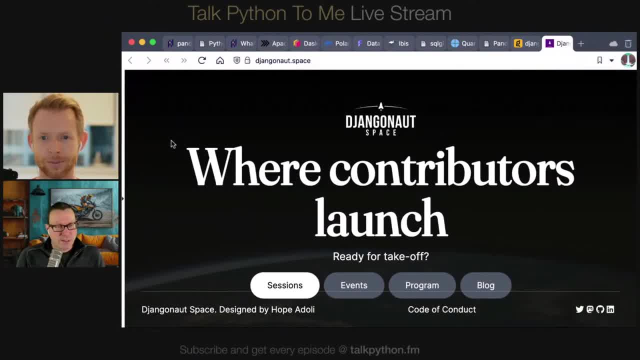 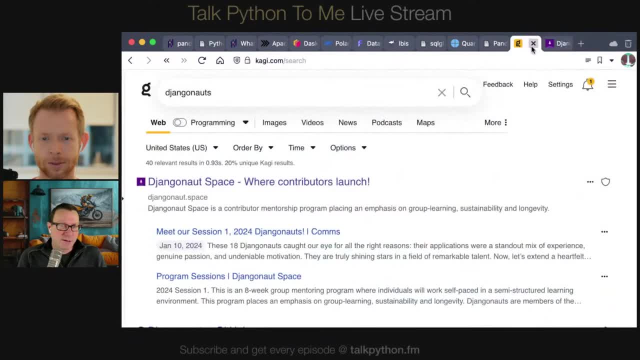 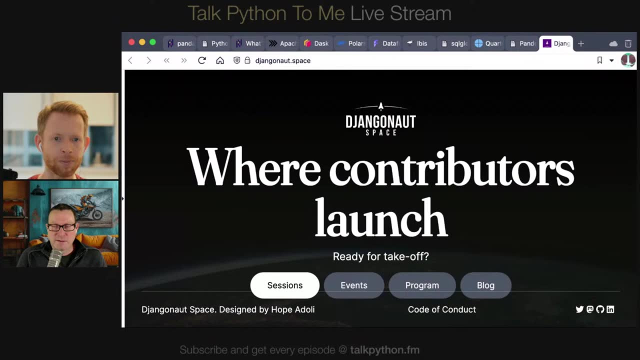 uh, basically like kind of like a boot camp, but it's for taking people who just like dingo and turn them into actually contributors or core contributors. do you guys have what's your onboarding story for people who do want to participate? um, I, I'm embarrassed to say that. 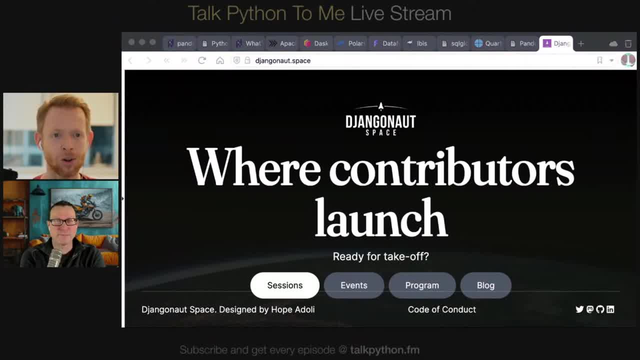 I'm not, uh, I'm not. I don't have a comprehensive view of, like all of the the different, you know, community outreach channels that the pandas project has done to help uh grow new contributors. um. so one of the core team members, Mark Garcia, has done like an amazing job working at organizing 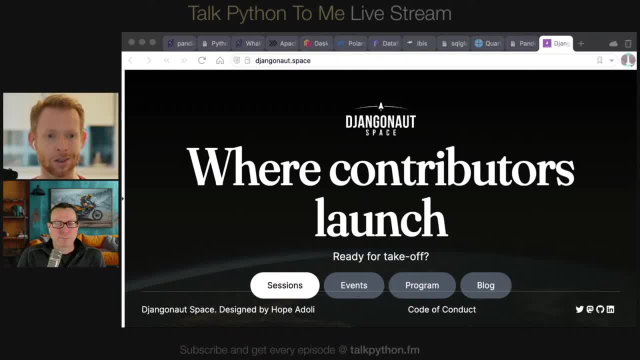 um documentation, Sprints and other like. contributor um sourcing events: essentially creating very, very friendly, accessible events where people who are interested in getting involved in pandas can meet each other and then assist each other in making their first pull request, and it could be something as simple as 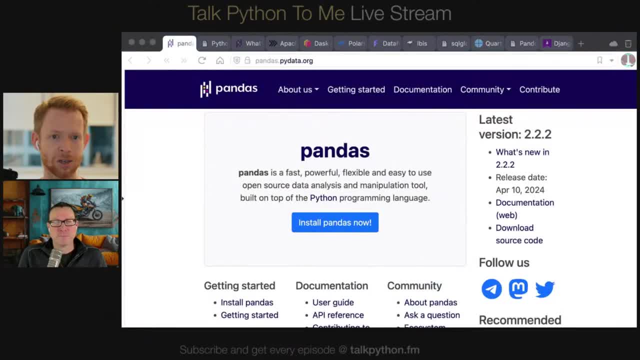 you know, making a small improvement to the, to the pandas documentation, because it's such a large project, the, the documentation, is, like always something that could be um, that could be made better. you know, either adding more, adding more examples, or documenting things that aren't documented um, or making- yeah, just just making the documentation better, and so it's something that 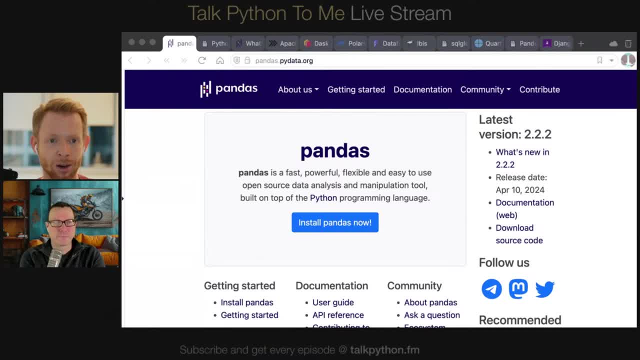 for new contributors is is more accessible than working on the internals of, like one of the you know algorithms or something and and uh, or like we're working on some significant performance improvement might be a bit intimidating if you've never worked on the pandas code base- and it's a pretty large code base, because it's been, it's been worked on continuously. 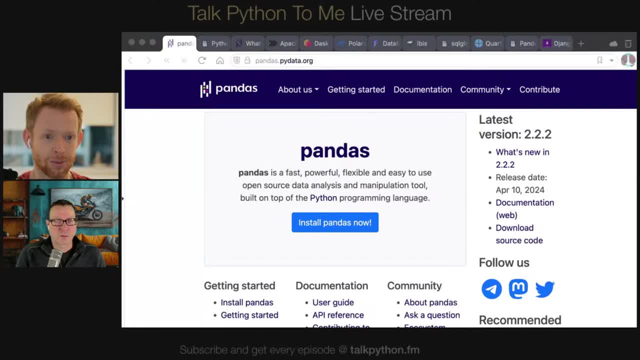 for, you know, for like going on 20 years. so, um, it's uh, yeah, it can be- takes a while to really get to a place where you can be productive, and that can be discouraging for new contributors, especially those who don't have a lot of open source experience. 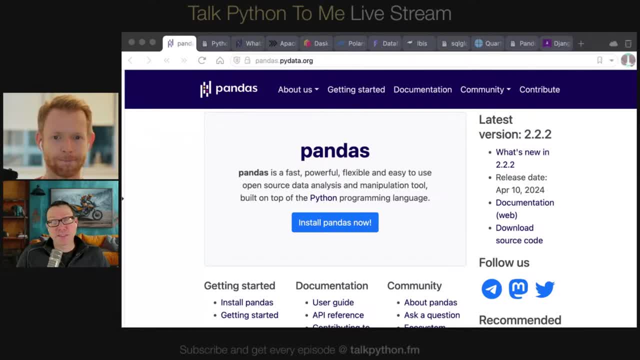 that's one of the ironies of challenges of these big projects is they're just so finely polished so many people are using them. every edge case matters to somebody right, and so to become a contributor and make changes to that it takes a while, I'm sure. yeah, yeah, I mean, I think it's, it's, um, definitely a. 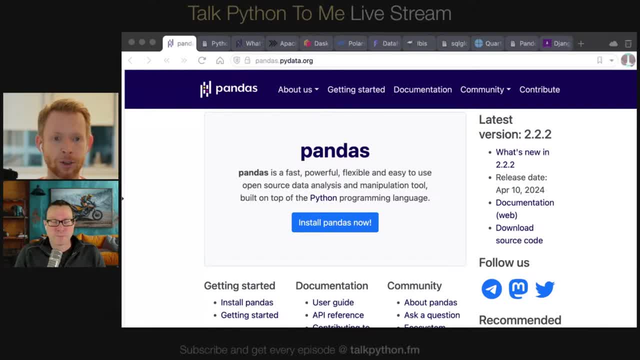 big. I think definitely a big thing that helped is allowing people to get paid to work on pandas or um, to be able to contribute to pandas as, as a part of their job description- like, as you know, maybe part of their job is maintaining maintaining pandas. so anaconda, um, you know, was, like you know, one of the earliest. 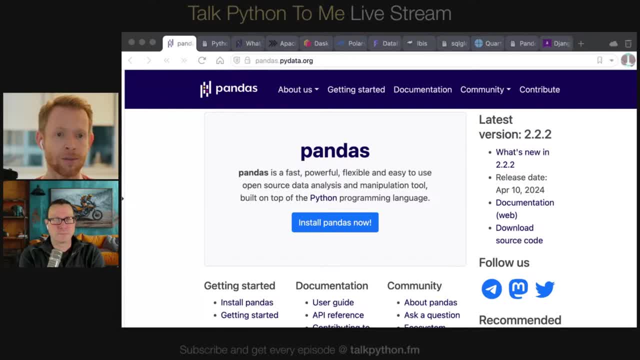 companies who had uh Engineers on staff. um, you know, like, uh, yeah, like you know Brock Mendel, you know Tom Augsburger, Jeff Reback, who part of their job was maintaining and developing, developing pandas, and that was that was huge, because prior to that, the project was purely based. 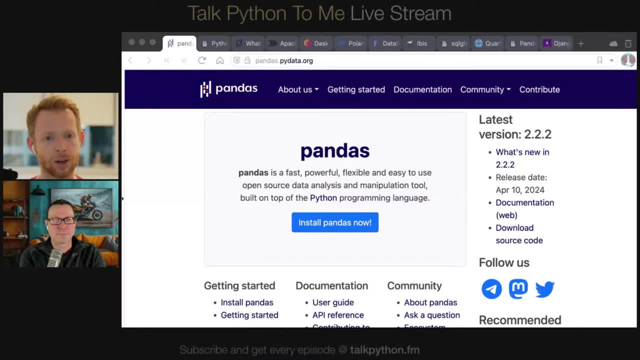 on volunteers like I. I was a volunteer and you know everyone was working on the project as a, as a passion project in their, in their free time. um and then um. you know Travis oliphant. you know one of the founders. he and Peter Wang founded anaconda um. Travis spun out from anaconda to create Quonsight. 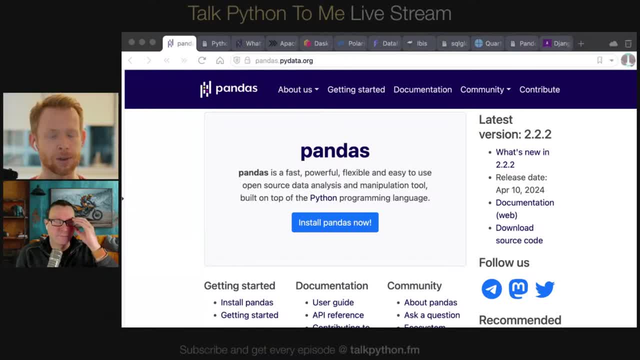 and has continued to. um, you know, sponsor, uh, sponsor development, um in and around, in and around pandas, and that's enabled people like Mark to do these- um community building, uh events and um, and for it to not be, you know something that's uh, you know totally, uh, totally uncompensated. 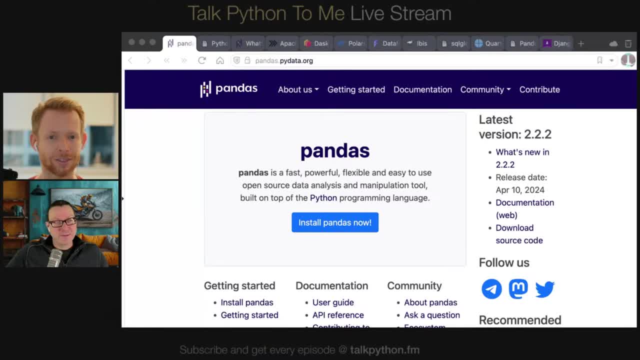 yeah, that's a lot of a lot of stuff going on and I think I mean it's interest is awesome, right? I mean, if there's just a different level of problems, I feel like you can, you could take on. you know, you know what I got this entire week and someone's that's. my job is to make this work rather than. 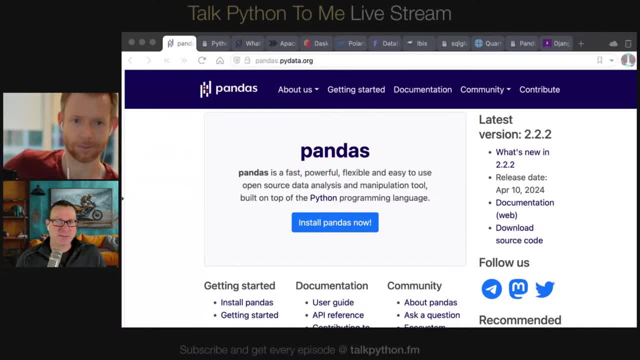 I've, I've got two hours and I can't really take on a huge project, and so I'll work on the smaller improvements or whatever. yeah, but I, I think, um, and I think many people know, but I, I haven't been involved day-to-day and panda since 2: 13.. so that's, that's getting on, that's, that's a lot. 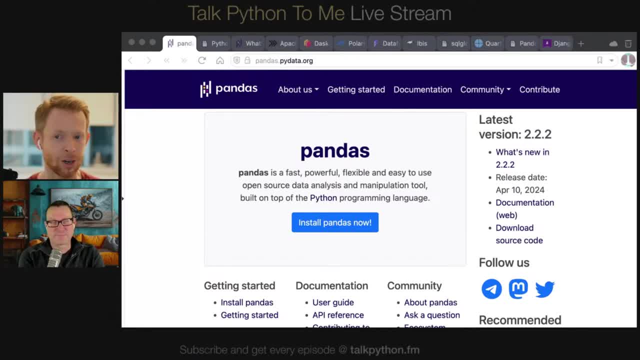 of that's a lot of years. um, you know I still um. you know I still talk to the pandas contributors um, we had a, we had a pandas meetup. um core core developer meet up here in Nashville. uh, pre-covered, I think it was in 20.. 19 maybe, um. so you know I'm still in active contact. 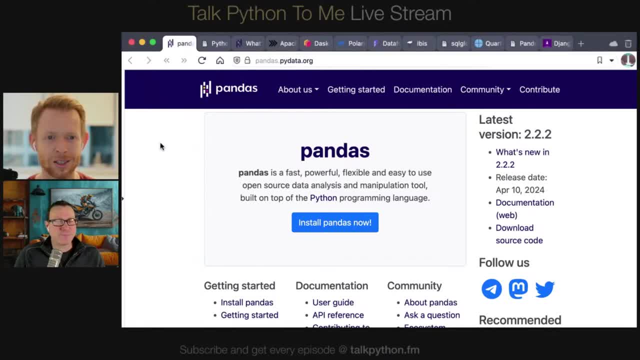 with the pandas developers, but, um, uh, it's, it's been a, you know, a different team of people leading the project. it's taken on a life of its own, which is, yeah, which is amazing. that's exactly that's. that's as an open, yeah, as a project creator. that's exactly what you want. um is to not be. 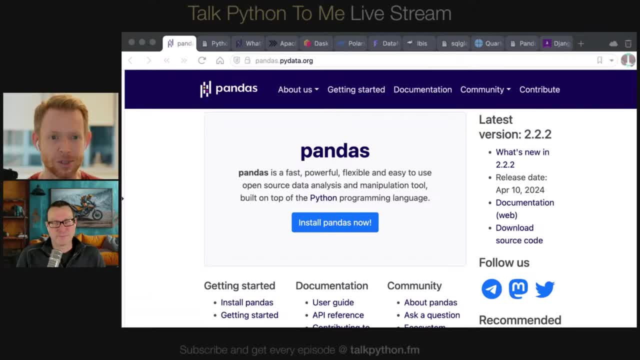 beholden to the, the project that you created, uh and forced and you know kind of uh, you know have to, you know be responsible for it and take care of it for, uh, the rest of the rest of your life. um, but if you look at like a lot of the community, a lot of the most kind of intensive community, 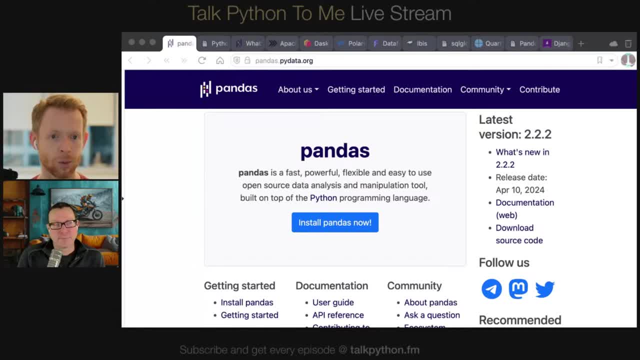 development has happened since, like since i, i moved on to work on on other projects, and so now the the project is- i don't know the exact count, but it's had thousands of contributors, and so, um, you know, to have thousands of different, unique individuals contributing to an open 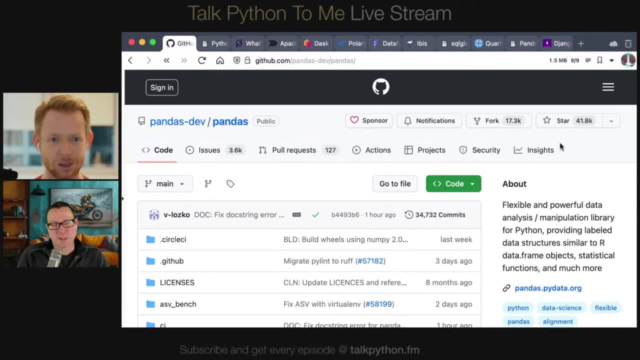 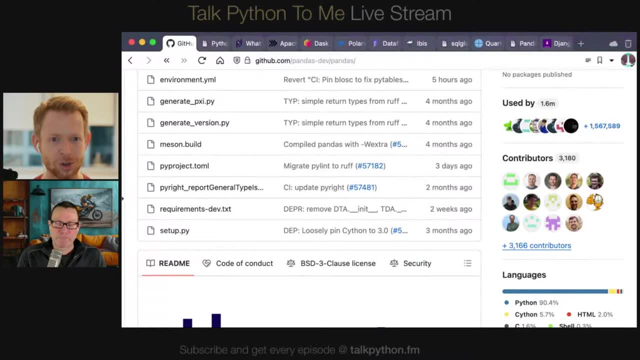 source project is: uh, it's, it's a big, it's a big deal. so i think, even i don't know what it says on the bottom of github. it says you know 30, 30, 200 contributors. but that's maybe not even the full story, because sometimes you know people, you know. 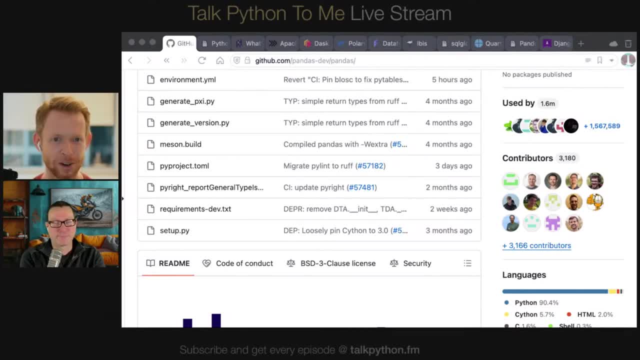 they don't have their email address associated, their github profile, and you know how github counts contributors. i would say probably the true number is closer to 4 000, so that's wow, yeah, but that's uh that. i think that's a testament, you know, to the uh, to the core team and all the outreach. 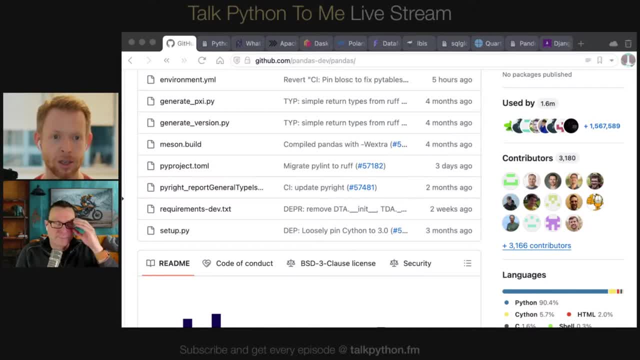 they've done and work making making the project accessible and easy to contribute to um. because if people, if you go and try to make a pull request to a project- and there's many different ways that that you can fail, so like either the project is technically, like there's issues with the build system or the 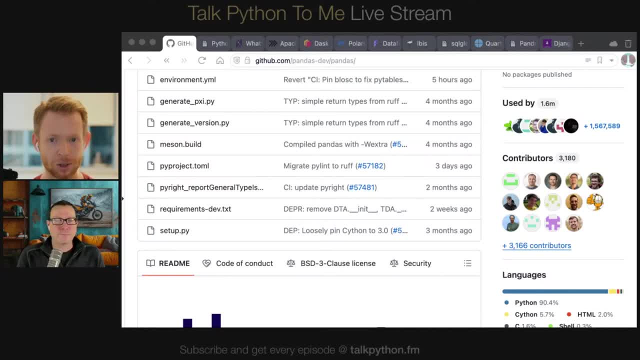 developer tooling, and so you struggle with the developer tooling, and so if you aren't working on it every day and every night, um, you can't make heads or tails of how the developer tools work. but then there's also, like, the level of accessibility of the core development team. 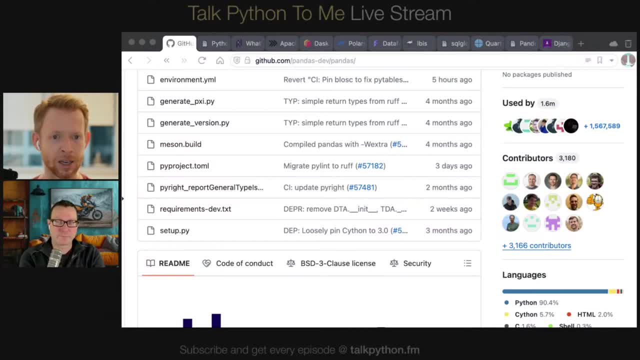 like, if they don't, if they aren't there to support you in getting involved in the project and learning how it works, and creating documentation, attribute and what's expected of you, um, that can also be, you know, a source of frustration where people uh churn out of the project, you know. 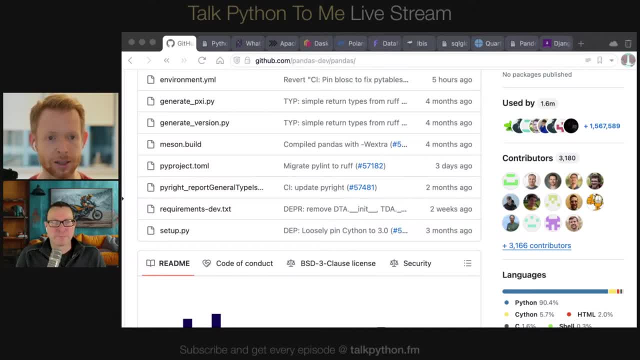 because it's just it's too hard to find their sea legs. um, and maybe, and maybe also, you know, sometimes development teams are um unfriendly or unhelpful or, you know, they make they make others feel like, um, they make others feel like they're annoyed with them or like they're 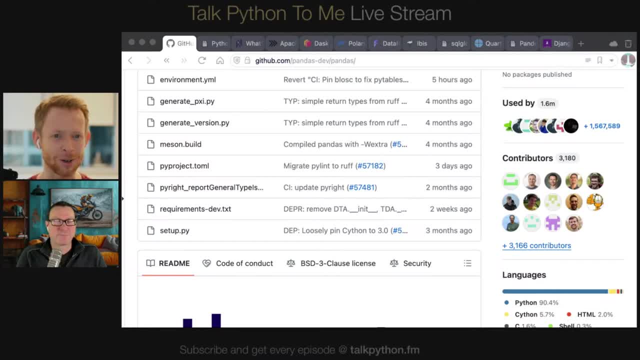 wasting their time or something. it's like i, i don't want to look at your, you know this pull request and give you feedback because you know i could do it more quickly by myself, or something like. sometimes you see that in open source projects, yeah, yeah, um, but they've, they've created. 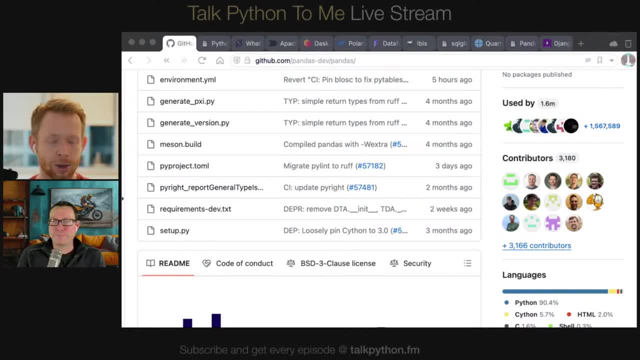 a very like they've. they've created a very welcoming, uh, very welcoming uh, environment and uh, yeah, i think the, the contribution numbers, speak speak for themselves. they definitely do. maybe last thing, before we move on to the other stuff you're working on, but the other interesting. 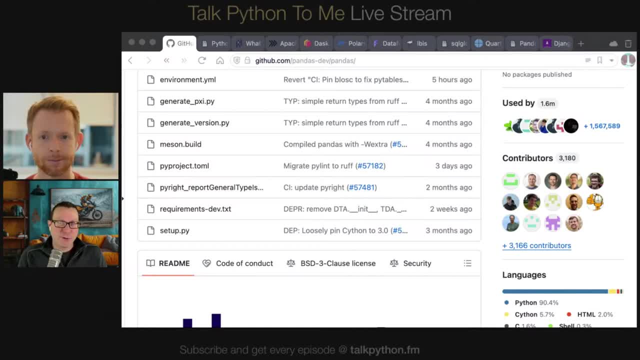 github statistic. here is the used by 1.6 million projects. that's. i don't know if i've ever seen used by that high. there's probably some that are higher, but not many. yeah, it's um, yeah, it's, it's, it's a lot of projects. um, i think it's, it's, it's, it's interesting, i think. 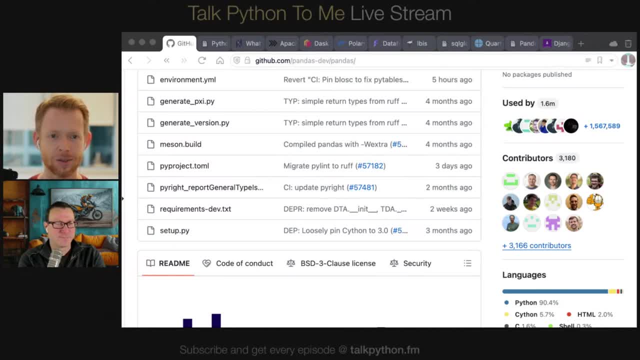 um, it's, it's like many projects. it's reached a point where it's it's a, it's an essential and assumed part of the of many, many people's toolkit, like they. uh, like, the first thing that they write at the top of a file that they're working on is, you know, import, import. 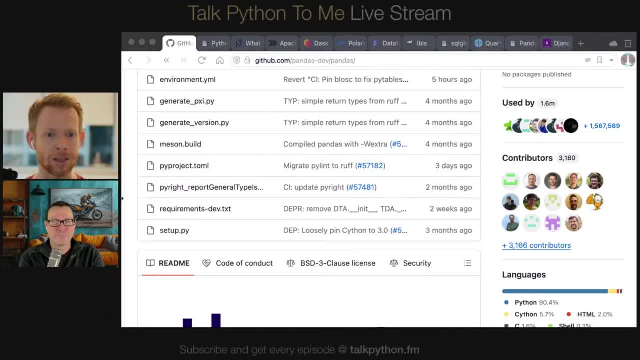 pandas as pd or import import numpy as pd and um, and so it's: uh, yeah, i think you know to create um. i think, in a sense, like i think one of the reasons why you know pandas has gotten so popular is that it is beneficial to it is beneficial to the community. 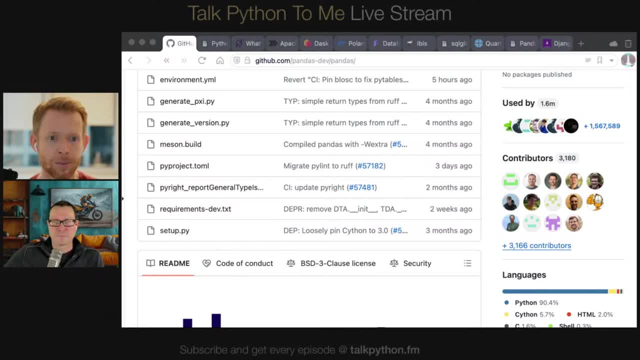 to the python community to have, um, you know, fewer solutions. you know kind of the zen of python. there should be one, and preferably only one obvious, obvious way to do things. and so if there were 10 different pandas like projects, um, you know, that creates skill portability problems and 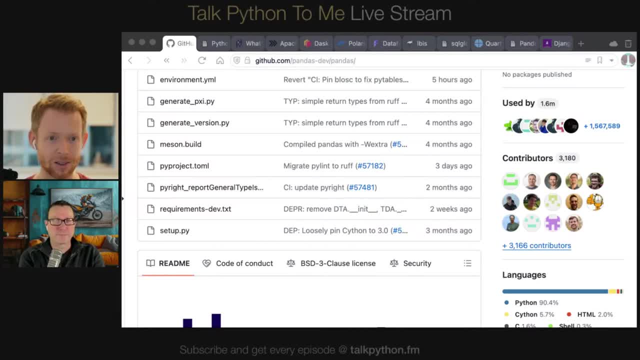 you know, it's just easier if everyone says, oh, we just pandas is the thing that we use. uh, change jobs and you can take all your skills like how to use pandas with you and um, i think that's also one of the reasons why python has become so successful in the business world is because 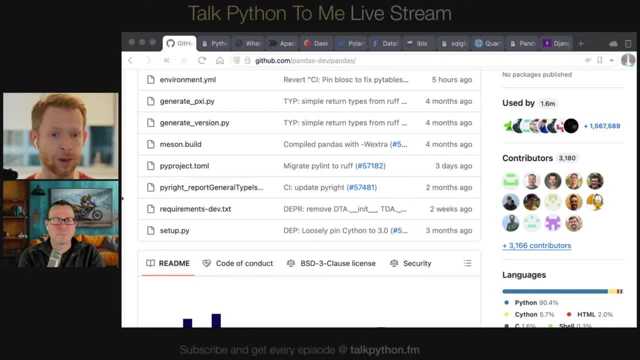 you can teach um somebody, even without a lot of programming experience, how to use python, how to use pandas and become productive doing um, doing. you know basic work, uh, very, very quickly, and so you know one of the solutions. i remember back in the early 2010s, there were a lot of 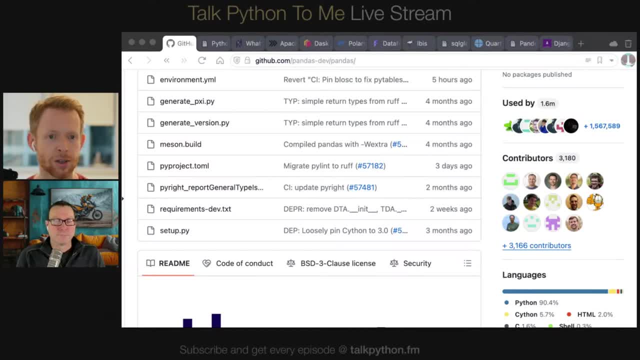 articles and talks about how to address the data science shortage, and my, my belief and i. i gave a um, uh, i gave a uh, a talk at web summit in dublin in 2000- gosh, maybe 2017, 2008, i have to look exactly- but basically it was the- the data science, data scientist shortage, and i and my 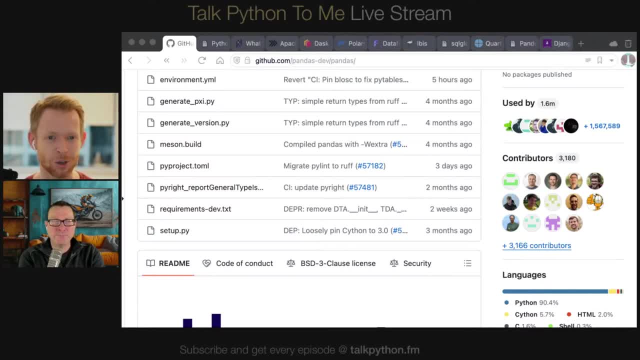 thesis was always it's we should make it easier to be a data scientist or like, like, lower the bar for, like, what sort of skills you have to master before you can. you can do productive work and work in a in a business setting, and so i think the fact that that there is just pandas and that's. 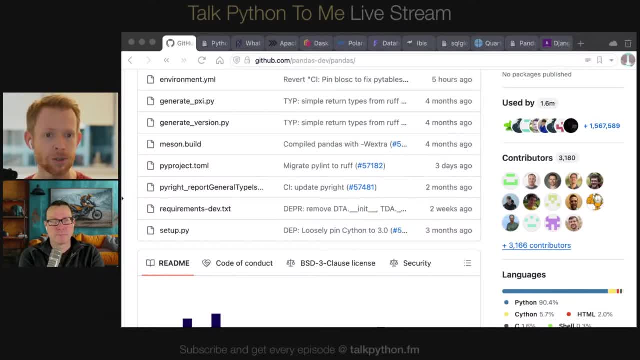 like the one thing that people have to have to learn how to, how to use is, like their essential, like starting point for doing any data has also led to this piling on of like people being motivated to make this, this one thing, better because it you know, you make. 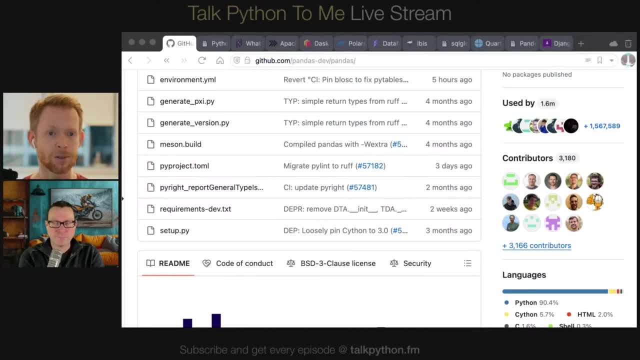 improvements to pandas and they benefit millions of projects and millions of people around the world, and that's uh, yeah, so it's like a, you know, steady snowballing effect. yeah, i agree with you and i think that i think doing data science is getting easier. we've got a lot of interesting frameworks and tools um share for python, one of them. 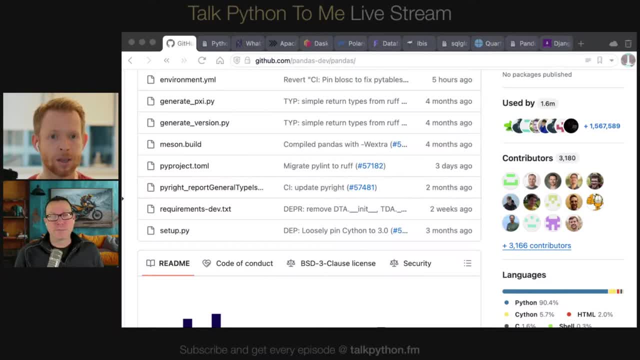 right, that makes it easier to share and run. run your code. you know yeah. so yeah, i think the um uh yeah, shiny shiny for python, uh, streamlit, you know dash like these different um interactive data application publishing framework so you can go from. you know, if you. 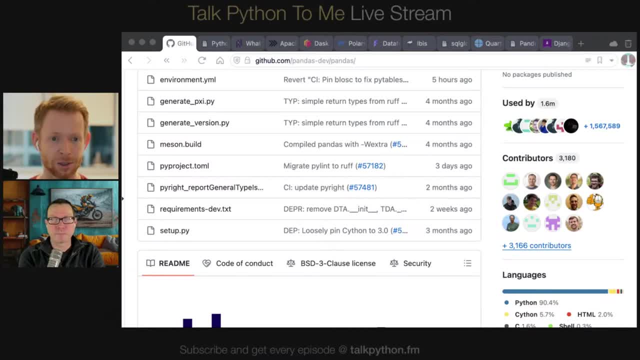 few, few lines of pandas code, loading some data and doing some analysis and visualization, to watching that as an interactive, interactive website, without having to know how to use any web development frameworks or nodejs or anything like that. and so to be able to, you know, get up and running and build a a working- you know- interactive web application, that's. 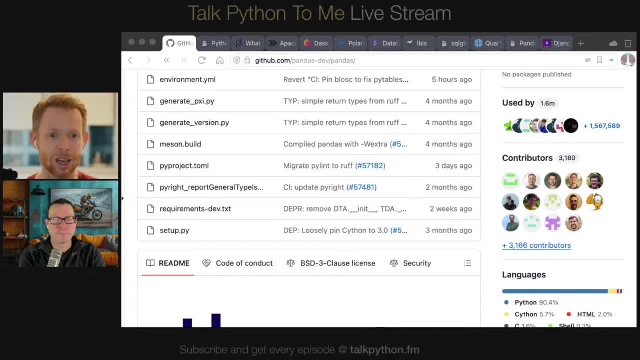 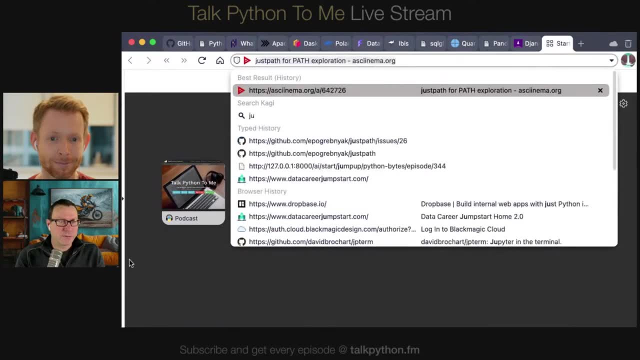 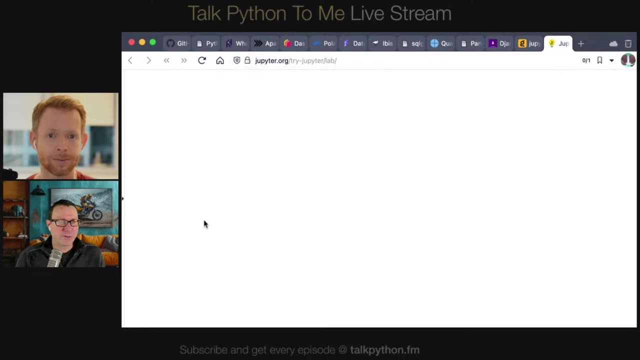 powered by powered by python, but yeah, it's, it's, it's a game changer in terms of, you know, shortening um end-to-end development life cycles. what do you think about a jupiter light and these um pyoxidide and basically jupiter, jupiter in a browser, yeah of things, yeah um. 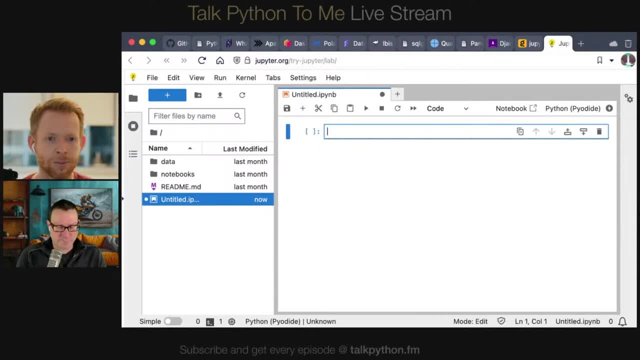 web assembly and all that. yeah, so i i uh definitely very um excited about. i've been following web assembly in general and so i guess uh some some people listening will know about, know about web assembly, um, but but basically it's a portable machine code that can be compiled and executed uh in within your browser in a sandbox environment. so 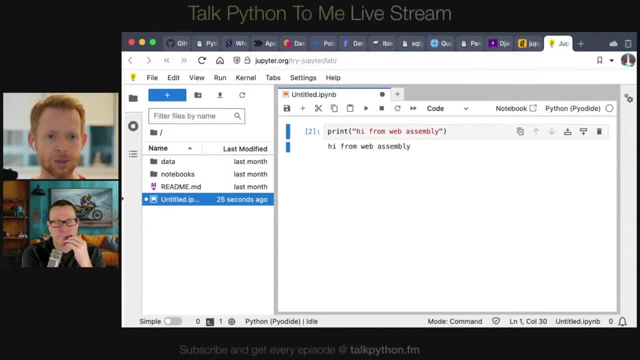 it. it protects against security issues and um allows prevents- like the person who wrote the web assembly code from doing something malicious on your, on your machine, which is very important. um won't necessarily stop them from, like you know, mining cryptocurrency while you have the browser tab open. that's a whole separate problem, but uh, but, yeah, i think it's, uh, it's enabled us to you. 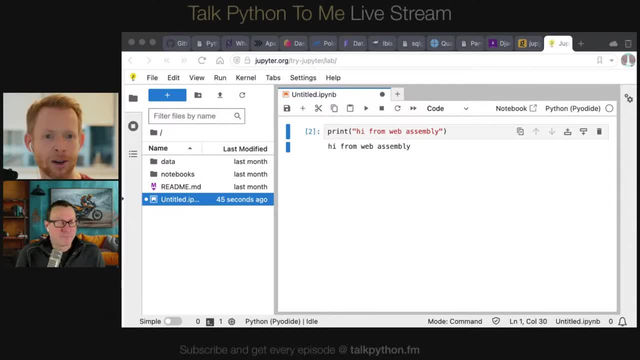 know run the whole scientific python stack, including jupiter and numpy and pandas, totally in the browser, without you know having a client and server and needing to. you know run a container someplace in the cloud and um, and so i think, in terms of creating application deployment, so like, 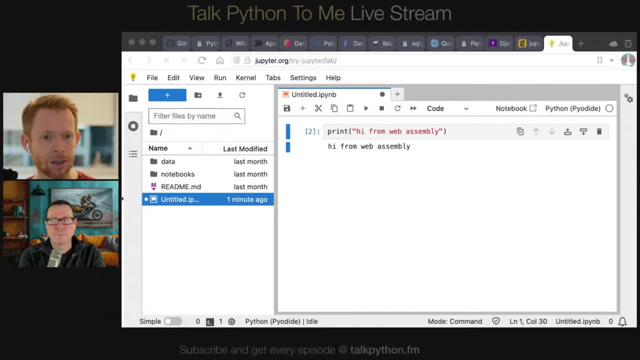 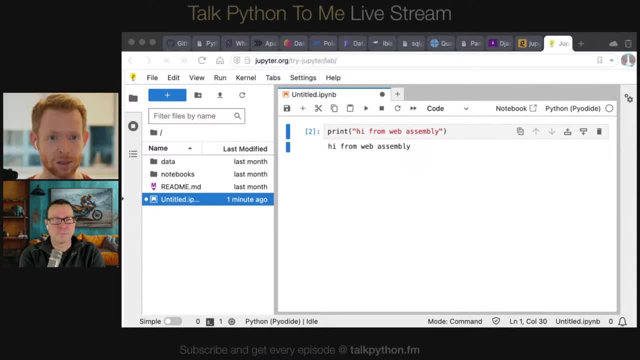 uh and opens. it, opens up new, new, new use cases, like new you know application architectures and make it makes things a lot for uh, because setting up and running a server creates brittleness, like it has cost, and so if the um, if the browser is doubling as your server process, like that's. 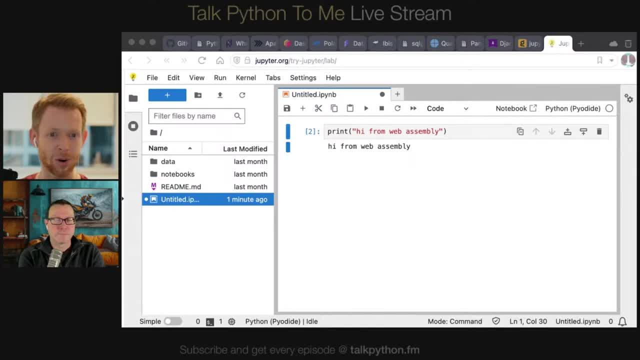 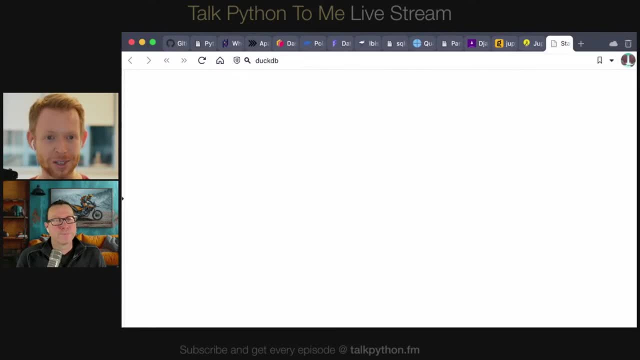 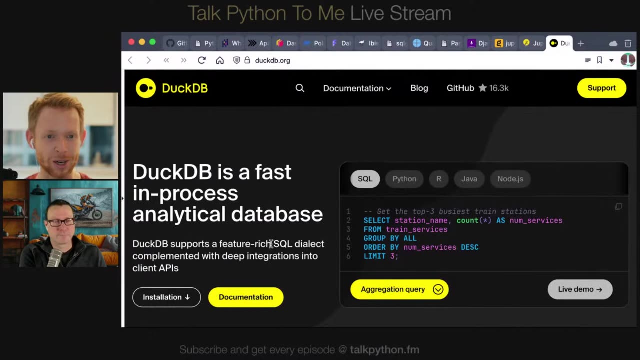 i think that's really cool. um, you also have, like, other projects like, uh, like duckdb, which is a you know high performance, uh, embeddable analytic sql engine, and so, you know, now with duckdb compiled to wasm, you can get a you know high performance database running in your browser, and so you can get. 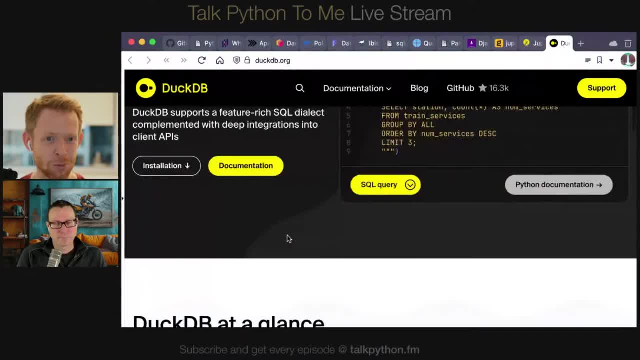 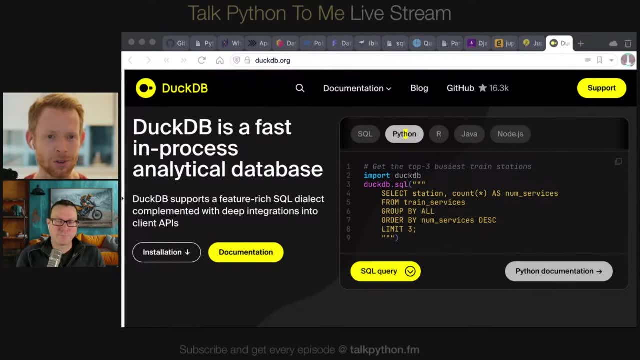 low latency, interactive queries and interactive dashboards, and and so it's- uh, yeah, there's um, it's, it's it's- web assemblies open up this whole kind of new world of of possibilities, and um, it's so, it's, it's it's transformative, i think, um. 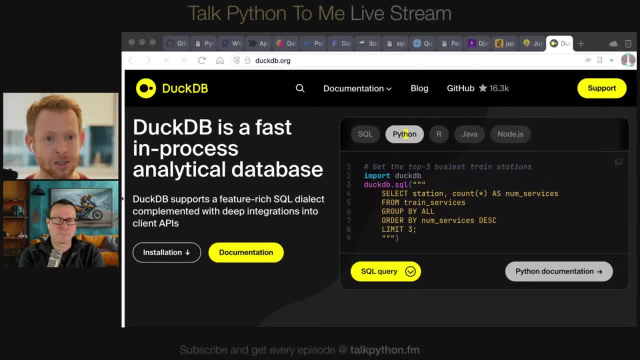 i think for for python in particular, you mentioned pyodide, which is uh kind of a whole package stack, so it's it's like a framework for um build and build and packaging and basically building an application and managing its dependencies so you could create a web assembly version of your application to be deployed like 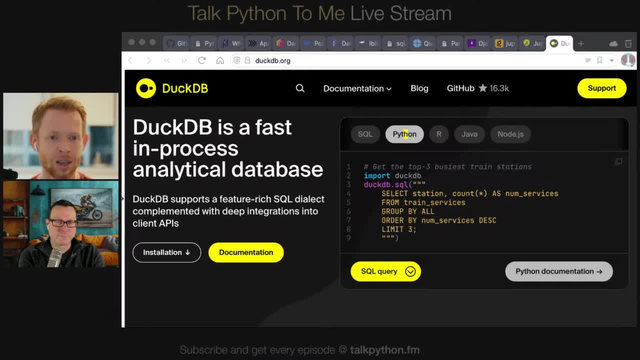 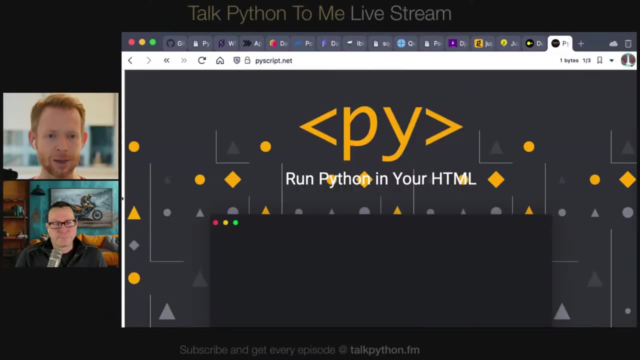 this, um, but uh, yeah, so i think i think the one of the pyodide is the pyodide main creator or maintainer went to anaconda. they create a pi script, uh, which made, which is another attempt to make it even easier to use python to uh, to make it even easier to use python to create uh web applications, uh, interactive. 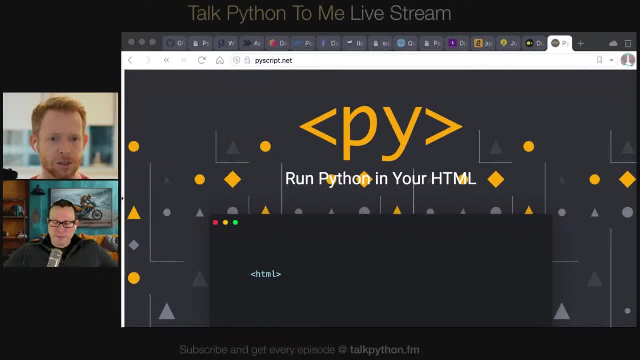 web applications and, um, yeah, so there's. there's so many cool things here. like in the r community, they have web r, which is, you know, similar to pi script and pyodide in some ways. like they have a lot of different ways of compiling the whole r stack to web assembly. there was just 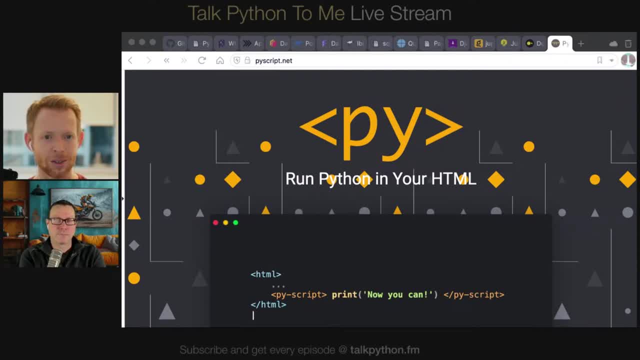 an article i saw on hacker news where um they worked on you know, figuring out how to get how to trick llvm into compiling fortran code like legacy fortran code to to web assembly. because when you're talking about all this you know scientific computing stack. you need the linear. 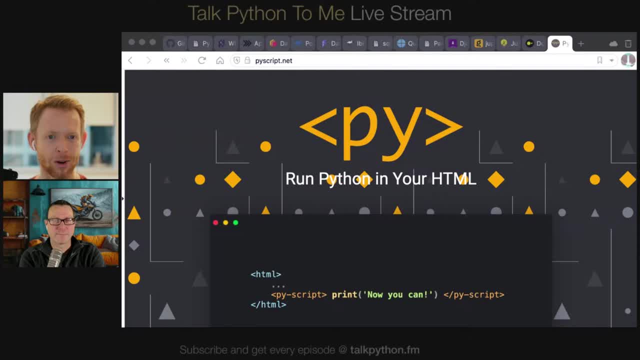 algebra and all of the- you know- 40 years of fortran code that have been built to support scientific applications. like you need all that to compile too and and run in the browser. so yeah, that's pretty wild to think of putting that in there, but very useful. i didn't realize that. 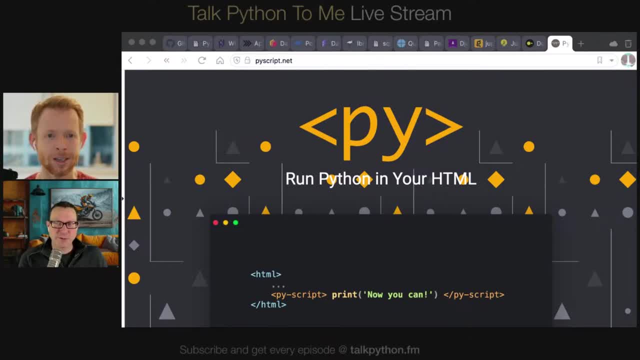 you could use duck db as a web assembly component. that's pretty cool, yeah, like there's. there's a company- uh, i'm not an investor or plugging them or anything, but it's called evidencedev and they, they, uh it's like a whole beat like business intelligence. um, open source business intelligence. 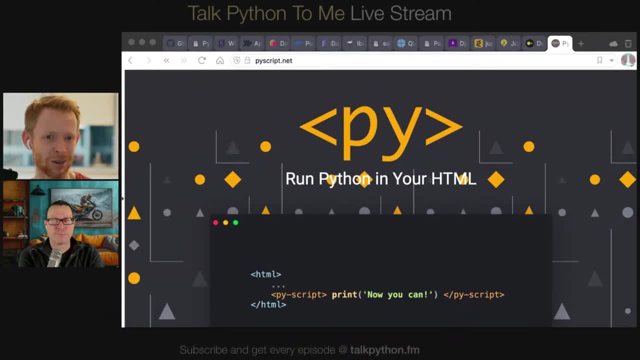 application that's uh, powered by, powered by duck db, and so, uh, if you have data that that fits in the browser, you know to have a whole like interactive dashboard or be able to do business intelligence like fully, like fully in the browser, with no need of a, no need of a server. 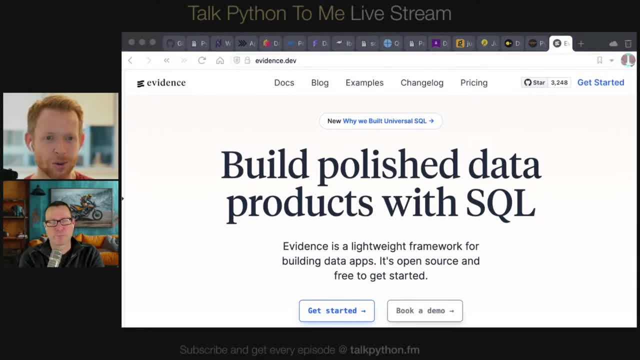 um, it's, uh, yeah, it's, it's, it's, it's very, very cool. so i'm, yeah, i've been uh following duck db since the early days and, um, you know, my company uh, voltron data, like you know, we we became members of the duck db foundation and built, you know, built actively build a relationship with them and they've 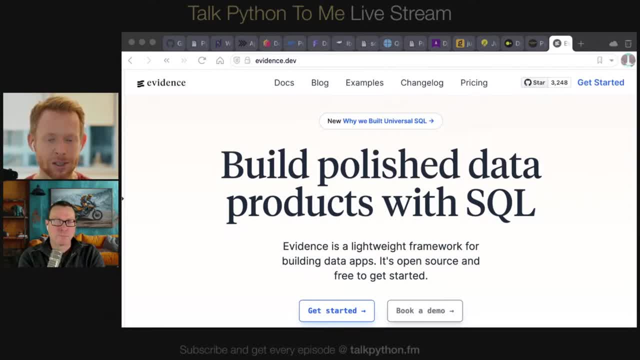 uh developed a partnership with, with duck db labs so we could help uh accelerate progress in this space, because i think the impact, the the impact is so uh is so immense and we, just we- it's hard to predict like what, um you know what people are going to build, um build with all this stuff and um. 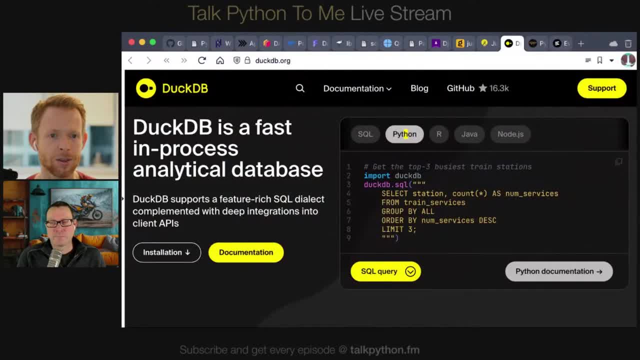 and so that was all you know with, i guess, going back, you know, 15 years ago to python, like one of the the reasons i became so passionate about building stuff for python was about in i think the way that peter wang puts that. it puts it is, you know, giving uh people superpowers. 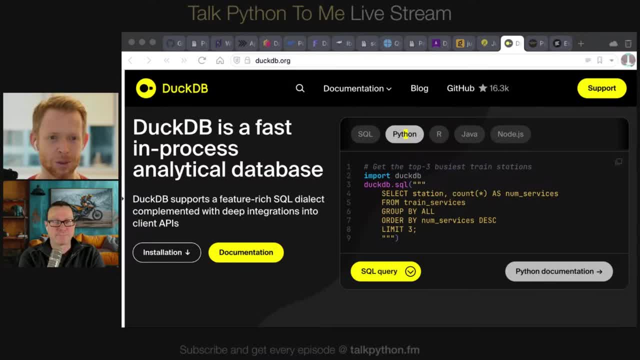 so we want to, uh, enable people to build things with much less code and much less time, and so, by making it things that much more accessible, that much easier to do, like in the mantra and pandas was like how, how do we make things? you know one line of code, or like this: that must be easy. 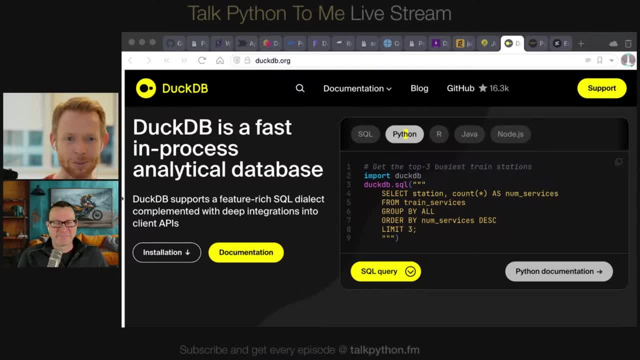 it's like one line of code. one line of code. it must be like like: make this as terse and simple, yeah, as possible, so that you can move on and focus on building the more interesting parts of your application rather than struggling with how to read a csv file, or you know how to do, you know? 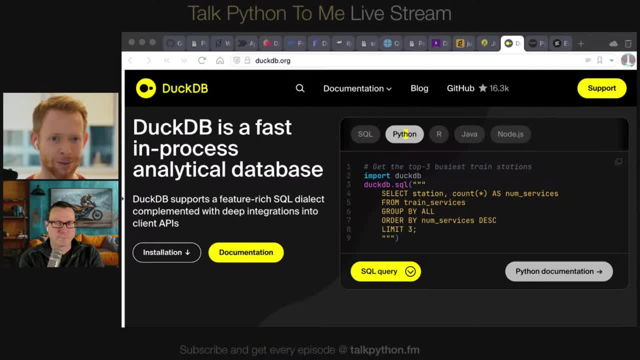 whichever, um, whichever you know, data munging, um technique that you need for your, for your data set. maybe an interesting mental model for duck db. it's kind of an equivalent to sqlite, but more analytics database for folks you know in process. yeah, things right, what do you think? yeah, 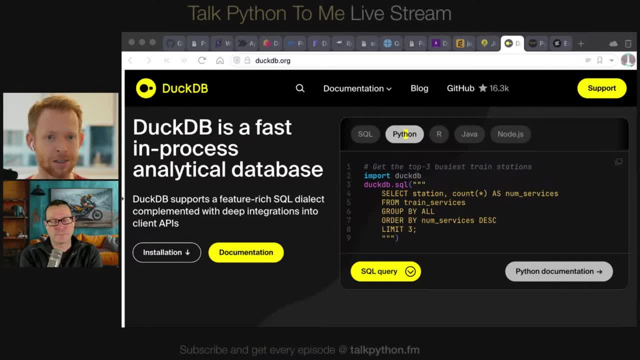 so, yeah, duck db is like sqlite and in fact it it can run the whole sqlite test suite, i believe. so it's a full database, but it's uh, it's uh, um, it's for analytic processing, so it's optimized for, for analytic processing and uh, as compared, you know, with sqlite, which is not um, it's, it's not designed for, for. 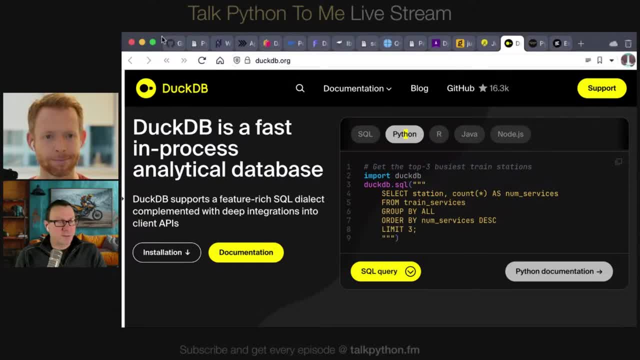 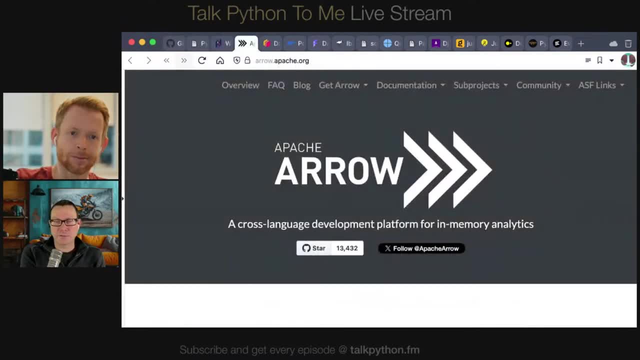 data processing. yeah, cool, all right. well, let's talk about some things that you're working on beyond pandas. uh, you talked about apache arrow earlier. um, what's, what are you doing with the arrow and and how's it fit in your world? yeah, so the the, the back story there was, uh, i don't know if you can hear the sirens in- uh, 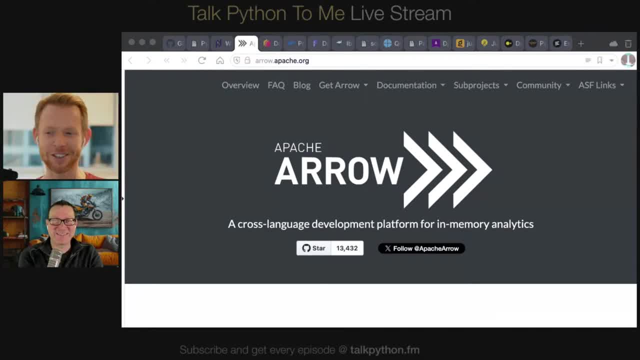 in downtown nashville. but no, actually it's, that's good, it's filled, the microphone filters it out, filters it out pretty well. um, yay for um, dynamic microphones. they're amazing. yeah, so in, uh, like around the mid, like the mid 2010s, 2015. um, i had a lot of trouble with the. 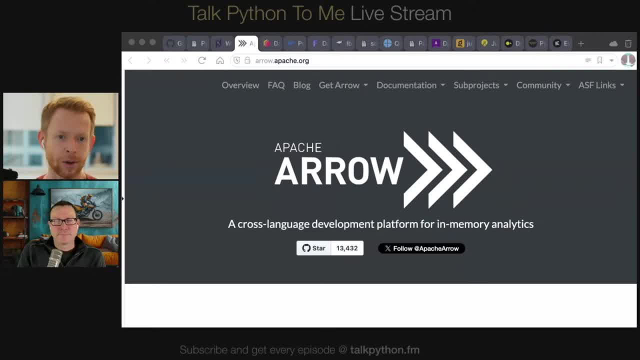 I started working at Cloudera, which is a company that was one of the pioneers in the big data ecosystem, And I had spent several years working on five, five years, five, six years working on pandas, And so I had gone through the experience of building pandas from top to bottom. 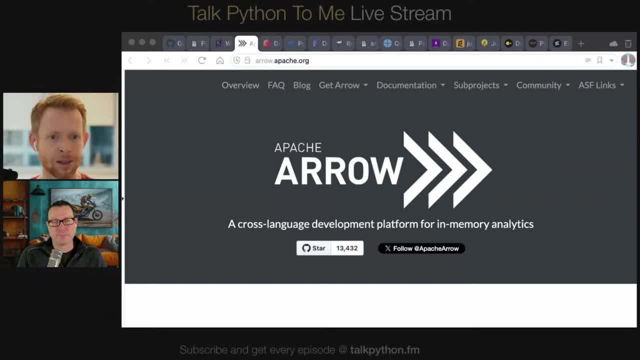 And it was this full stack system that had its own mini query engine, all of its own algorithms and data structures and all the stuff that we had to build from scratch. And I started thinking about you know what, if it was possible to build some of the underlying computing technology, like data readers, like file readers, all the algorithms that power the core components of pandas, like group operations algorithms- 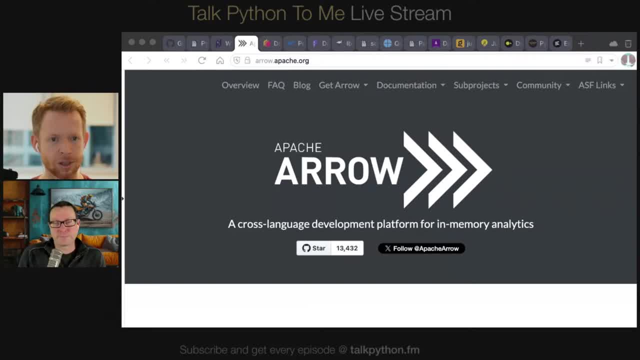 Like what if they were possible to have a general purpose library that isn't specific to Python but is really really fast, really efficient and has a large community building it, so that you could, you know, take that code with you and use it to build many different types of libraries, not just data frame libraries, but also database engines and, you know, stream processing engines and all kinds of things. 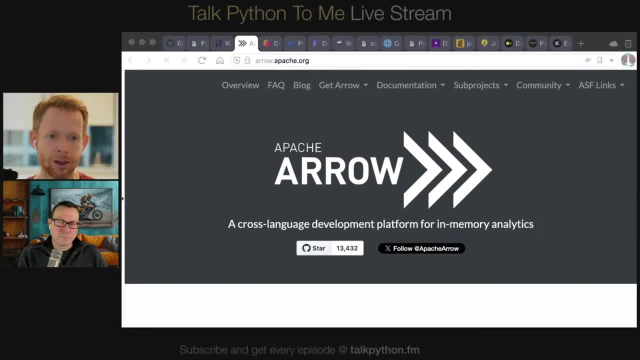 And so that was it, And so that was kind of what was in my mind when I started getting interested in what turned into Arrow, And one of the problems we realized we needed to solve- this was like a group of other open source developers and me- was that we needed to create a way to represent data that was not tied to a specific programming language. 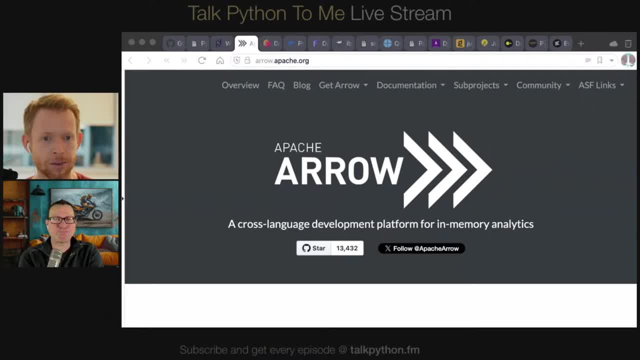 And that could be used for a very efficient interchange between components. And the idea is that you would have this immutable like this, This kind of constant data structure which is like it's the same in every programming language, And then you can use that as the basis for writing all of your algorithms. 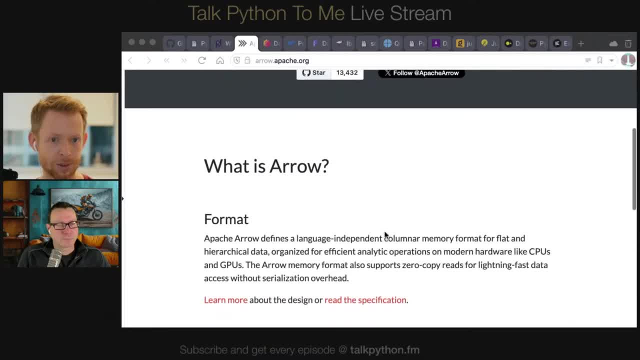 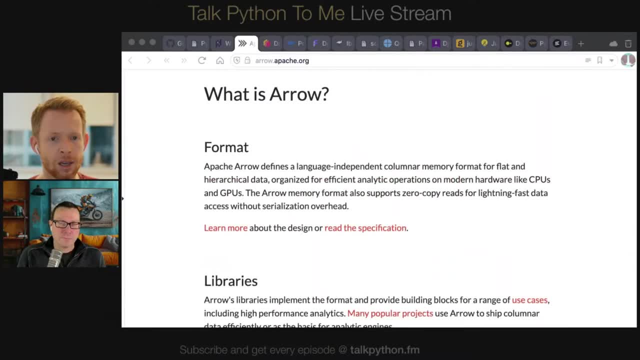 So, as long as it's Arrow, you have these reusable algorithms that process Arrow data. So we started with building the Arrow format and standardizing it, And then we've built a whole ecosystem of components, like library components and different programming languages for building applications that use the Arrow. 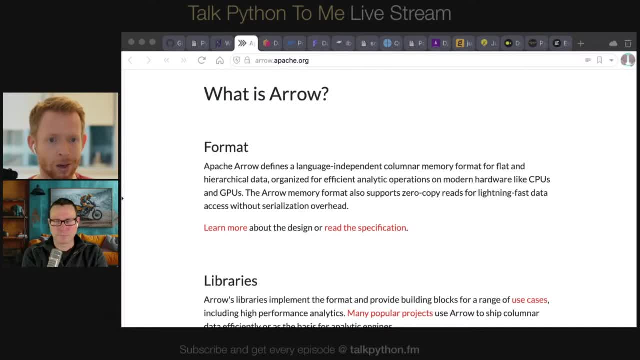 So that includes you know not only tools for building and interacting with the data, but also file readers So you can read CSV files and JSON data and Parquet files. read data out of database systems. You know wherever the data comes from. we want to have an efficient way to get it into the Arrow format. 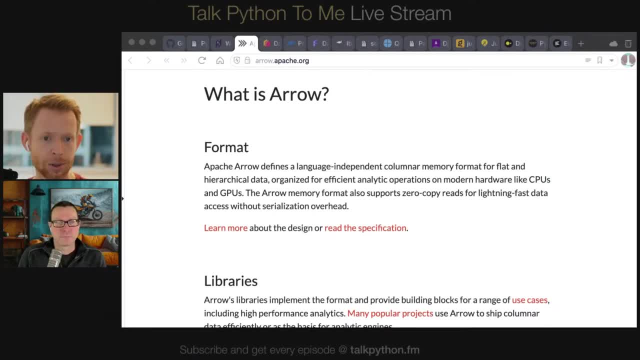 And then we moved on to building data processing engines that are native to the Arrow format, so that Arrow goes in, The data is processed, Arrow goes out. So DuckDB, for example, supports Arrow as a preferred input format and is DuckDB is more or less Arrow-like in its internals. 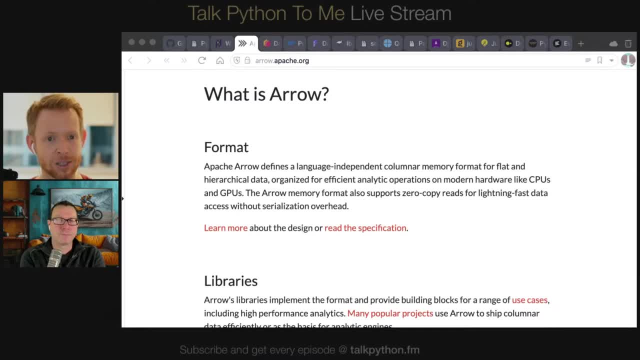 It has kind of Arrow Arrow format plus a number of extensions that are DuckDB, DuckDB, specific for better performance within the context of of DuckDB, And so so in numerous communities. so there's the Rust community, which has built DataFusion, which is an execution engine for Arrow. 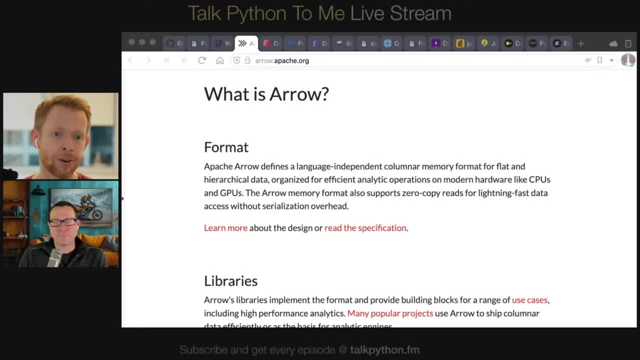 SQL engine for Arrow. And so, yeah, we've kind of like looked at the different layers of the stack, like data access, computing, data transport- you know everything under the sun. And then we've built libraries that are across many different programming languages, that are you can pick and choose the pieces that you need to build your, build your system. 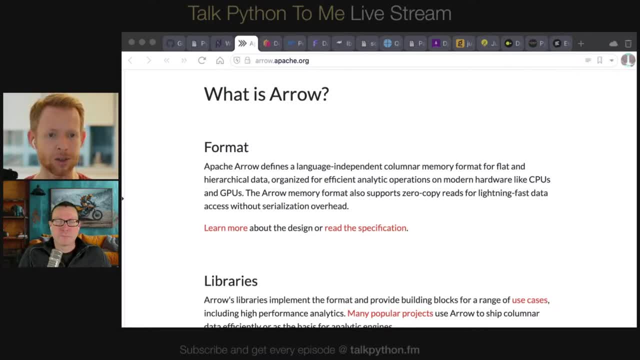 And the goal, ultimately, was that we in the future, which is now- we don't want people to have to reinvent the wheel Whenever they're building something like Pandas, that they could just pick up these off-the-shelf components, they can design the developer experience, the user experience that they want to create and and they can get built, you know. so, if you were building Pandas now, you could build a Pandas-like library based on the Arrow components in much less time. 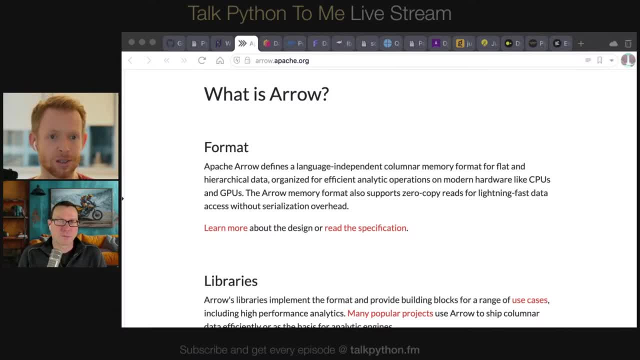 And it would be. it would be fast and efficient and interoperable with the whole ecosystem of other projects that use Arrow. Yeah, So it's, it's. it's very cool, It's. I mean, it was really ambitious in some ways obvious to people. 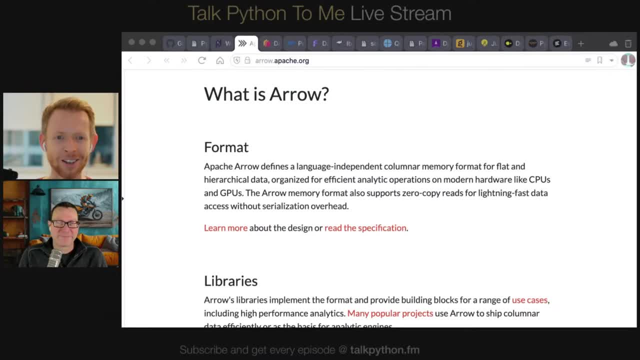 They would. they would hear about Arrow and they'd say: that sounds obvious, Like clearly we should have a universal way of transporting data between systems and processing it in memory. Why hasn't this been done in the past? And it turns out that, as is true of many open source software problems, that that many of these problems are the social problems are harder than the technical problems. 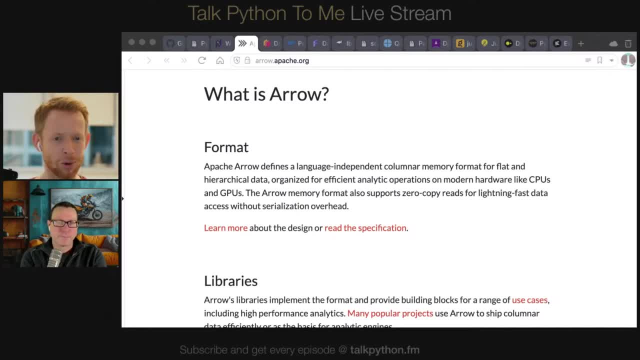 And so If you can solve the the kind of people, coordination and consensus problems, solving the technical issues is much, much easier by comparison. So I think we were lucky in that we found, like the right, you know, the right group of people, the right personalities, where we were able to. you know, as soon as I met, I met Jacques Nadeau, who had been at MapR and we, you know, was working on his, his startup, Dremio. 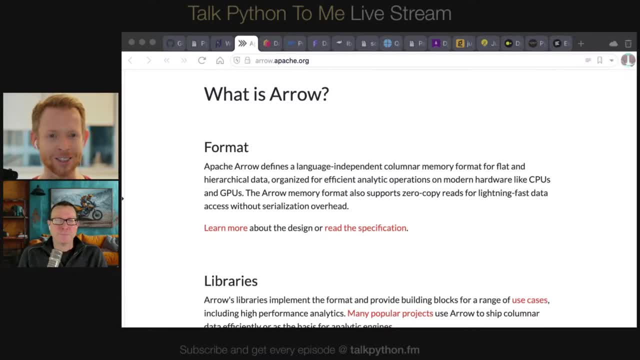 So, like I knew instantly, when I met Jacques Nadeau, I was like it's like I can work. he's like, it's like him, like he's going to help me make this happen. I met Julien Ledem, who had also co-created Parquet. 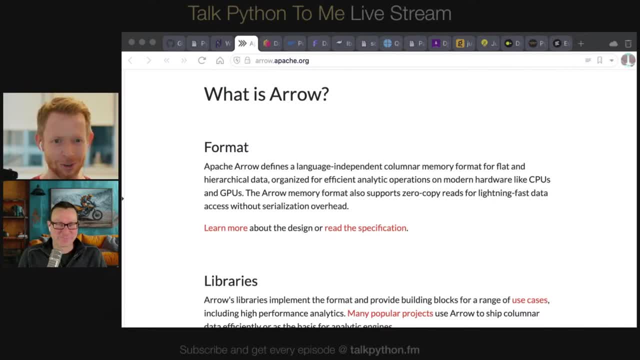 I was like, yes, like we are going to make this, like, like we, like I found the right people, like we are, we are going to make this happen. So it's been a. it's been a labor of love and and and and much, much work and and stress and everything. 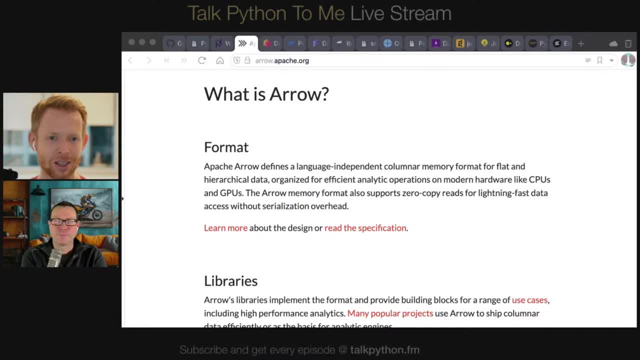 But it's yeah, that's. you know I've been working on things circling, you know, with Arrow is the sun. You know I've been building kind of satellites and moons and planets circling the the, the Arrow sun, over the last, over the last eight years or so. 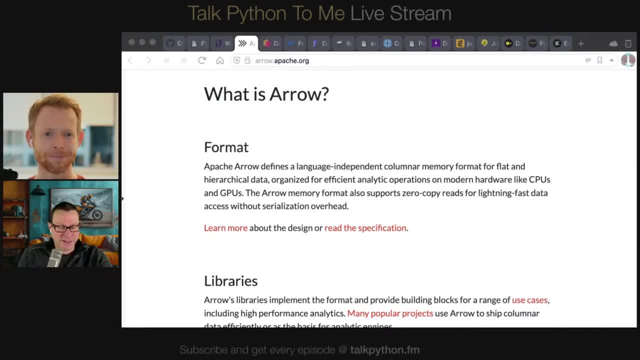 And that's kept me pretty busy. Yeah, it's only getting more exciting and interesting Over here. it says it uses efficient analytic operations on modern hardware like CPUs and GPUs. One of the big challenges of Python has been the GIL, also one of its big benefits. 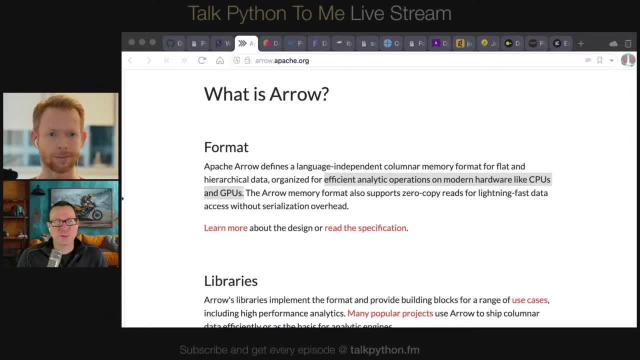 But one of its challenges when you get to multicore, More computational stuff, has been the GIL. What's the story here? Yeah, so in in in Arrowlands, when we're talking about analytic efficiency it, it mainly has to do with the like underlying, like how the how modern CPU works, or how how how a GPU works. 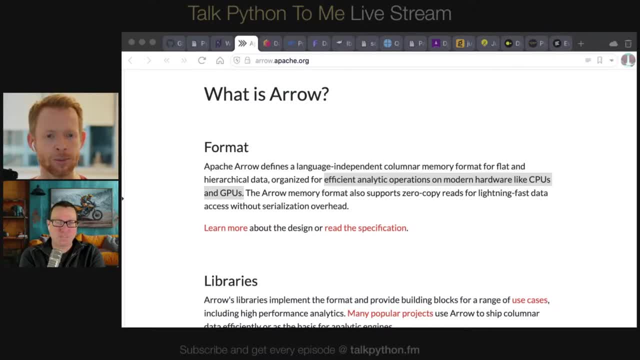 And so when the data is arranged in column oriented format that enables the, The data to be moved efficiently through the CPU cache pipelines, So the data is made, made available efficiently to the, to the CPU cores. And so we spent a lot of energy in Arrow making decisions, firstly, to enable very cache, like CPU cache or GPU cache, efficient analytics on on the data. 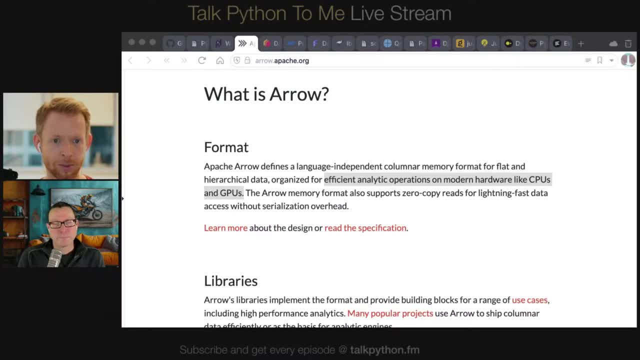 And so so we were kind of always we were deciding. we would break ties and make decisions, But Based on, like, what's going to be more efficient for the, for the computer chip. The other thing is that modern- and this is true with GPUs, which have a different parallelism model than, or a different kind of multicore parallelism model than, CPUs- 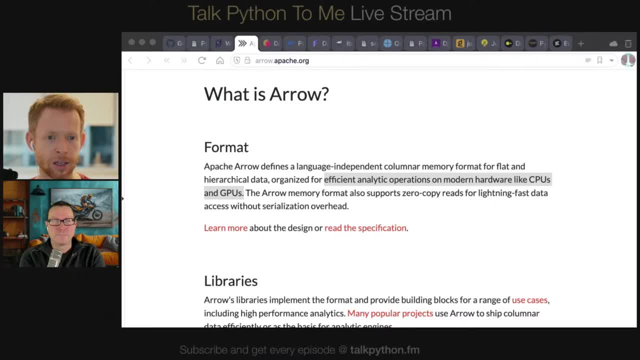 But in CPUs they've focused on adding what are called single instruction, multiple data, intrinsic like built-in operations in the processor. So It is the best thing you can do Where you know. now you can process up to 512.. 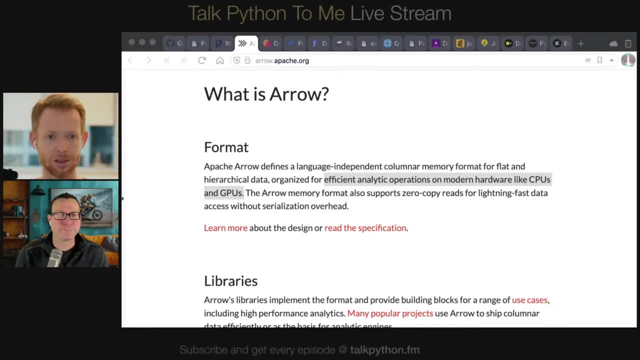 Bytes of data in a single CPU instruction, And so that's like you know my brain's doing the math right, Like 16,, 32 bit floats, or you know eight, 64 bit integers in a single Cycle. 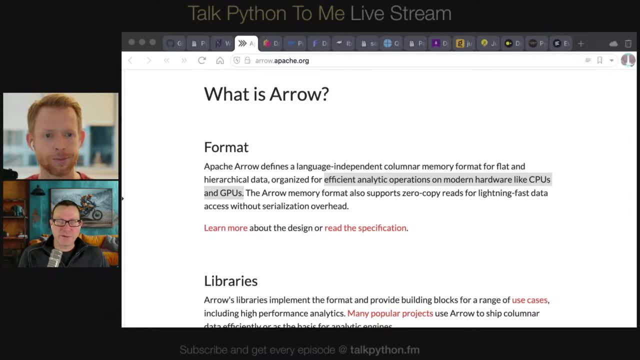 There's like intrinsic operations: Multiply this number by that one, Multiply that number to these eight, things all at once, Something like that. That's right, Yeah. Or you might say like: oh, I have a bit mask and I want. 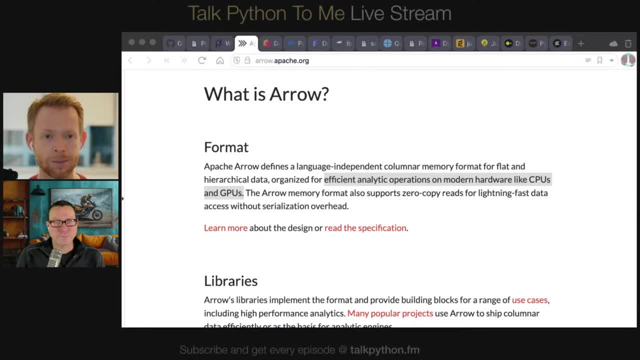 to select. i want to gather, like the, the, the one bits that are set in this. you know, this bit mask from this array of of integers, and so there's like a gather instruction which allows you to select a subset, a sort of a simd vector of integers, you know, using a bit mask, and so that 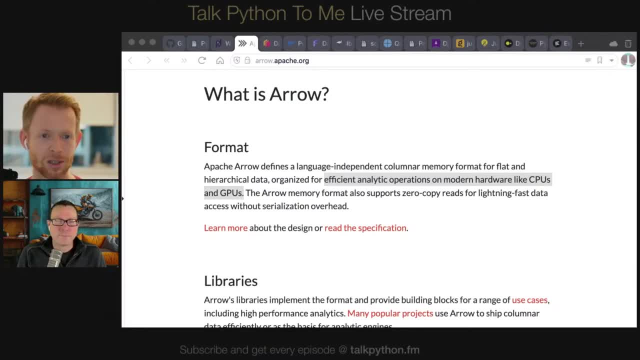 you know, turns out to be like a pretty, you know, pretty critical operation in certain, uh, certain data analytic workloads, um. so, yeah, we were really, you know, we wanted to have a data format that was, um, essentially, you know, future-proofed in the sense that it's some it's. 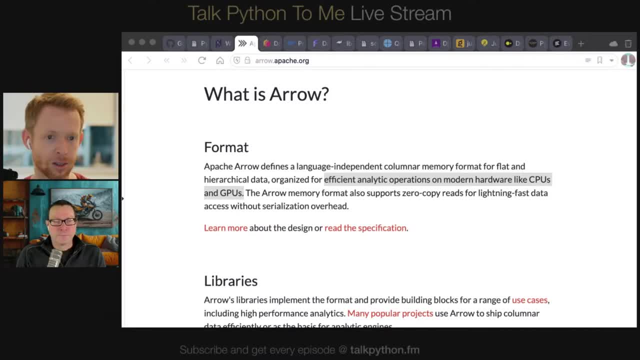 ideal for the coming wave, like current current generation of cpus, but also um, given that a lot of processing is moving to gpus and to fpgas and and to custom silicon. like we wanted arrow to be usable there as well, and it's arrow's been- successfully, you know- used as the, the foundation of. 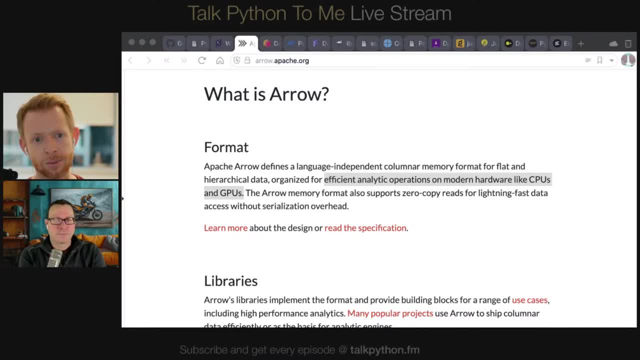 um gpu computing libraries, like we, um, you know, kind of voltron data built. we've built a whole um accelerator native, gpu, native, um you know, scalable execution engine, that's that's arrow based and um, and so i think the fact that we, that was our aspiration and we've been able to prove, 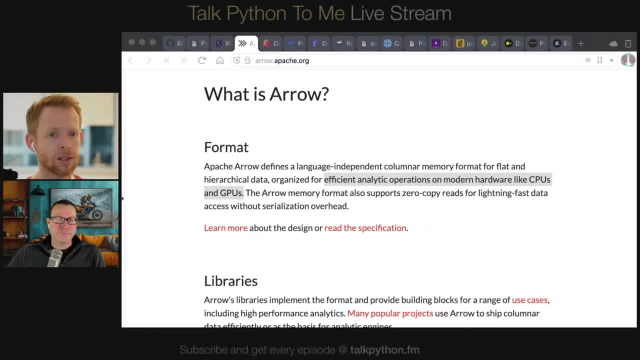 that out in in real world workloads and show the the kinds of efficiency gains that you can get with um using modern computing hardware. uh, correctly, or at least as well as it's intended to be used, um that's. that's a big deal in terms of, like making applications faster, reducing the carbon footprint of large. 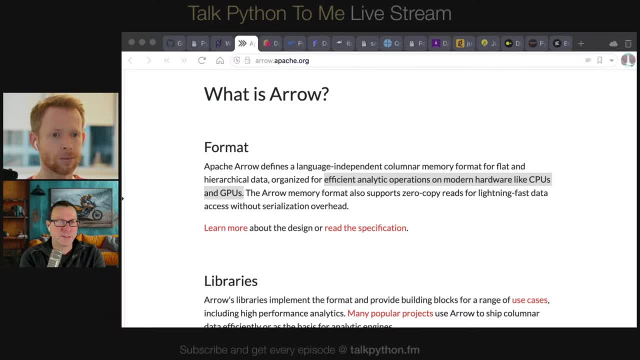 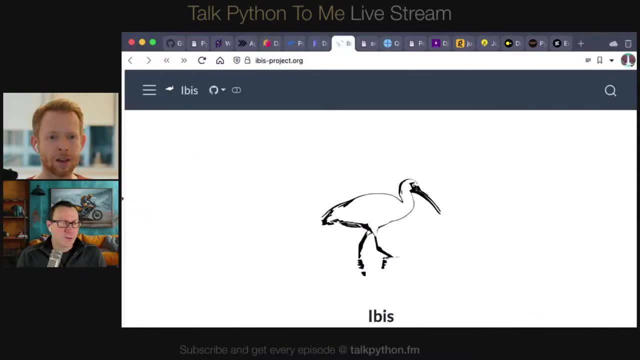 scale, data workloads, things like that- yeah, amazing. all right, let's see. what else have i got on deck here to talk to you about? uh, let's- yeah, maybe we could talk about. uh, we got a little time left, we gotta- yeah, let's, we can talk about this. um, yeah, we could. we could probably spend another hour talking. 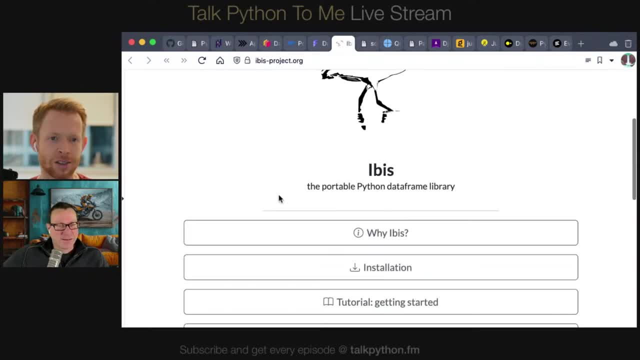 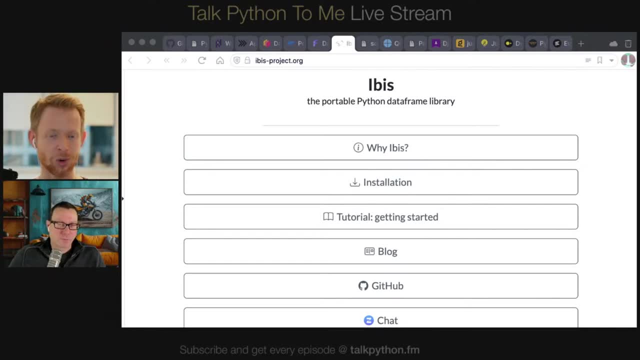 about this. i think, uh, i think one of the more interesting areas in in recent years has been um new data frame libraries and data frame apis that that transpile or compile to different uh execute on different back ends, and so around the time that that i was helping start arrow. 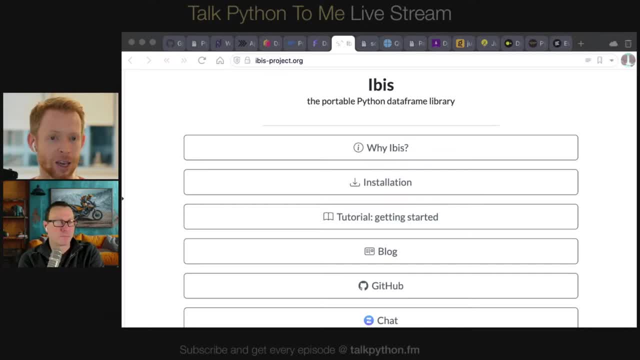 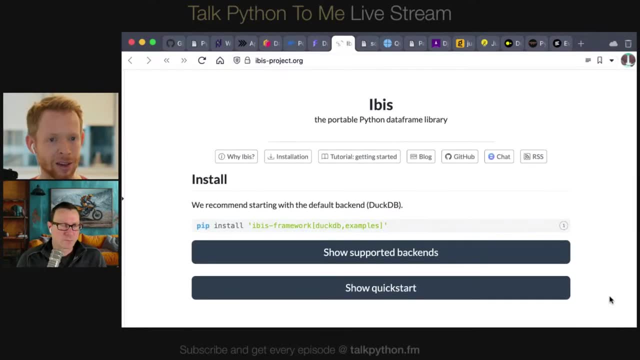 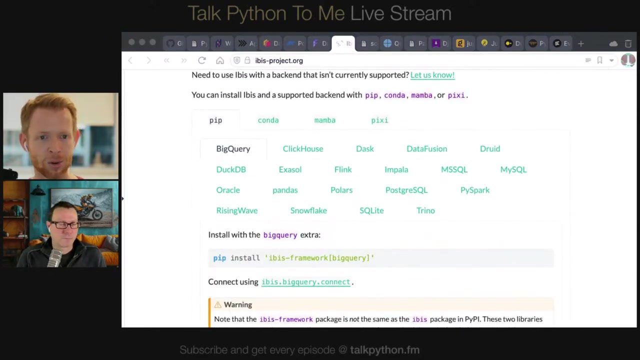 i created this project called ibis, which, uh is basically a portable data frame api that knows how to generate um sql queries and compile to pandas and pullers and different data frame data frame backends, and the goal is to provide a really productive data frame api that gives you portability across uh different execution backends, with the goal of 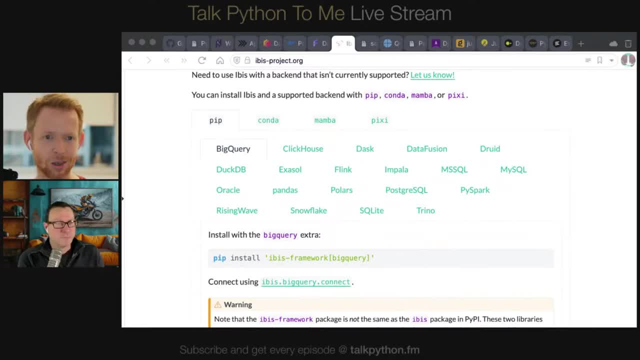 enabling what we call the multi-engine data stack, so you aren't stuck with using one particular system because all of you, the code that you've written, is specialized to that system. you have this tool which, um, so maybe you could work with. you know, duck db on your laptop, or pandas, or. 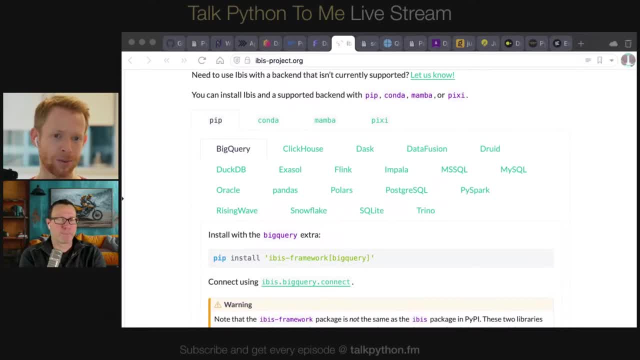 you could work with ibus on your laptop. but if you have, if you need to run that workload someplace else, maybe with you know click house or bigquery, or maybe it's a large, big data workload that's too big to fit on your laptop and you need to use spark sql or or something that you can just. 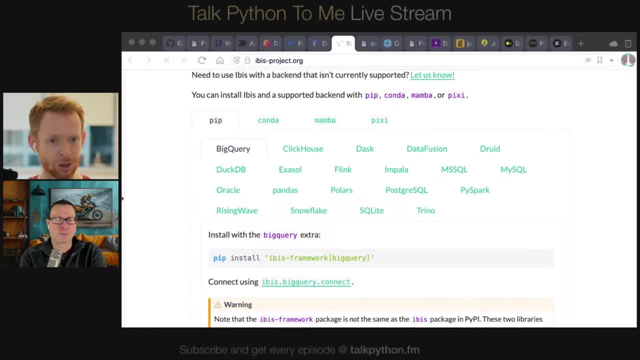 ask, ibis say, hey, i, i want to do the same thing on this larger data set over here and it has all the logic to to generate the correct, um, you know, query representation and run that workload for you. so, um, but there's a whole wave of, like you know, work right now to help enable people to work in a. 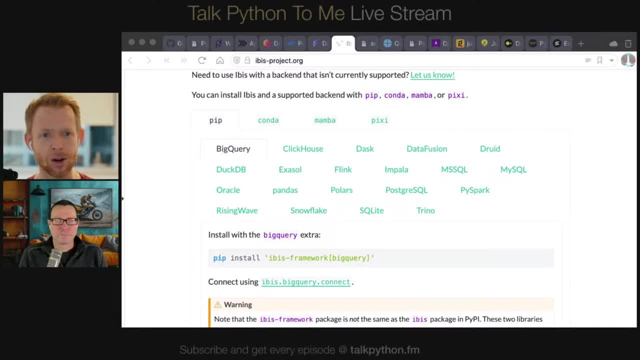 pandas like way, but get work with big data or, you know, get better performance than pandas, because pandas is a swiss army knife but, is you know, isn't a chainsaw. so it, uh it, it isn't. um, you know, if you were rebuilding pandas from scratch, it would end up a lot. um, you know, there's areas of the project. 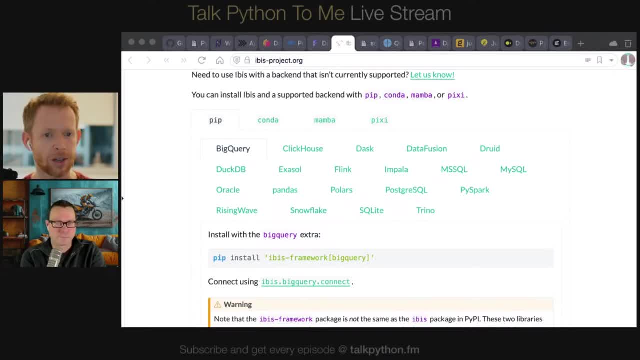 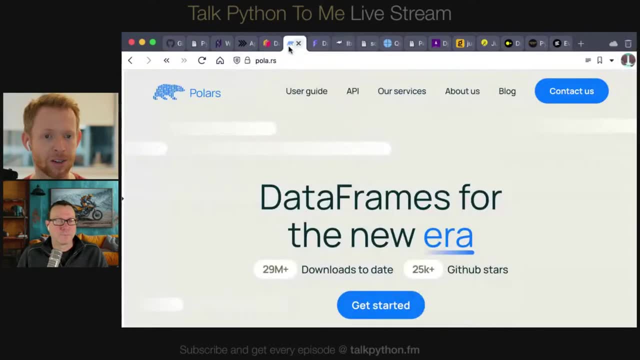 that are, you know, more bloated or have performance overhead. that's hard to get rid of and so that's why you have. you know, richie fink uh started the polars project, which is kind of a reimagining of of pandas um pandas: data frames written in rust and exposed in python. 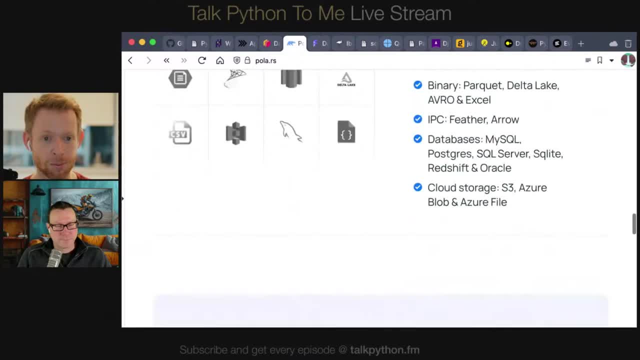 um and polars. of course is uh built on apache arrow at its core, um. so you know building a aero native data frame library and rust, and you know all the benefits that come with uh. you know building uh python extensions and rust. you know you avoid the gil. 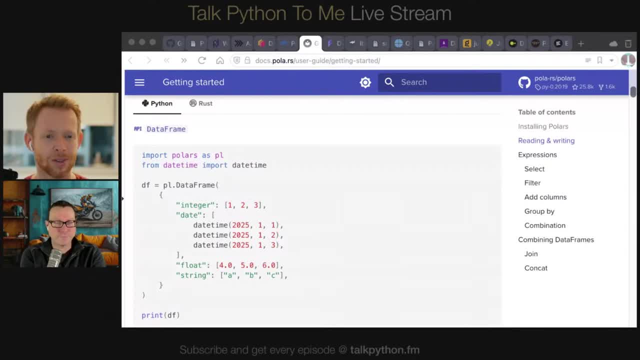 and you can manage the multi-threading in a systems language. all that, all that fun stuff. yeah, when you're talking about aero and supporting different ways of using it and things being built on it, certainly polar is keeping in mind for me. you know, when you talk about ibis, i think. 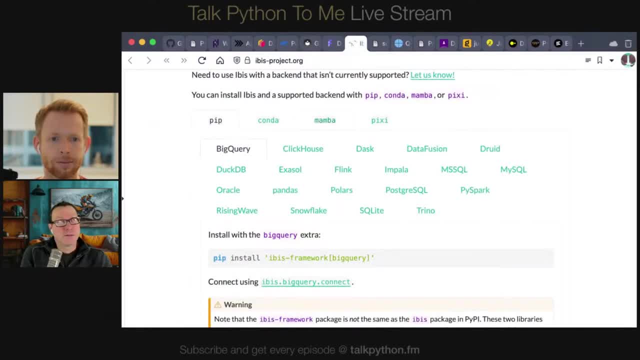 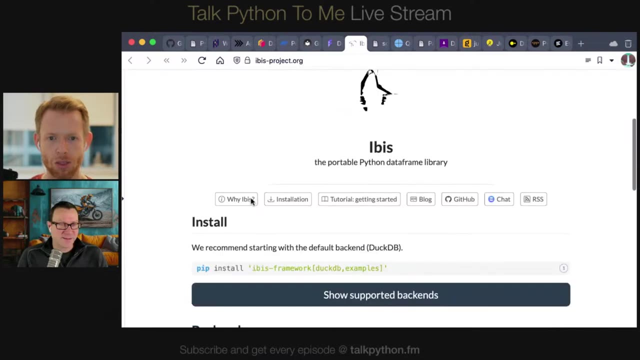 it's interesting that a lot of these data frame libraries they try to base their api to be pandas like but not identical potentially. you know thinking of dask and, yeah, others. but this ibis sort of has the ability to configure it and extend it, make it different, kind of like. 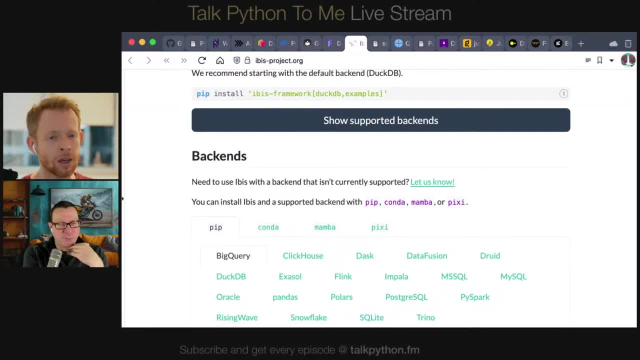 for example, dask, which is one of the back ends here. yeah, it does, but the api doesn't change right, it just it. it talks to the different back ends. yeah, there's, there's different schools of thought on this. so there's there's a another project called moden, which is similar to ibis in many. 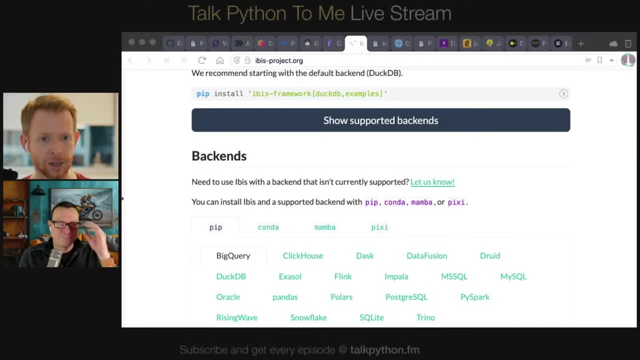 ways in the sense of like transpilation and sort of dynamically supporting different back ends. but like the way it's structured, it's sort of based on the standard understanding for our context of sim shareholders. so it's pulled into, you've got a backing track, there's a 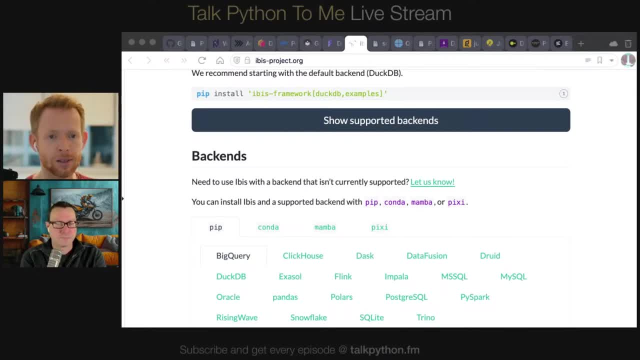 standaloneơ- tus run the paddanged code that projects like polars and ibis and das data frame that uh take like design cues from pandas in the sense of like the general way in which the, the api, works, but has made meaningful departures in the interest of um doing things better in many ways than than um than pandas did in certain parts. 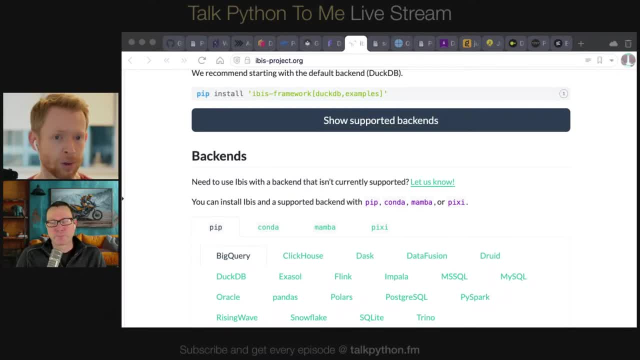 of the parts of the api, um, and making things simpler and not being beholden, like beholden to decisions that were made in pandas, you know, 15 years ago. not to say there's anything bad about the pandas api, but, like with any api, it's large, like it's it's, it's very large, as evidenced by: 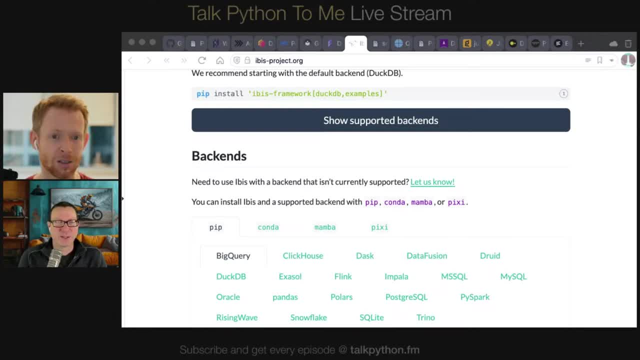 you know the 2000 page pages of documentation, and so, um i i understand the the desire to make things simpler while also refining certain things, making certain types of workloads um easier to, easier to express, and so polars, for example, is very expression based um, and so everything is. 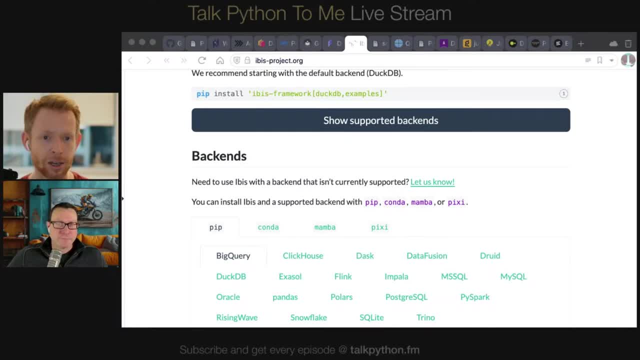 column expressions and is lazy and not eagerly computed, whereas pandas is eager execution, just like numpy is, which is how pandas, you know, became eager, eagerly executed in the first place. um, and so i think the mantra with polars was: we don't want to support the eager execution by default that pandas provides. 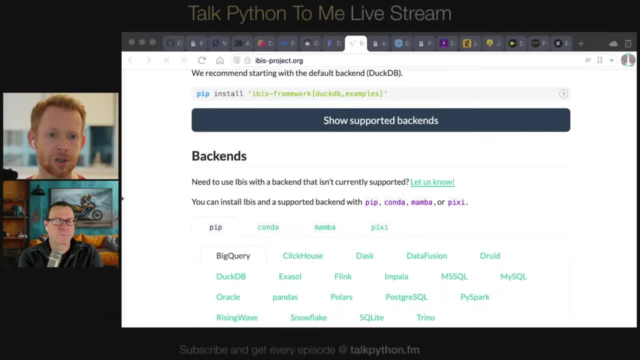 we want to be able to build expressions so that we can do query optimization and take inefficient code and, under the hood, rewrite it to, you know, be more efficient, uh, which is, you know what you can do with a query optimizer, um, and so ultimately like, and that that matters a lot when you're executing code remotely or in like a big data. 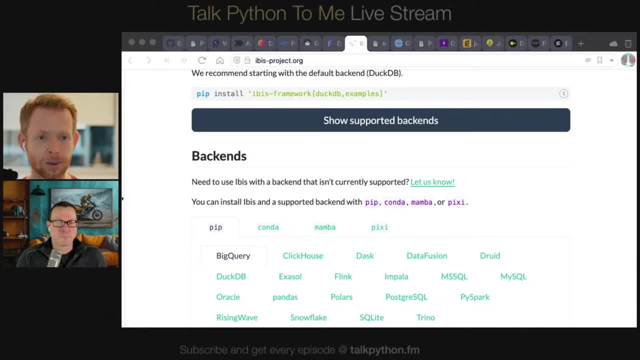 system um that you you want to have the freedom to be able to take, like a lazy, you know analytic expression and rewrite it. you know, based on it might be like you need to seriously rewrite the expression in the case of like dask, for example. like dask has to do um planning across a distributed 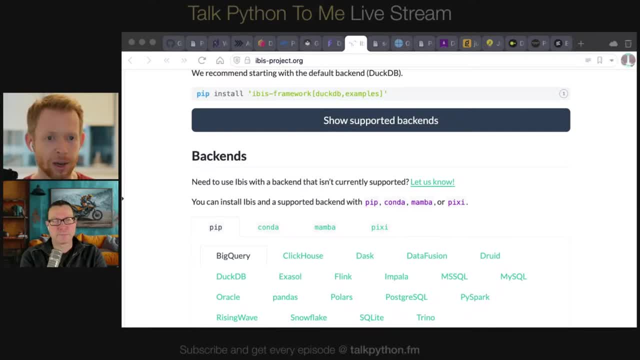 data, um, and so you know dask data frame is very pandas like, but it also includes some explicit details of being able to control how the data is partitioned and being able to have some knobs to turn in terms of, like um, having more control over what's happening on a distributed cluster. 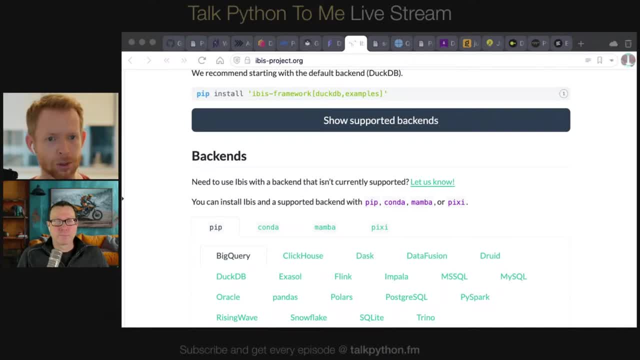 and i think the goal there is like to give the developer more control, as opposed to like trying to be intelligent. you know, make all of the decisions on behalf of the developer. um, so if you, you know, if you know about how you know, know a lot about your data system, you know how to do that. 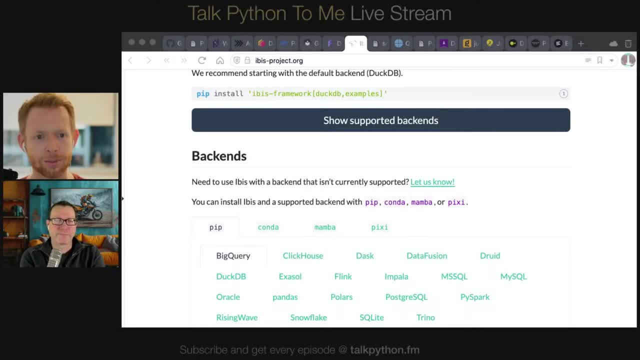 then you can make more. you can make- uh, um, you know- decisions about how to, how to schedule and execute it. of course, dask is building, you know, query optimization to to start making more of those decisions on behalf of the user. but, um, you know, dask has become very popular and impactful. 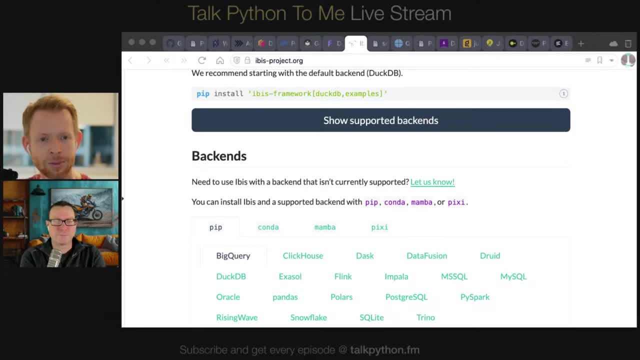 and making distributed computing easier in python. um, so they've gotten, you know, i think gotten a long way without turning into a database, and i think dask never aspired to be a, to be a database developer, so i think that's a really good example of how distributed computing is. you know not. 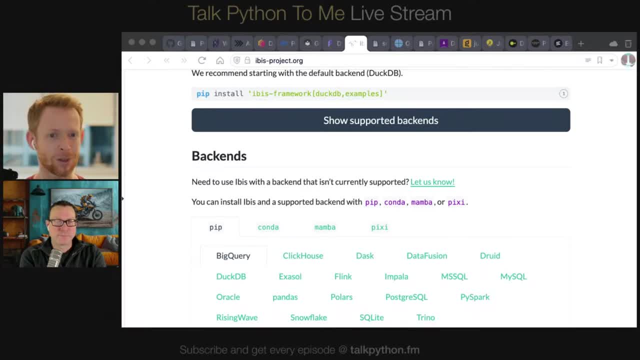 database, like it could be distributed array computing or distributed model training and just being able to easily run distributed- you know- python functions on a cluster and do distributed computing that way. it was amazing like how many people were using um pi spark in the early days just for the convenience of being able to run python functions in parallel on a cluster. yeah, and. 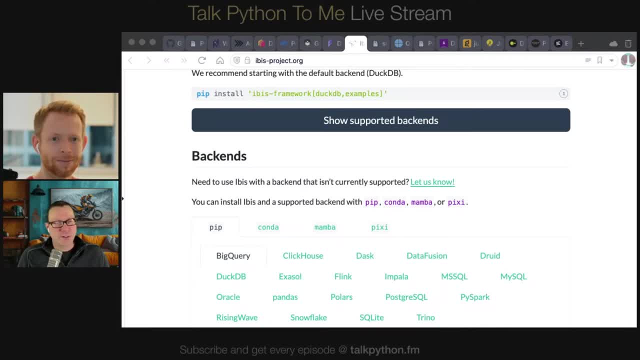 that's pretty interesting. you know, you probably come across situations where you do a sequence of operations. they're kind of commutative in the end in practice but from a computational perspective, like how do i distribute this amongst different servers maybe? uh, one order matters a lot more than the other. 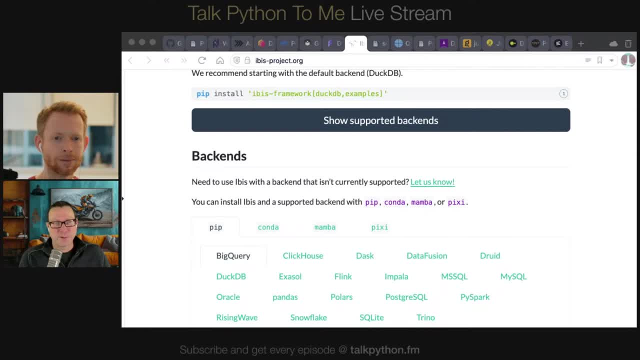 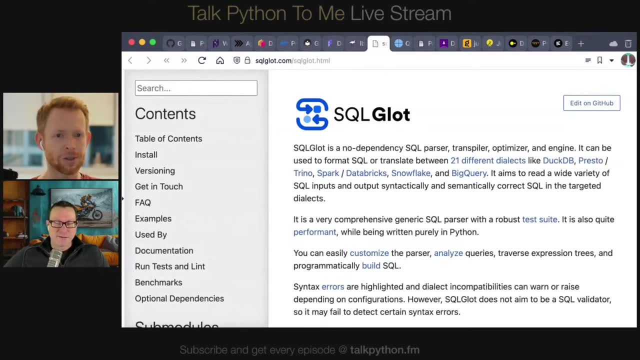 performance. you know, yeah, yeah, interesting, all right. one final thing: sql glot. yeah, so, so sql glot, uh project started by toby mao, so he's a netflix alum and uh, um, you know, really, yeah, really talented, talented developer who's created this? uh, sql query transpilation framework, uh, library for python and uh, you know. 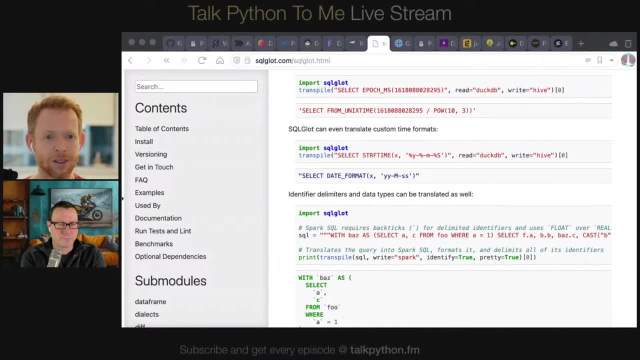 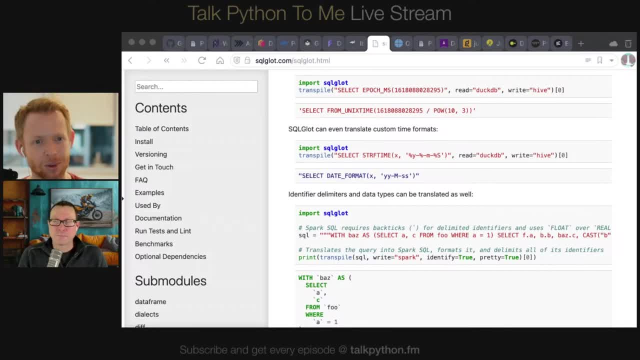 sql queries written for one engine and use them someplace else um without something like sql glot, you would have to manually rewrite and make sure you get the typecasting and coalescing rules um correct. and so sql glot has. um understands the intricacies and the quirks of every database. 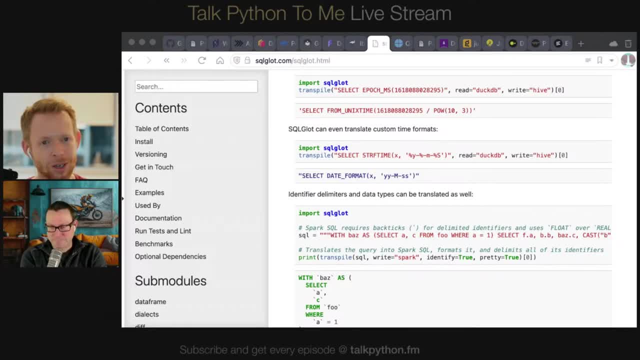 dialect, sql dialect, and knows how to uh correctly translate uh from one dialect to another. and so ibis uh now uses sql glot um as its underlying engine for um query transpilation and generating uh, generating sql uh, generating sql outputs. so originally ibis had its own um kind of bad version of sql glot uh kind of a query. 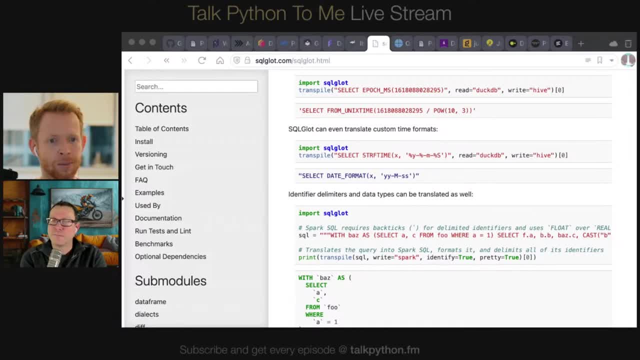 transpile like sql transpilation, um, that was uh powered by, i think powered by uh, sql alchemy and um and some and a bunch of custom code, and so i think they've been able to delete a lot in ibis by moving to sql glot and 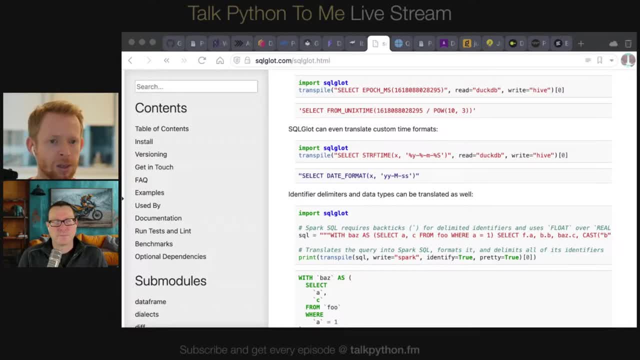 i know that you know sql lot is also, you know, being used to you know power kind of a new um, yeah, being used in people building new products that are python powered and things like that. so, and and toby, like his uh company, tobiko data, they uh, yeah, they're building a product called sql mesh. 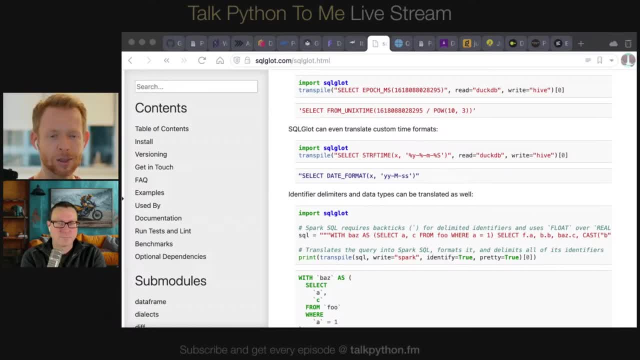 um, that's uh. that's powered by sql glot, so very cool project and maybe a bit in the weeds, but if you've ever needed to convert a sql query from one dialect to another, it's uh. yeah, sql lot is here to save the day. i would say. you know even simple things is how do you specify a parameter? 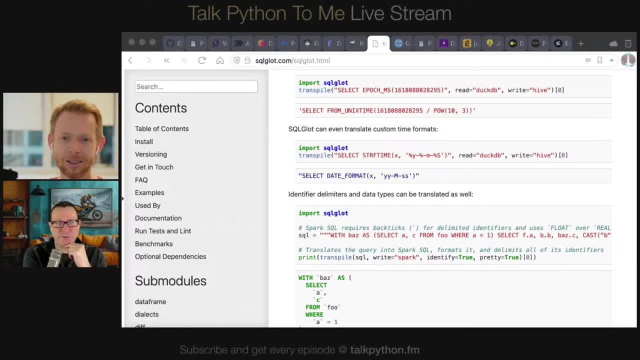 variable, you know, for a parameterized query right, and microsoft sql server it's like at the very the, the parameter name, and oracle it's like question mark or sql. i think it's also quite. you know just that. even those simple things it's a bad, and without it you end up with little bobby. 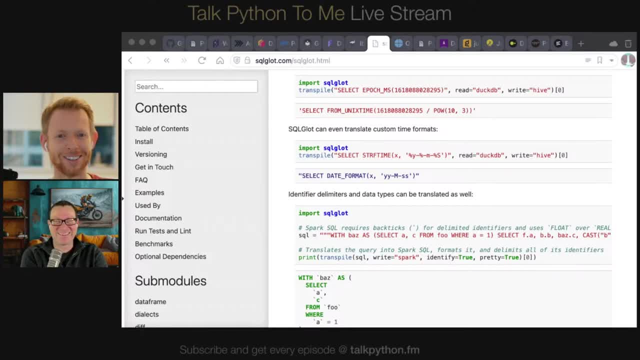 tables, which is also not good. so that's true. that's true, nobody wants to talk to him. yeah, this is really cool sql- a lot like polyglot, but all the languages of sql, nice and uh, you do things like you can say: read duck db and write the hive, or 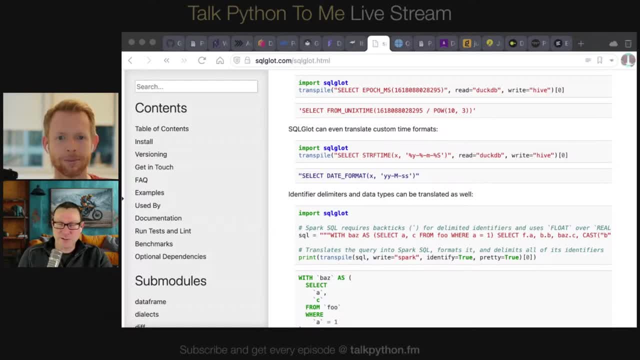 read duck db and then write to spark or or whatever. that's pretty cool. yeah, all right, west, i think we're getting short on time, but you know, i know everybody appreciated hearing from you and hearing what you're up to these days. anything you want to add? 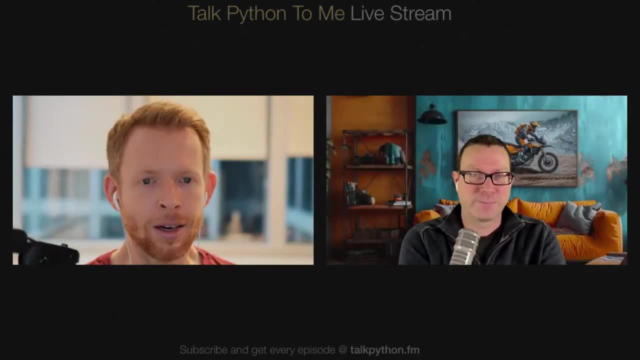 before we wrap up, i don't think so. yeah, i enjoy the conversation and um, yeah, um, yeah, there's a lot of stuff, a lot of stuff going on and uh, still plenty of things to get get excited about. so i think often people feel like. people feel like, uh, you know all, the, all the exciting problems in the 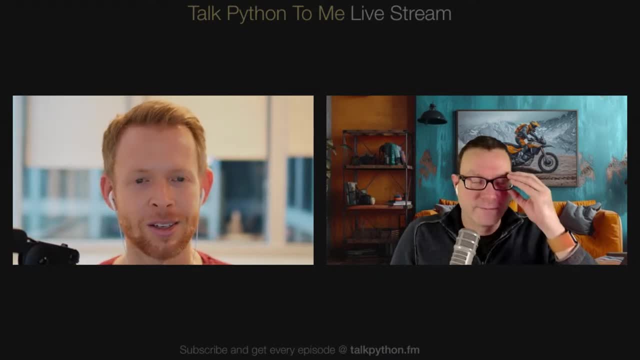 in the python ecosystem have been solved, but there's still still a lot to do. and, um, yeah, we've made a lot of progress in the last uh, uh, you know, 15 plus years, but, um, you know, in some ways feels like we're, feels like we're. 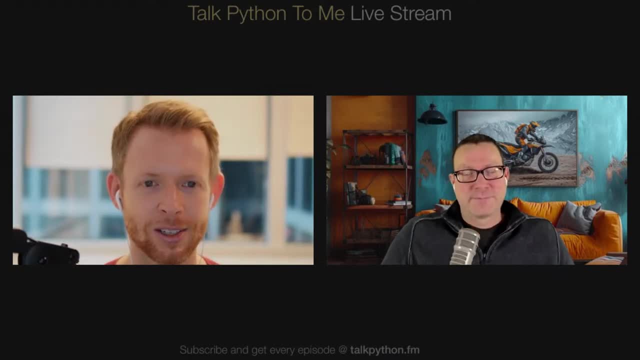 just getting started. so we are just excited, excited to see where things go next. yeah, every time i think all the problems are solved. then you discover all these new things that are so creative and you're like, oh well, that was a big problem. i didn't even know it was a problem, it's. 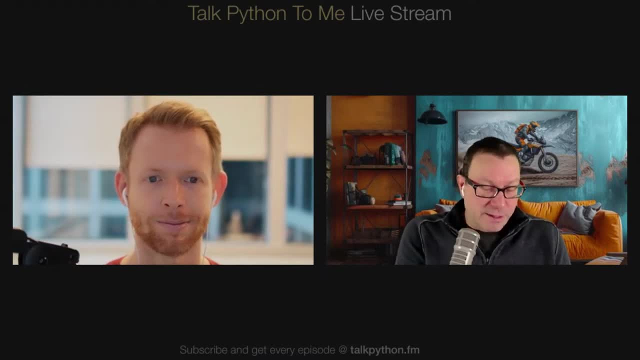 great. yeah, well, all right, thank you for being here and taking the time and, yeah, keep us updated on what you're up to. sounds good, all right.